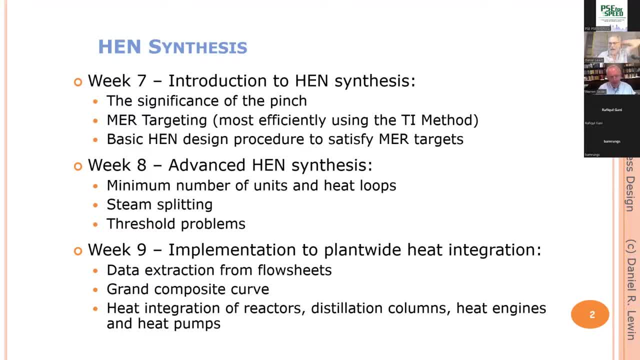 And in the last of the three weeks we bring everything to reality, That is, we connect to the real process. that involves teaching the students how to do data extraction from real flow sheets. It's all about mastering the usage of the grand composite code, which enables a marshaling, alternative utility sources to minimize costs. and, finally, rules about heat integration of reactors, distillation columns, heat engines and heat pumps. 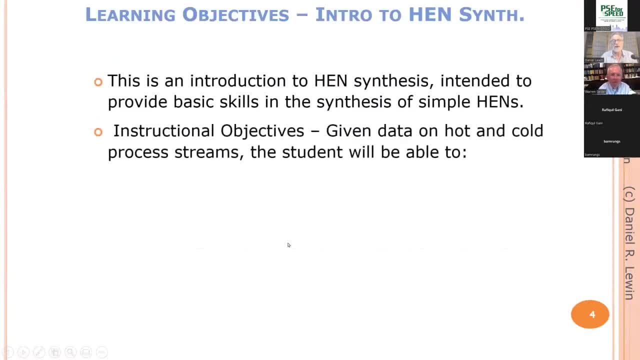 Let's go into some more detail. So here is the first part, introduction. Here are the instructional objectives. As I said before, you are given data for hot and cold process streams. You should be able to compute the pin range, temperatures, compute the MER targets and design the HEN to meet the targets. Very, very. 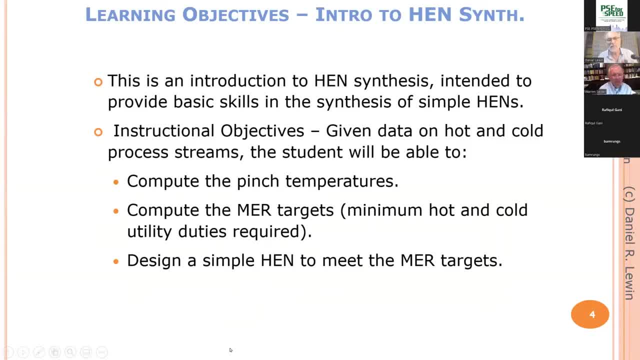 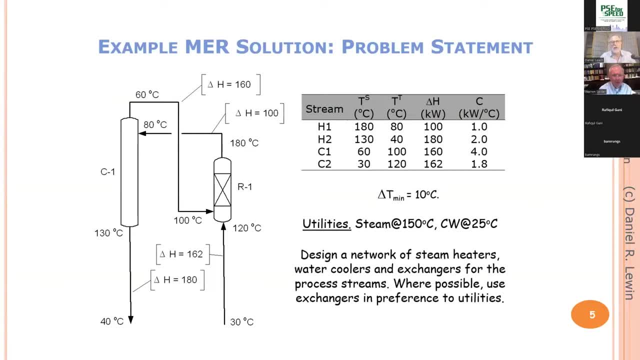 straightforward, simple: first week We walk before we run. Typically they'll get a problem to look at. This is a very simple example problem involving two units: one reactor, one column. one separating column involves four possible streams for heat integration: too hot, too cold. 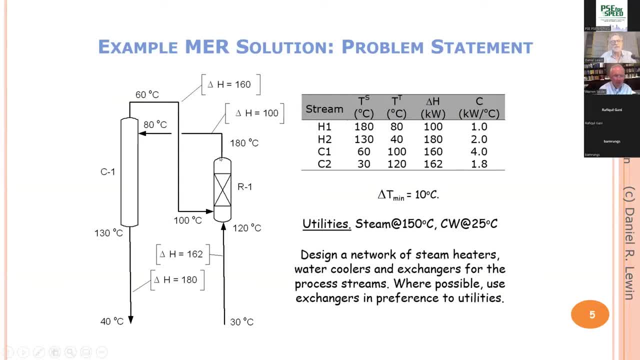 So for each stream you would have its source temperature. For example, for hot stream, one source temperature is 180 degrees, target temperature 80 degrees. The enthalpy change is 100 kilowatt, which means the flowing heat capacity is one kilowatt per degree centigrade. 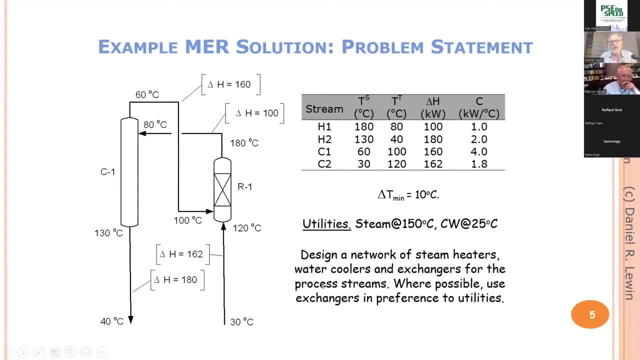 The same method is used to extract data from the others. Of course, in reality, we would need to be doing this from real process streams, but that comes later. So the objective is to design an efficient network of heat generators, and we're going to do that. So we're going to do that. 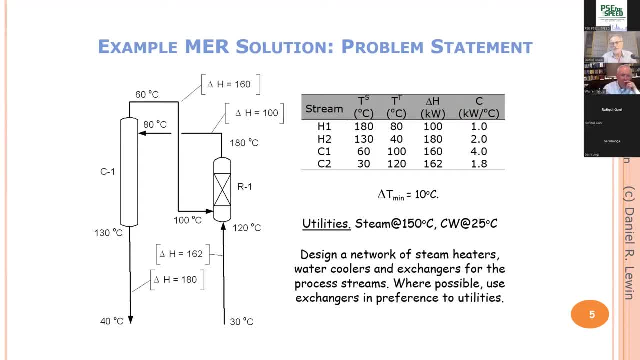 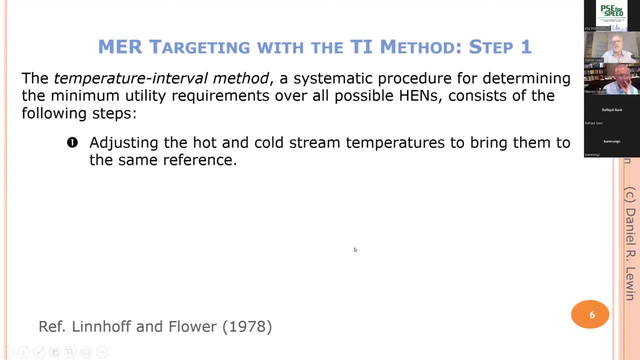 The temperature interroute method, which is what we teach, involves three steps. First, we adjust the hot and cold stream temperatures to bring them to the same reference. Typically what that means is we remove delta T min from all the hot stream temperatures. That means now we're only 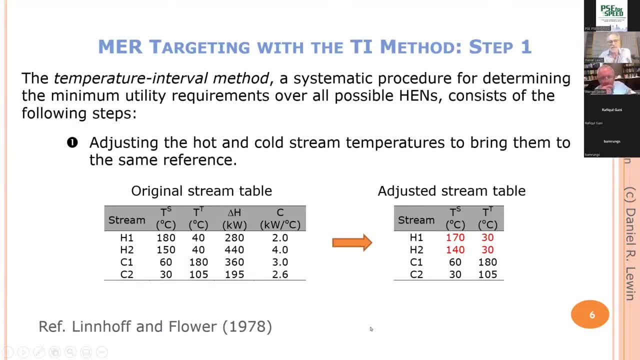 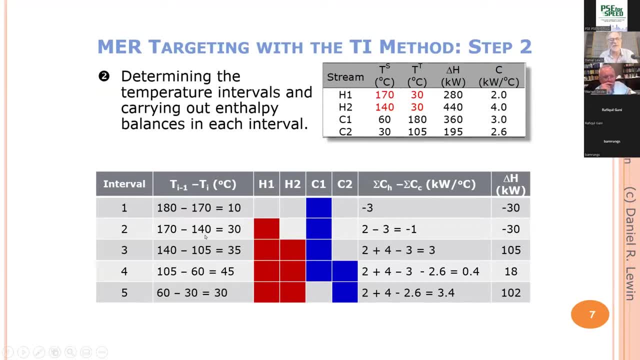 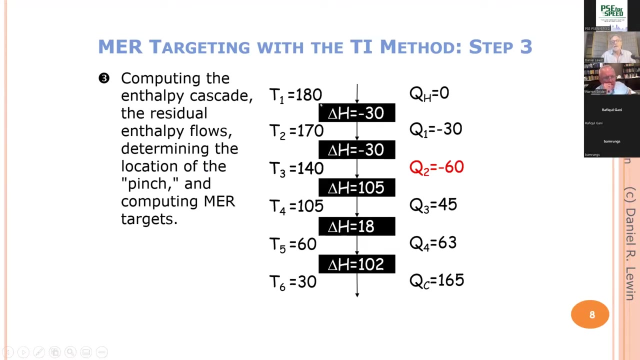 talking about one temperature scale, the cold stream scale. We then determine temperature intervals by just stacking the determined temperature intervals that have been extracted in a descending order. defining for each temperature interval The enthalpy balance gives us the possibility to do calculation of the enthalpy cascade. Basically, we stacked. 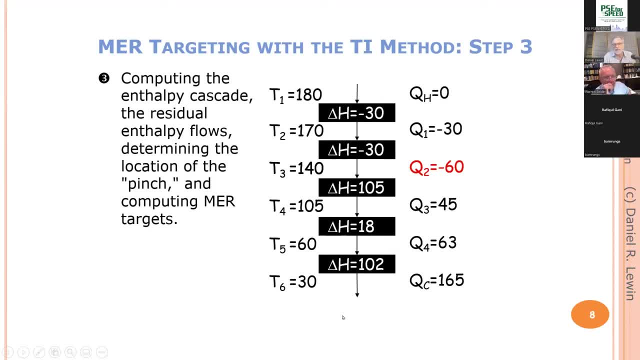 the intervals. Between each interval we have the enthalpy change that we just computed. We assume no external heat hot stream required and then just cascade down, estimate or compute the minimum residual enthalpy And of course this minimum residual enthalpy has to be zero. 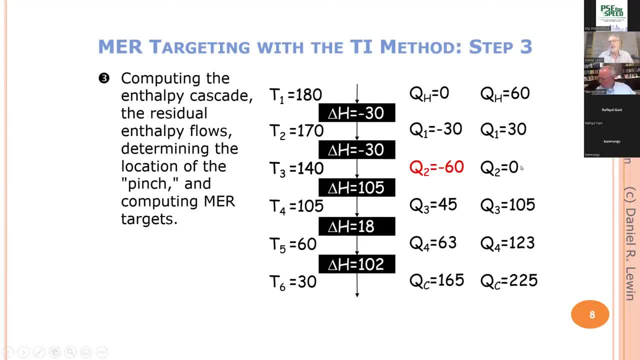 or greater When it is equal to zero. we now have the MER targets. So here we have six, 60 kilowatts of heating, 225 kilowatts of cooling as our target, and we've identified the pinch temperature of 140 degrees centigrade cold and, of course, 150 degrees centigrade hot. Very good. 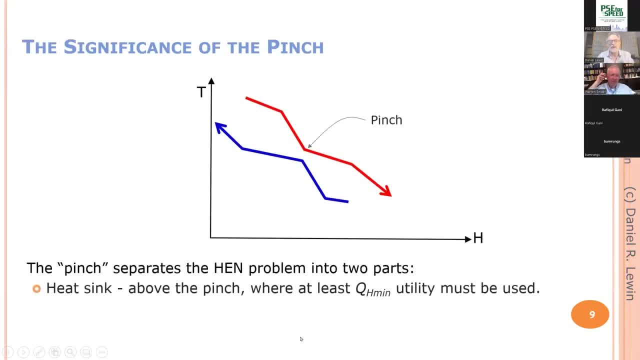 Why is the pinch significant? Because it defines the problem into two portions: a heat sink above the pinch and a heat source below the pinch. Above the pinch, we are only allowed to use external heating, and the targeting allows us to use external heating, So we have a temperature. 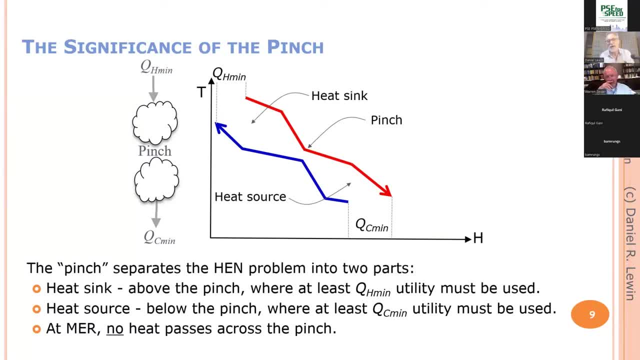 interval that allows us to estimate the actual value, which is now calculated as qh min. Below the pinch there's a heat source. Therefore, we can only use cooling, and the minimum cooling requirement has just been determined by the temperature interval method. 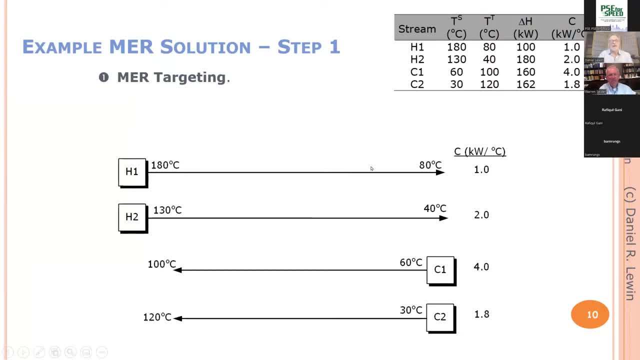 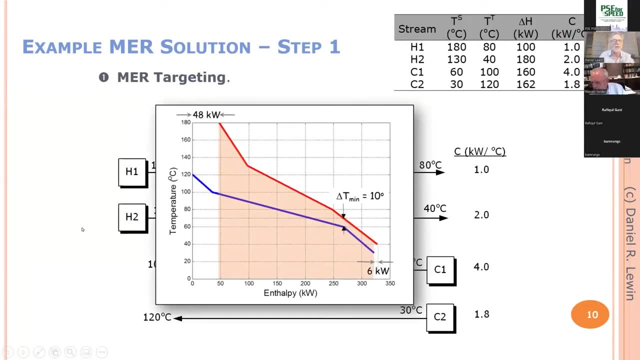 We then have to design a heat exchanger network that meets the targets, for, of course, the first step being targeting, which we just did. So, for example, for the problem that we started the section with, there's the reactor and the heat and the distillation column. 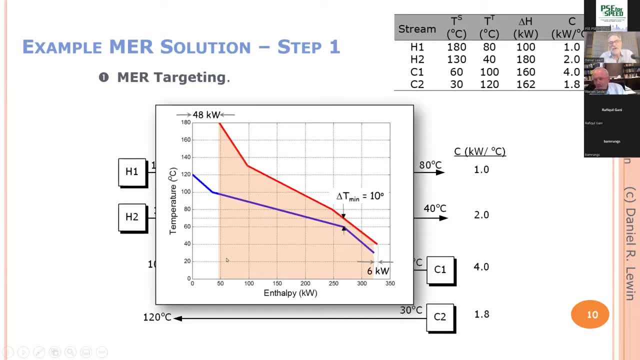 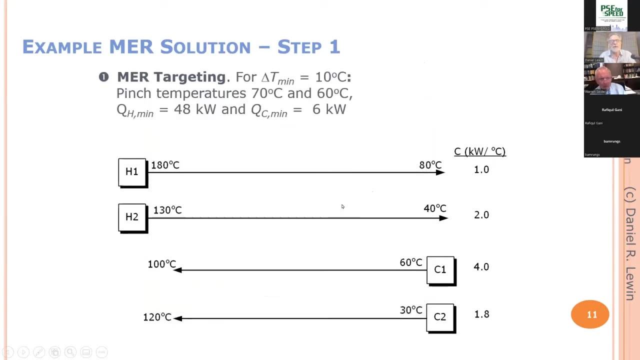 The minimum heat requirement is 48 kilowatt Minimum cooling from the six kilowatt For delta T min of 10 degrees. the pinch temperatures are 70 hot, 60 cold. So the first thing we do is we take our streams, all four streams, separate the system at the pinch and then 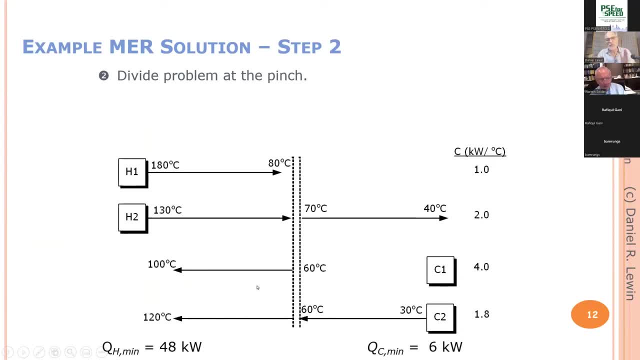 design, first above and then below the pinch, Two separate design problems. And what is the really key? the students have to get this point across: that the design is always from the pinch moving outwards. The reason we do that is at the pinch the system is most constrained. 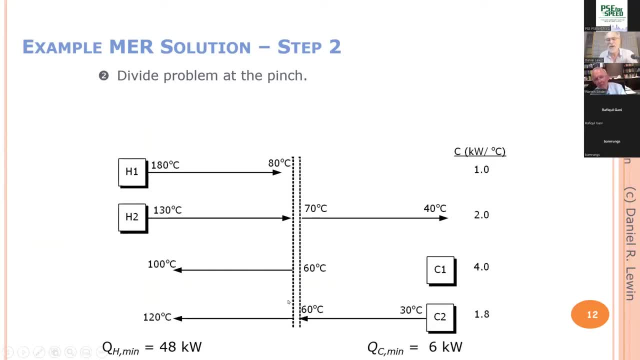 At that point all the hot streams and cold streams at the pinch are exactly delta T min apart, and we have to make sure that we do not violate this limit. So there are rules Immediately above the pinch. we pair such that the hot flowing stream capacity has to. 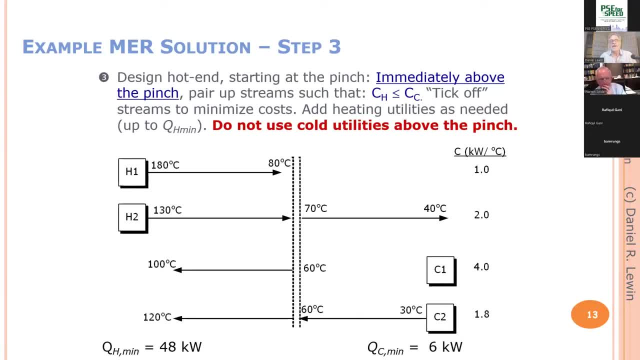 be less than or equal to the cold stream capacity And take off. The other important thing to notice is, since we start by designing above the pinch, above the pinch, there is only hot utility allowed. Therefore, all the cold, all the hot streams have to be cooled by cold streams. Therefore, the key is to eliminate. 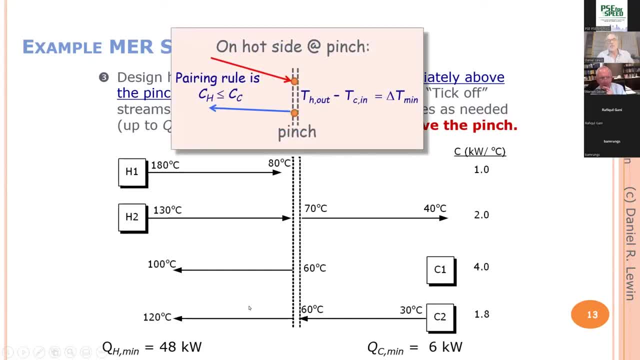 the hot streams first. So, using this rule, we have to pick a cold stream to match the only hot stream at the pinch. In this case it will be H2. And we have to make sure that the cold stream flowing Heat capacity is greater than the hot stream, Since the hot stream flowing heat capacity 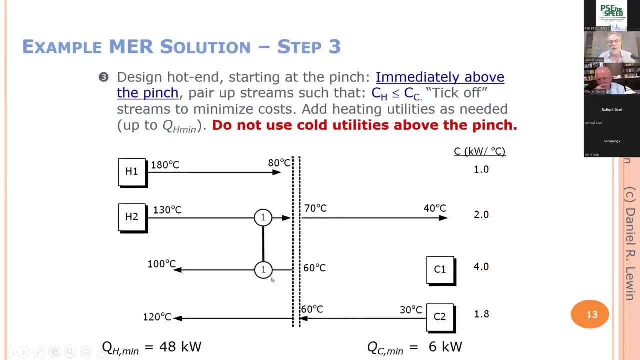 here is two kilowatts per degree centigrade. obviously we have to match it with C1. And we load this heat exchanger in such a way that we tick off one of the two streams. In this case we have now eliminated H2 above the pinch That cooling requirement has been. 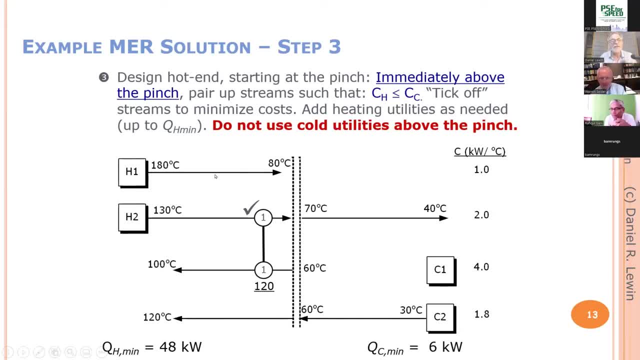 totally satisfied by C1.. We then have to decide what we do with H2. And obviously we're going to match this with the other cold stream that is still available and load it in such a way that we tick off one of the two, whichever. 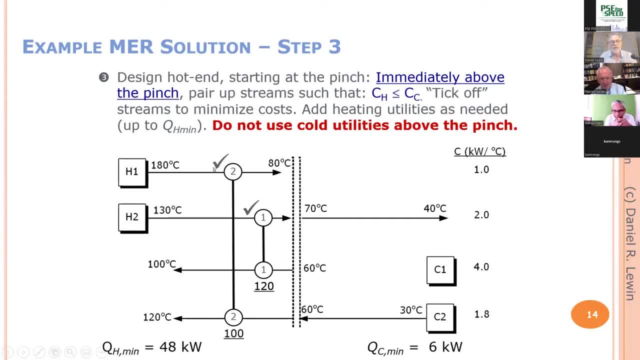 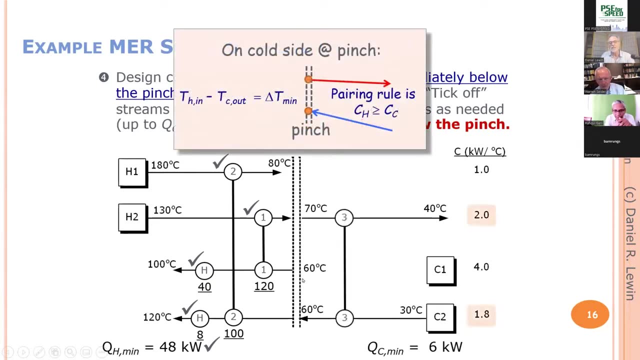 has the lowest heating or cooling requirement, We tick off H1.. We've now eliminated both the hot streams, which means we now just basically add trim heaters to complete the design above the pinch and simultaneously also match the hot target. The same rule in reverse is applied. 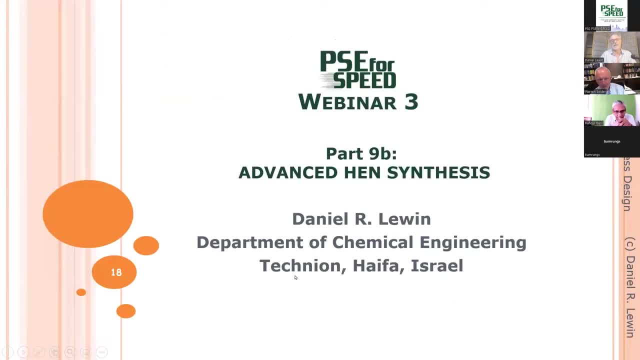 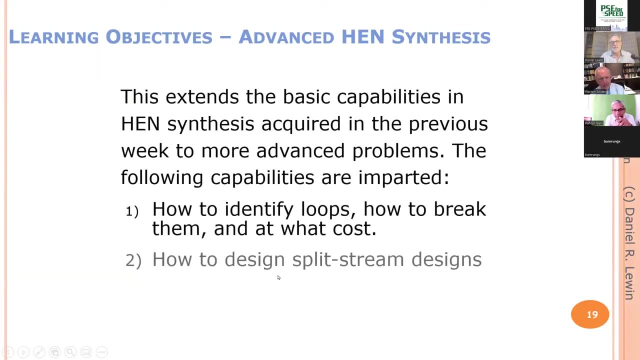 below the pinch, And that's basically what the students have done in the first week. That's their level. We then move in the second Week to advanced whoops, to to advance hand synthesis, basically how to identify loops, how to break them and at what cost, how to design split stream designs and how to design. 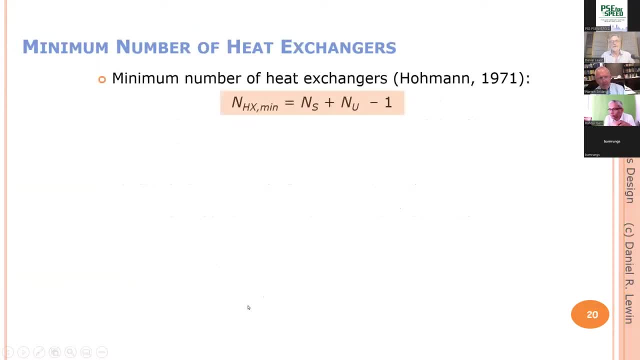 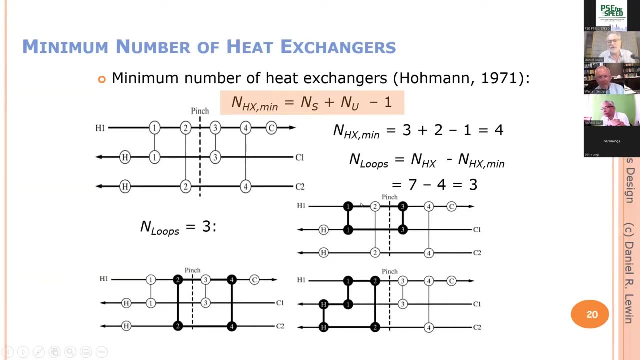 threshold systems. That's what we're doing in the second week, So I'm not going to go into a lot of detail here. Basically, there is a way of estimating the minimum number of heat exchanges and thus determine how many loops there are in the system in stream split. 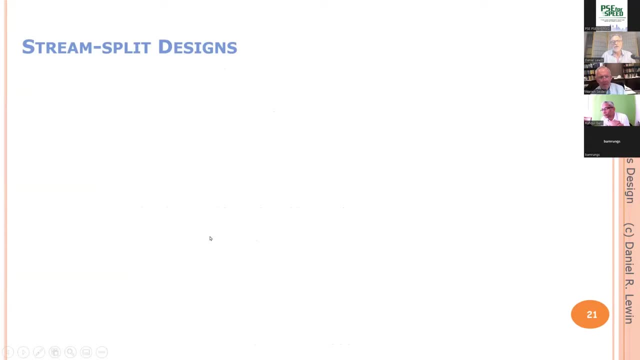 designs. The idea is to, for example, in this case, where we have an example situation with one hot stream, two cold streams, the one possible solution would be: well, after we've done the calculations for targets, we see that our targets require no external heating, no external cooling, and the unit target gives: 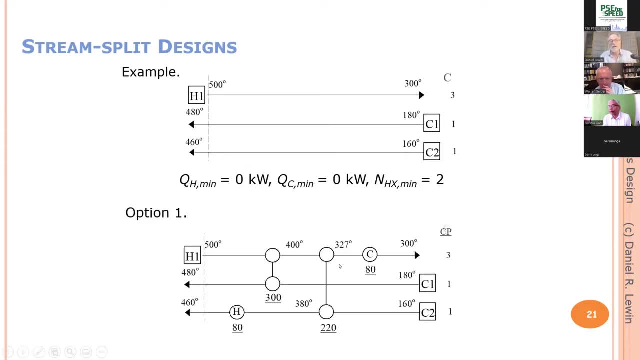 us a value of two units that we should be able to satisfy. A student who was totally asleep in the first week of the course might design something like this, which involves four units to above the minimum and also requires Heating and cooling utilities which are above the minimum values of zero. Anybody who does 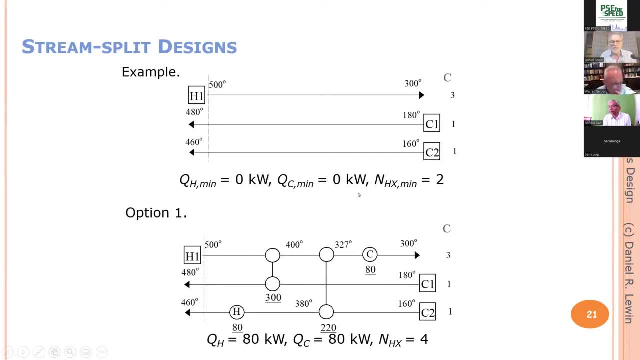 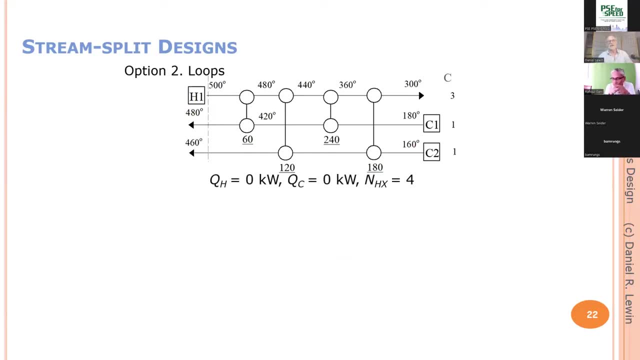 this was not around in the first week of the course, So hopefully no one will design this by the second week of the material. but somebody who doesn't know about stream splitting would do this design which, on the one hand, manages to satisfy the MIR targets, but unfortunately, 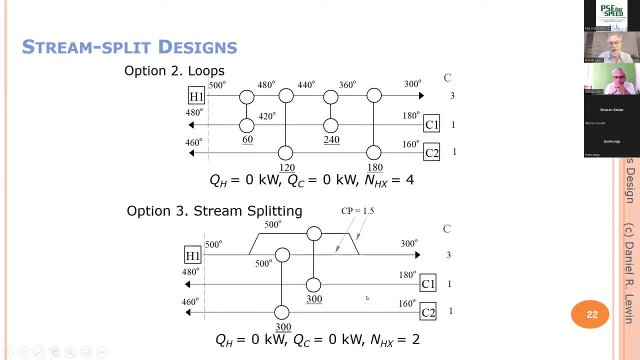 has two more heat exchanges than are required. Learning about stream splitting will allow us to do this for a design that is to split the hot stream And maximize the driving force available between two- the two cold streams that need that need heating- And this actually is- is the stream split design. There are rules associated. 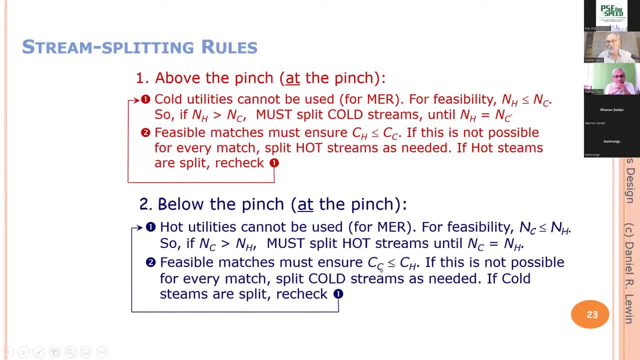 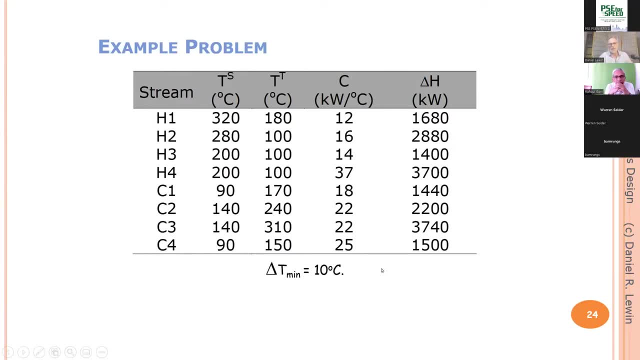 with the stream split design, the details of which I will not trouble you with in the in the interest of time. But what do we do with this? We now are able to deal with more complicated problems, The kind of problem that a student would be solving by the second. 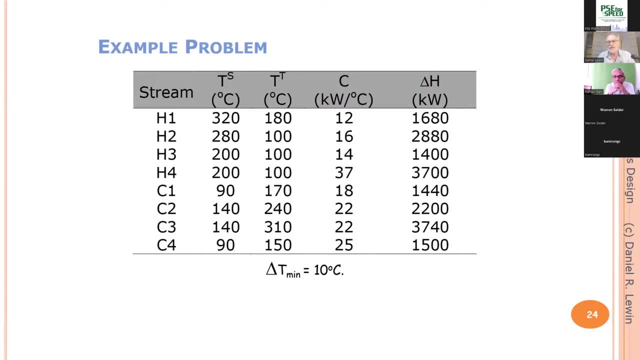 week of this material would be this monster here which, after the initial heart attack, the students Will experience, will they will soon realize that if they apply what they've learned, it's not as tough as it looks. All right, We start by targeting right. That's what we said. 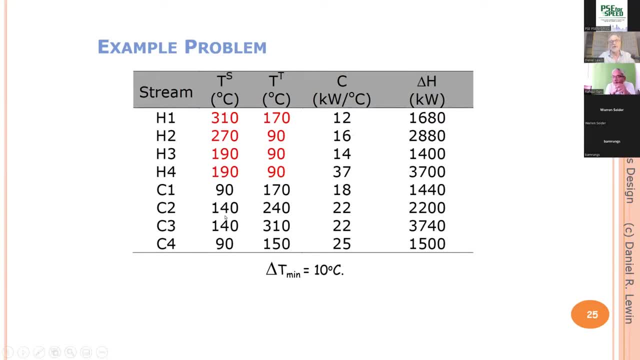 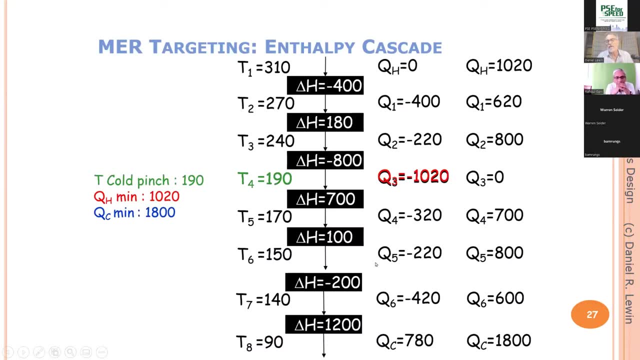 So targeting means remove Delta team in from all the hot streams. do interval balances, do the energy cascade, compute the targets? So here are our targets: We have 1,020 kilowatts of heating, external heating, 1,800 kilowatts of external cooling, And the pinch is at 190. 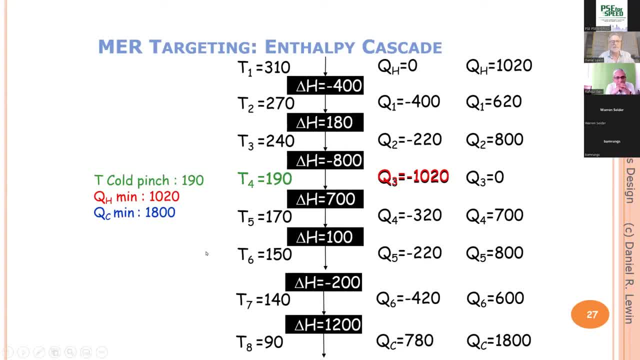 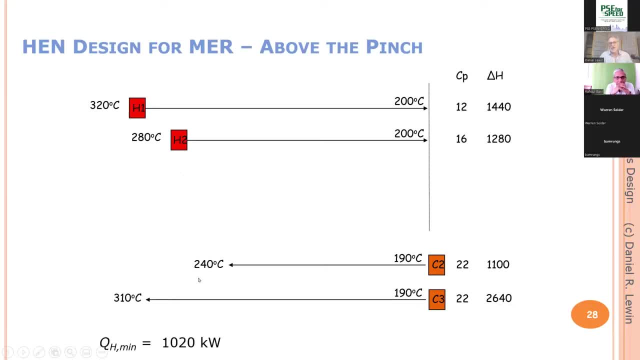 degrees centigrade cold. obviously for Delta team in of 10 would be a 200 degrees centigrade hot. So now we're gonna do the design first. above the pinch. The only streams that are actually active above the pinch, as you see here, are H 1, H 2, C 2 and C 3.. And actually this is 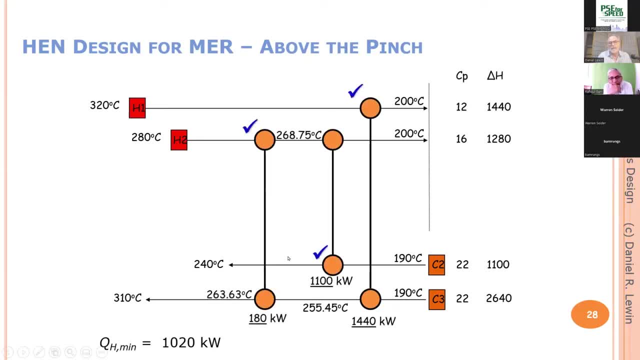 very, very easily solved. This is actually the easy part of the problem And here we have a solution. Manages to satisfy the minimum Number of units. we managed to satisfy also the energy target of 1,020.. However, below the pinch the situation is. 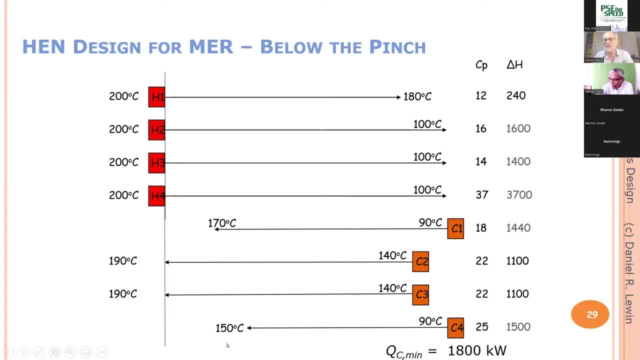 somewhat more complicated. Again, in the interest of time, I will zip through this solution. But trust me, this is what we do in class with the students And they helped me solve this problem. The trick here is to realize that we have actually we have four hot streams and two cold. 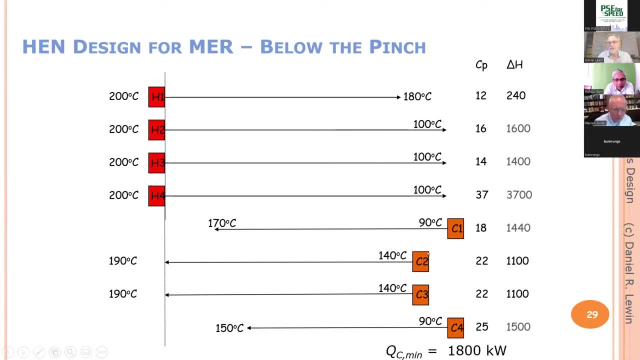 streams at the pinch right. So we have to deal with C2, C3 first of all. One possibility is this: Here we've killed C2.. We've satisfied C2, which is wonderful. Now we have C3 with a flowing heat. 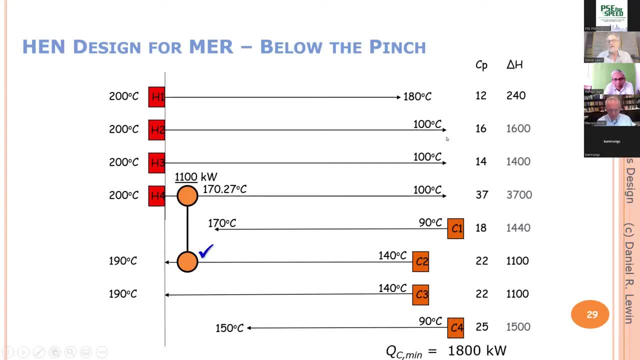 capacity of 22,, which we cannot match directly with any of the hot streams because below the pinch, we need to ensure that the flowing heat capacity of the hot stream, matched at the pinch, has to be greater than that of the cold stream, Which means that we have to split C3.. One possibility is to do an even split, like I've. 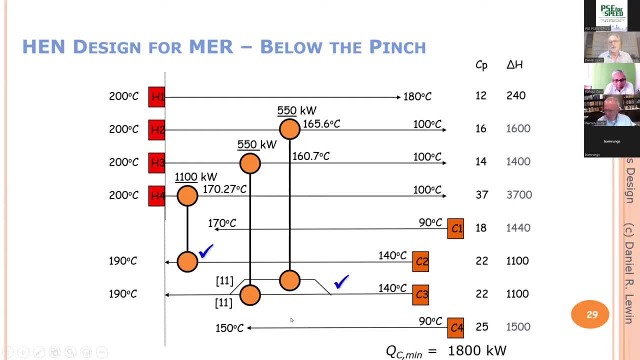 shown it here, which we've done and eliminated C3. Wonderful, We proceed with the design. Now we've taken care of C4.. We're getting very excited and very happy. Now we have C1, which we can partially deal with this way. Unfortunately, now we have a problem because 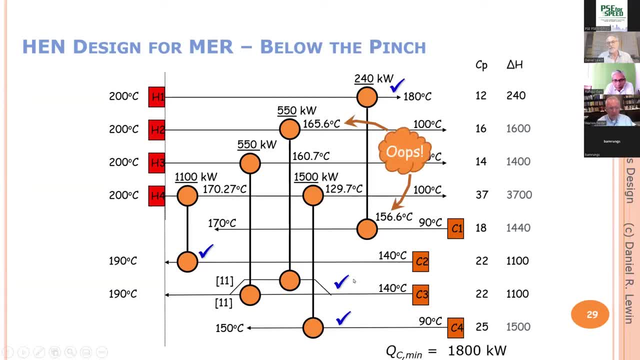 now we've generated a situation where the feed stream feeding this heat exchanger at 156 is trying to cool a hot stream which leaves the heat exchanger at 550 kilowatts, at 165.6.. And you see, here the difference between these two temperatures is less than 10 degrees. What that? 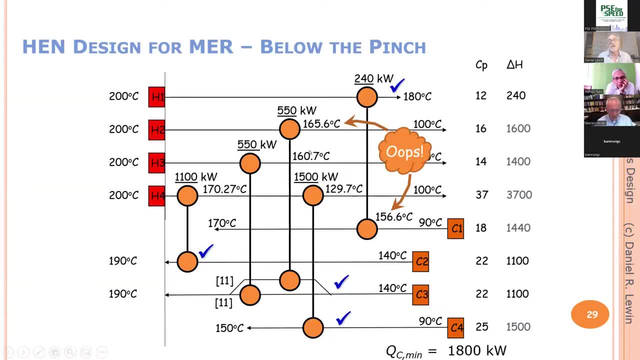 means is that this temperature around 65.6 is too low. It has to be higher In order for it to be higher. the heat duty of this heat exchanger, here this one, I'm indicating you guys see my mouse- Yes, 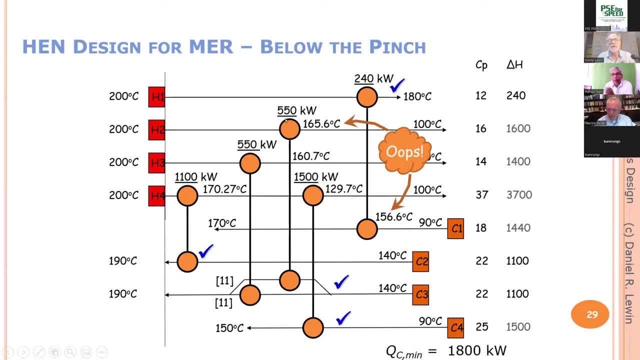 Do you see my mouse? Somebody said yes, Wonderful. So this duty has to be lower, which means I have to do a different split here, which means we have to backtrack and do the split some other way, right? The idea being that we distribute the heat transfer such 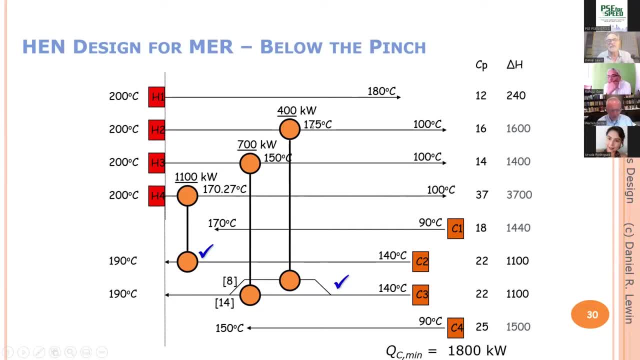 that the temperature of leaving this heat exchanger in H2 is higher, which we did. We can proceed with exactly the same steps that we did before, And now we have a situation where the temperature of leaving this heat exchanger at 156.6 meets 175.. Sally meets Harry with more than. 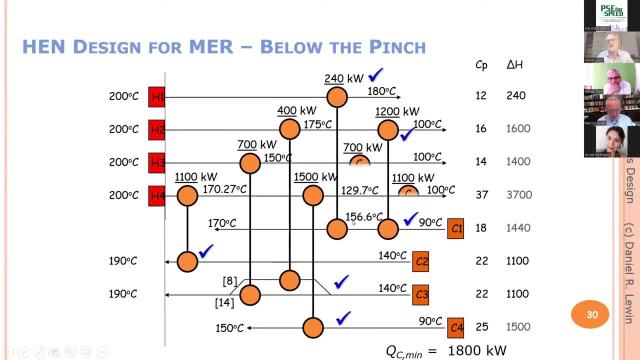 10 degrees. Wonderful, We can now position our last heat exchanger and then trim. Why is it important that students go through this design in a systematic way in class time with the lecturer? Because this kind of problem is going to come up in their designs. It's going to come. 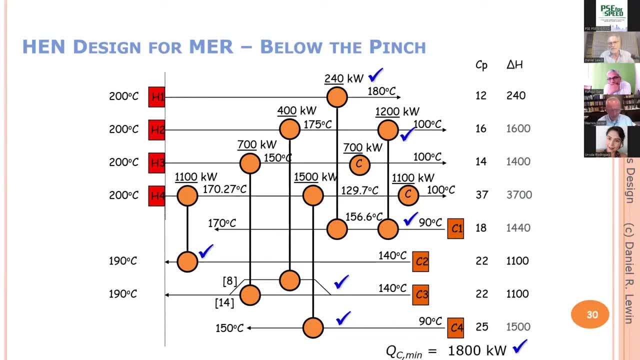 up in their exams And they have to know how to get out of trouble. This has to be done in class, with the students. This is one example why I flip, Because if I was to spend all my time in class transmitting information and not working with the students, I don't get to do this with them. 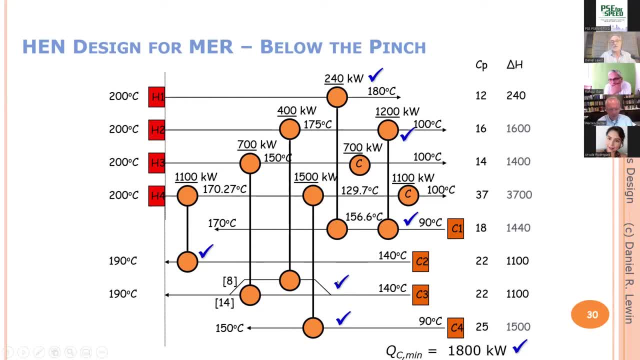 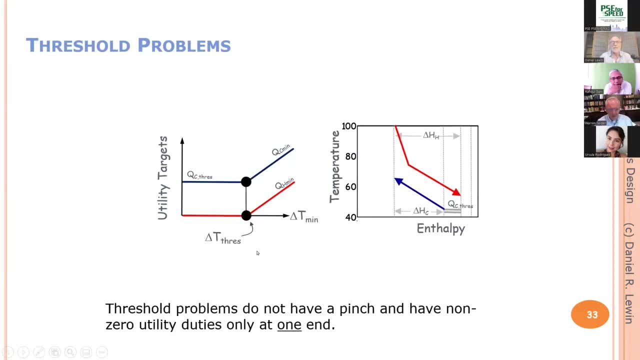 And that's their loss And it makes them less efficient engineers and designers. The last thing that we do in the second week is to deal with threshold problems, basically problems where there is only heating or only cooling, not both. I'm not going to go. 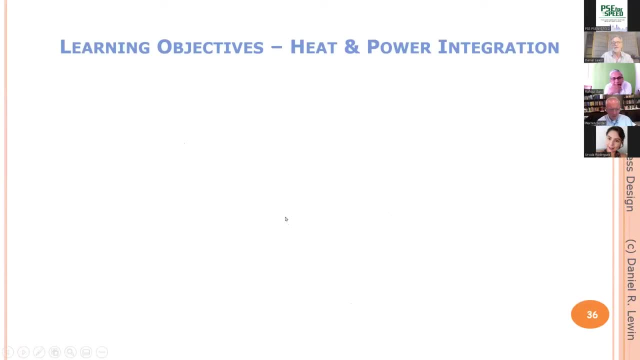 into more detail about that. But I'm going to go into more detail about that And I'm going to go into more detail about that. The last week is on, basically, heat and power integration per se. Basically, we teach the students to extract process data from a flow sheet simulator for. 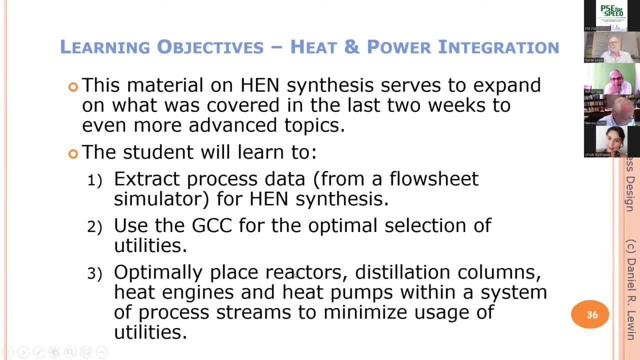 hand synthesis, how to use the grand composite curve for optimal selection of utilities and how to optimally place reactors, distillation columns, heat engines and heat pumps within a system of process streams to minimize the usage of utilities. So basically, the idea of safe 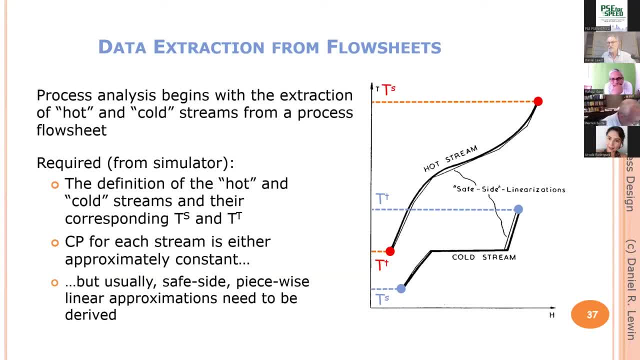 side approximation is you take the real process streams with. let's face it, they are not constant values of flowing heat capacity. We approximate them by piecewise, linear segments. Safe side means that all the hot streams are approximated on a temperature enthalpy diagram. 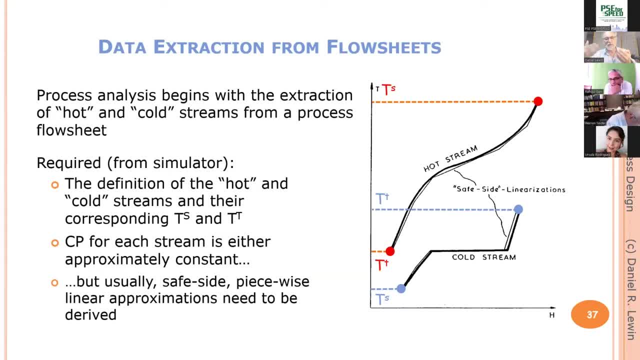 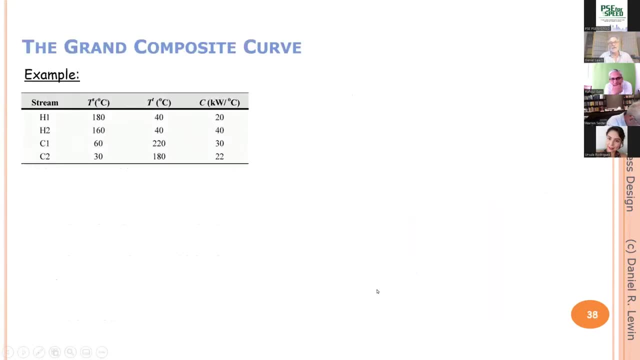 from below and all the cold streams are approximated from above. That means that we are underestimating the available driving force, which is fine for safe side approximation. So we teach the students how to do this from real flow sheet data. Grand composite curve. 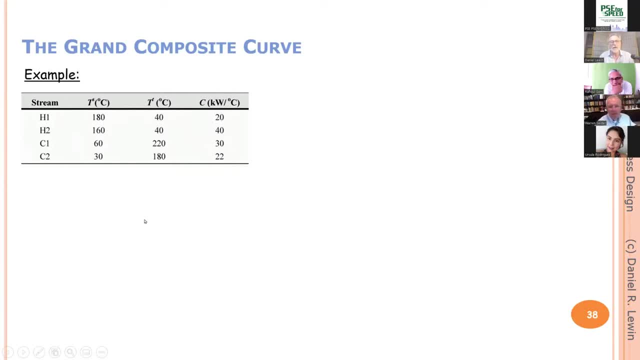 the idea is nothing really specially new. Basically we actually had the data for grand composite curves once we do targeting. Basically, all we're doing here is plotting the residuals on the x-axis against temperature intervals on the y-axis. That information we already had. So for 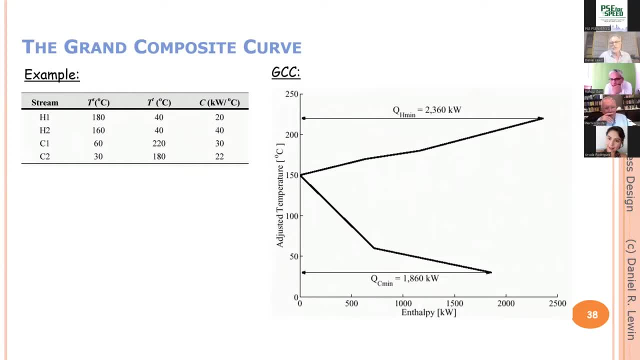 example, for this very simple system involving two hot and two cold streams, we have a hot target of 2,360 and a cold target of 1,860 with a piecewise linear segment. So we have a very simple system where we have a three-inch temperature at 150 degrees centigrade on the cold side. Now we could 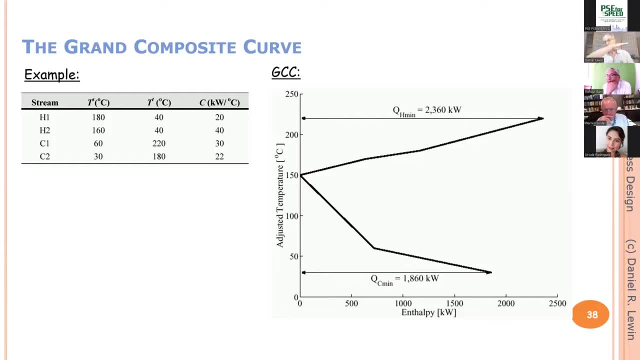 implement this design with just one heat utility- anything above 220 degrees centigrade and one cold utility anything under about 30 degrees centigrade, Or we could instead use multiple utilities and thus save money, because intermediate pressure steam is cheaper than high pressure steam. 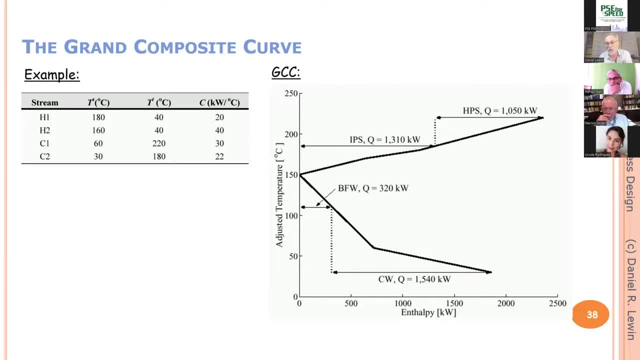 and definitely boiler feed water is cheaper than cooling water because boiler feed water generates energy as opposed to cooling water that just removes it. So we could use this to marshal our energy targets by utility type. Advantage- obviously: saving money. Disadvantage to actually 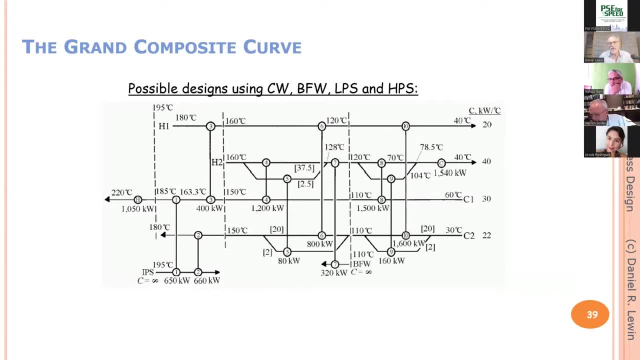 implement a design for the grand composite curve I showed before. we now have to deal with three pinches, not one. There's the process pinch, which is this one here, But we also have a pinch because of the intermediate pressure steam, and another pinch because of the boiler feed water. In fact, these pinches are this: 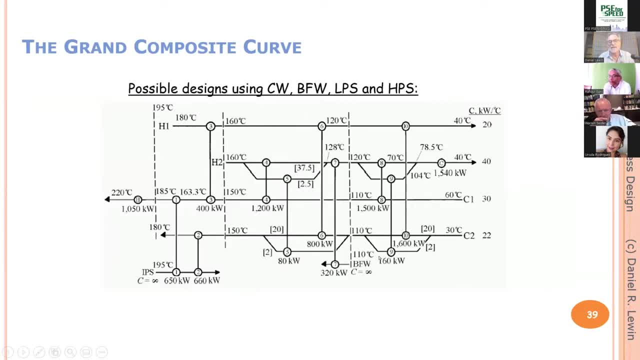 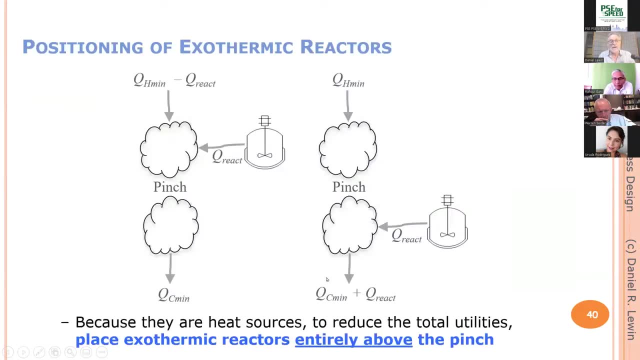 one, this one and this one. It makes the design more complicated, but it is worth considering because we significantly reduce the cost of energy. Regarding the positioning of reactors, heat reactors, distillation columns, heat pumps and so on, there's a lot of work to be done, And 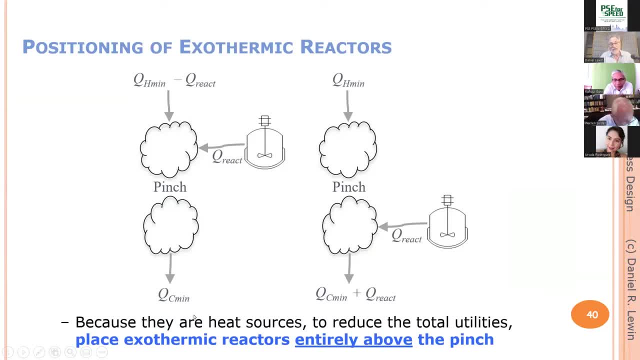 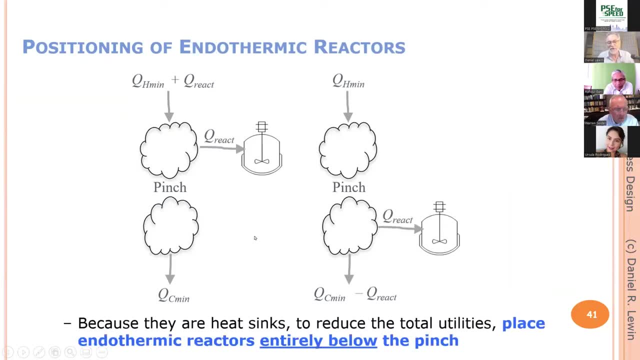 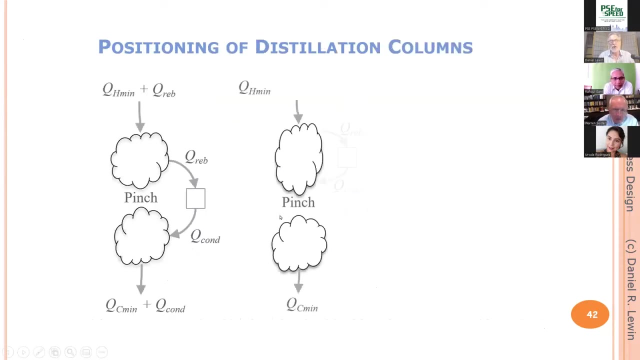 heat engines. very, very briefly. exothermic reactors are, of course, heat sources. Therefore they should be placed entirely above the pinch. Endothermic reactors are heat sinks. Therefore they should be placed below the pinch. Distillation columns have to be positioned. 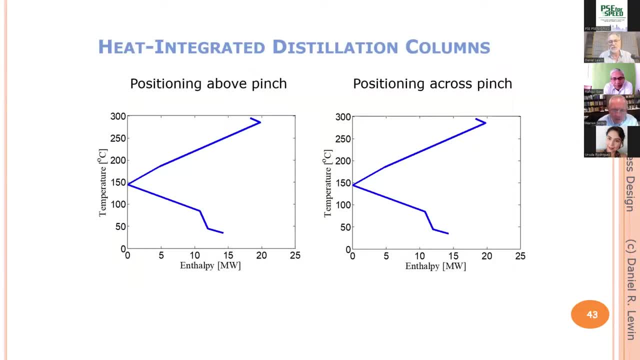 either above or either below the pinch, not across the pinch. Very easily explained using the grand composite curve here as an example of a well-placed distillation Distillation column: entirely above the pinch is the pinch, But if we decide to place it across the pinch, 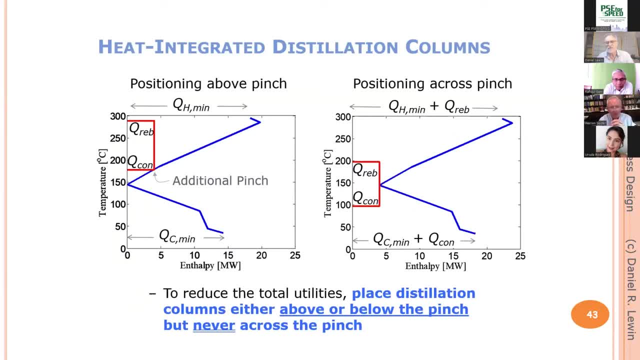 basically, what we're doing is we're not heat integrating the distillation column. Its reboiler and condenser duties are added on to the targets we had before. So that's a clear reason for opting for this solution and not this one. And what's nice about the grand composite? 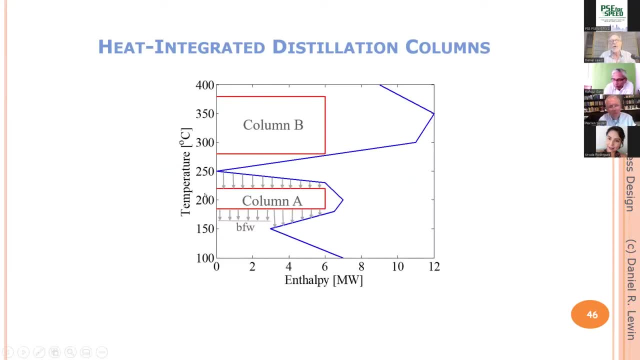 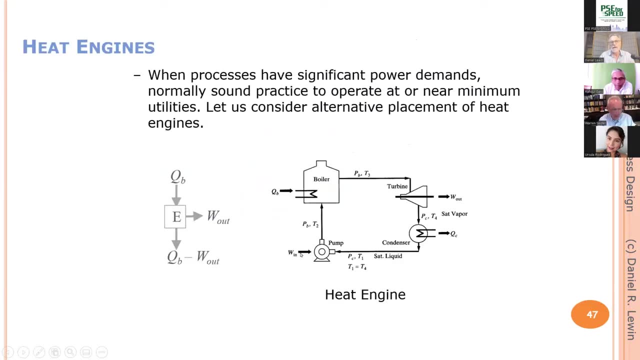 curve is: it allows one to integrate rather complex distillation column systems within an existing process, very nicely. Heat engines: heat engines have either got to be positioned above or below and not across, And heat pumps have to be placed across the pinch, of course. 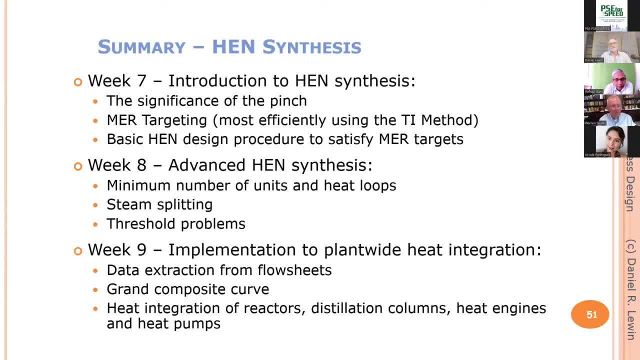 And a quick summary of what's covered in those three weeks. again, first week: very simple introduction to hand synthesis. keeping it really simple: for the first week, we start the students walking, not running. They have to understand what the pinch actually means. 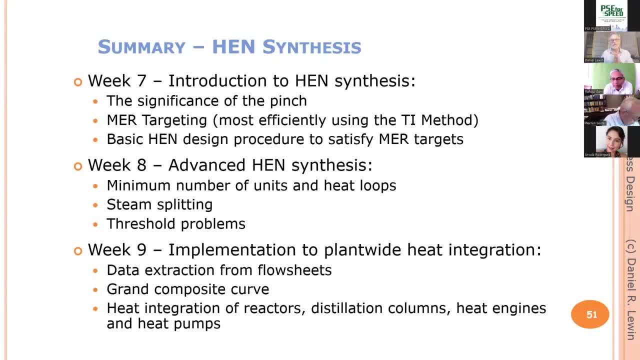 and how to use the concept of the pinch for very simple designs. how to target and how to do simple, basic pen design, nothing fancy. second week, more advanced topics: the idea of heat loops, the idea of minimum number of units, the concept of stream splitting, how that improves the capability of 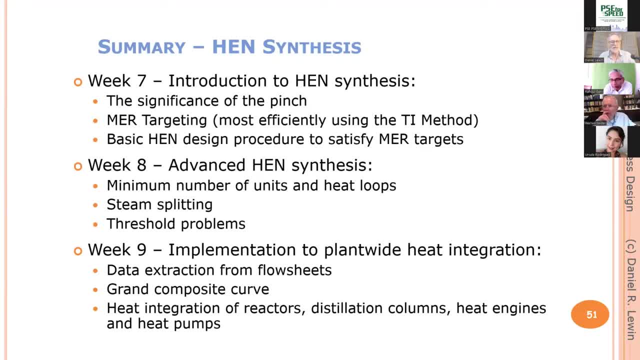 designing from there and the idea of how to deal with threshold problems, which are basically pinch problems, with only one half of the problem in actually designed for in the last of the three weeks. how to make real these tools that we've acquired. how to extract data from flow sheets. 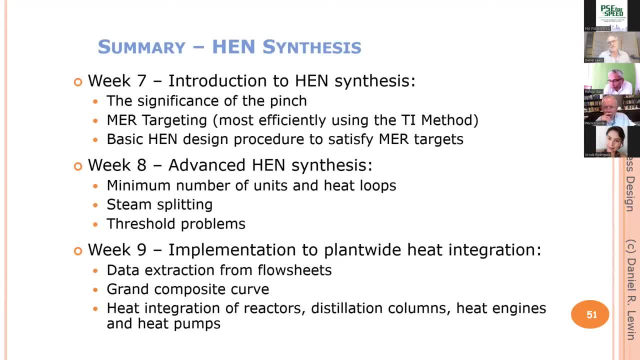 how to use the grand composite curve efficiently and how to position reactors, distillation columns, heat engines and heat pumps within a process that covers what what can do in about three weeks of lecture material and associated um exercises and with that i hope you enjoyed this video. and i hope you enjoyed this video. and i hope you enjoyed this video. 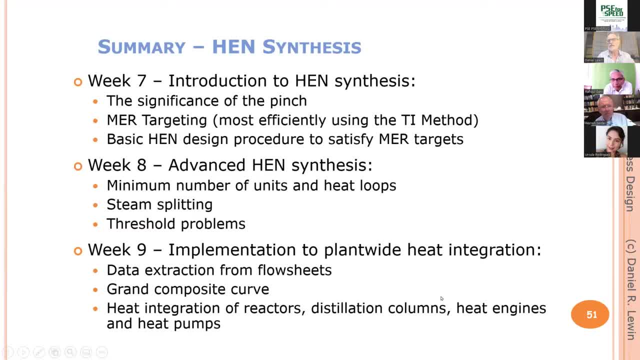 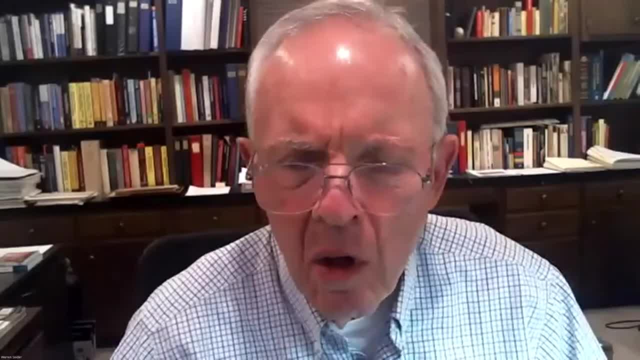 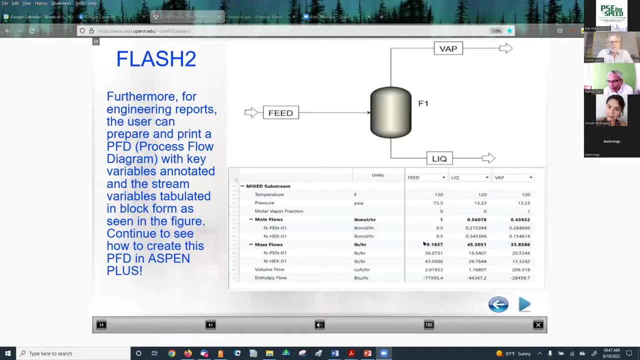 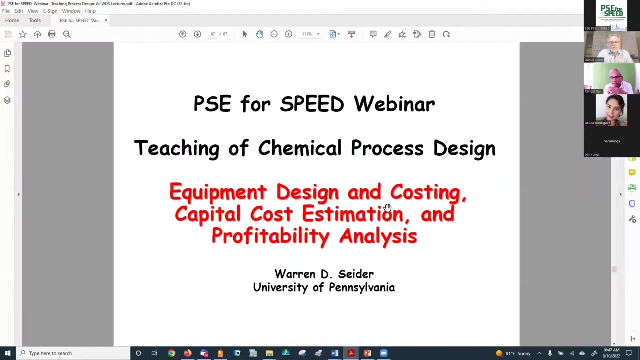 to complete my coverage of uh hand synthesis over to you, warren. okay, thank you, danny, and let me share the screen. okay now. what do i have here that i don't want, that i have to have? is this over here? okay, everyone? well, i hope you're ready for this. 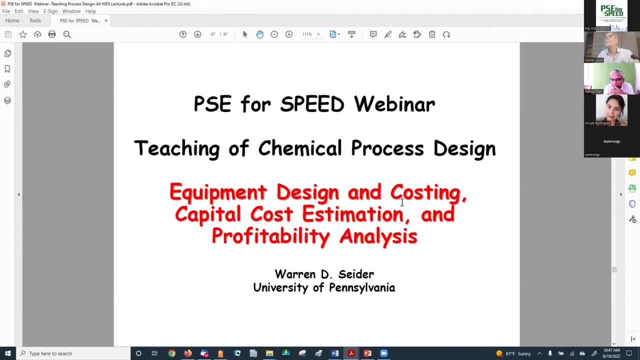 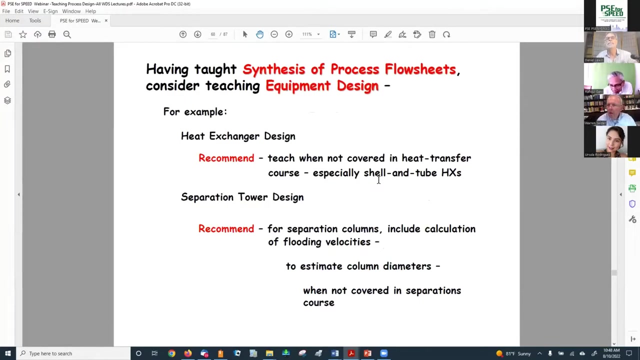 um, equipment design and costing, capital, cost estimation, profitability analysis- those obviously are key subjects throughout design. okay and uh, i'd like to offer some guidance. warren, if i, if you don't mind my disturbing you. yes, keep it a little bit shorter so we can recover some. 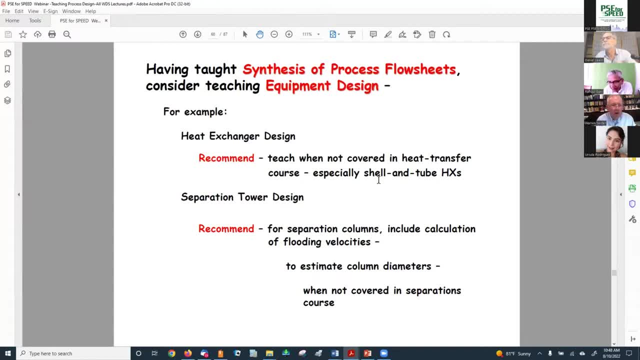 time. we are running a little bit late. i'm aware of that. uh, rafi, i will do my best, okay, um, all right, so you need to. you know, consider teaching equipment design after you've synthesized the process flow sheet. okay, so, um, do you need to teach heat exchanger design? well, it depends upon the 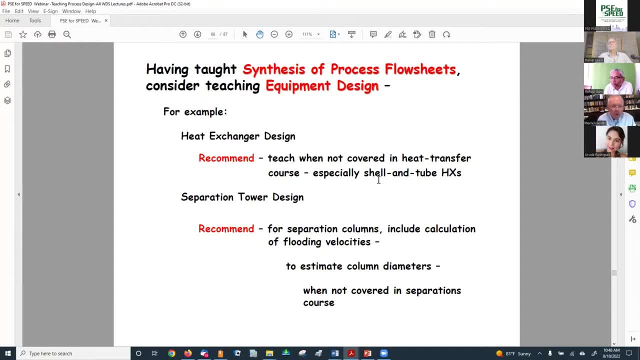 quality of your heat transfer course? is it the? they should have covered shell and tube heat exchanges. okay, we do that in chapter 10 and chapter 12.. um separation tower design? well, again, it depends on the separations course and in my view, i, the students, should be well aware of the importance of estimating the 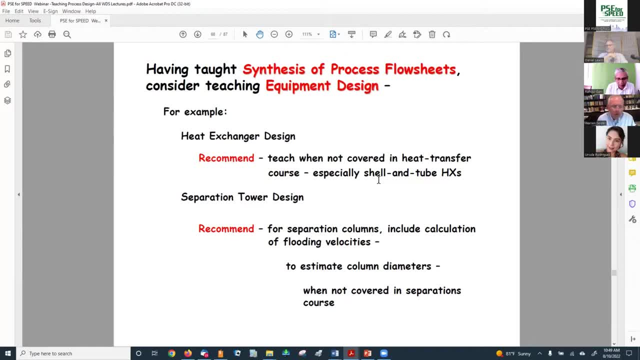 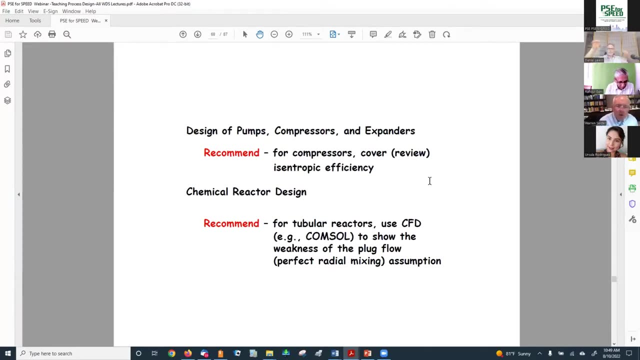 column diameter. they have to be aware of using what's involved in calculating the flooding velocities. okay, we do that in our chapter 13.. okay, i'm going to skip where this is having to do with pumps and compressed expanders and also chemical reactor design. okay, now i'd like to go to 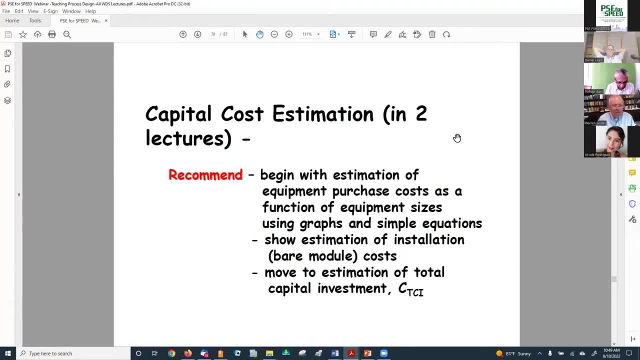 capital cost estimation. okay, so we're recommending that begin with the estimation of the equipment purchase costs as a function of equipment sizes, uh, using graphs and simple equations, and show estimation of installation- what are known as bare module costs- and move to estimation of total capital investment. so i'll try to guide you through this quickly. i think most. 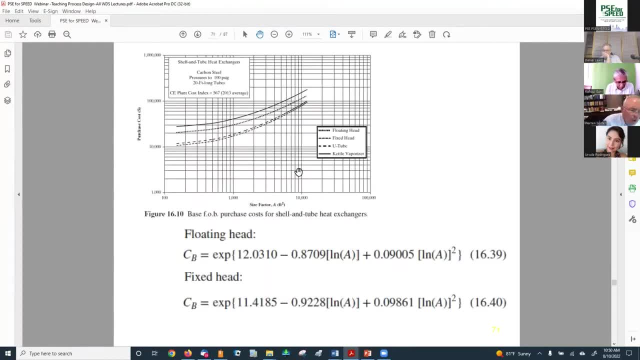 people are familiar with it. okay. so if we look at our figure 1610, chapter 16, here's for a shell and tube heat exchanger, and this is the base case. this is where you have a carbon steel exchanger. the pressures are lowest than 100 psi g. the tube lengths are 20 feet long. okay, so the purchase. 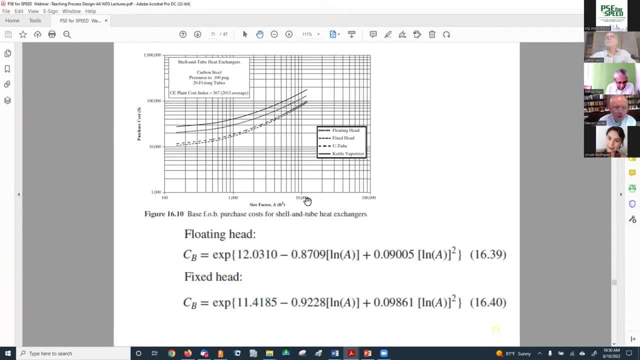 cost is a function of the size factor, which is the area. hopefully everybody here knows this. you have different kinds of exchangers and the curves then go like that. this is. these are log, log curves. if you look at the, the base cost, there's a function of the area. 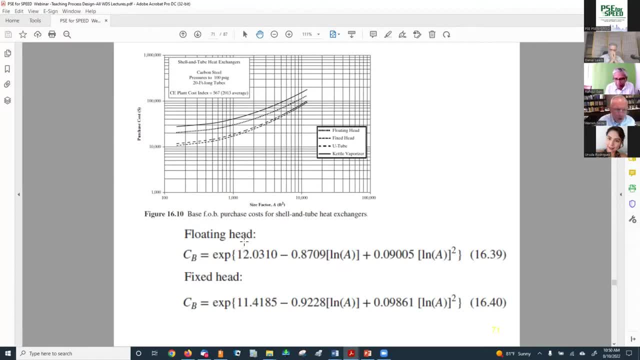 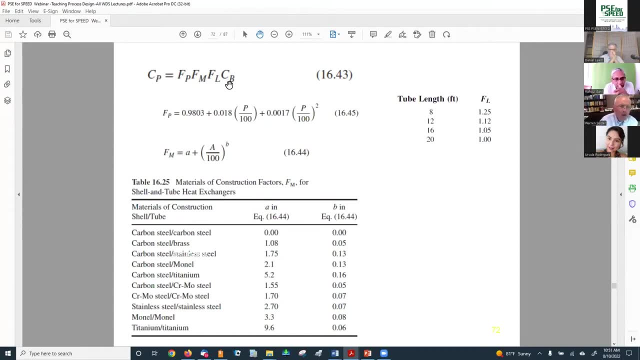 the relationship is this: for a floating head exchanger, fixed head exchanger, once you have got the cost of the base course computed, then you want to make corrections if the pressure is greater than 100 psi. we have an equation like this that gives us a pressure factor if the materials are different. 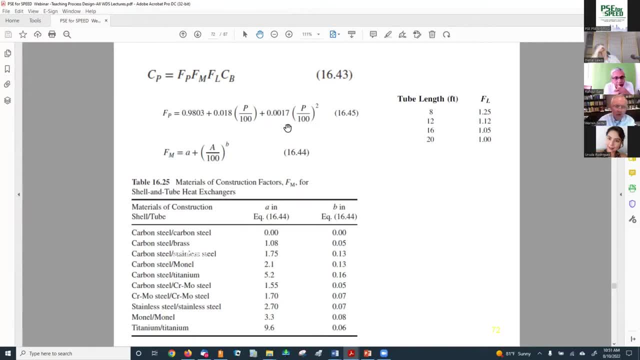 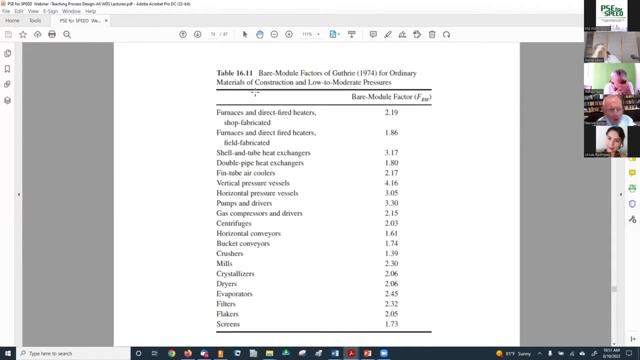 than carbon steel. we have then a materials factor. if the tube length is different than 20 feet, well, we have a materials factor and you multiply by those factors, so i'll skip through this now. in the book we spend a lot of time talking about what is it? what is involved in going from? 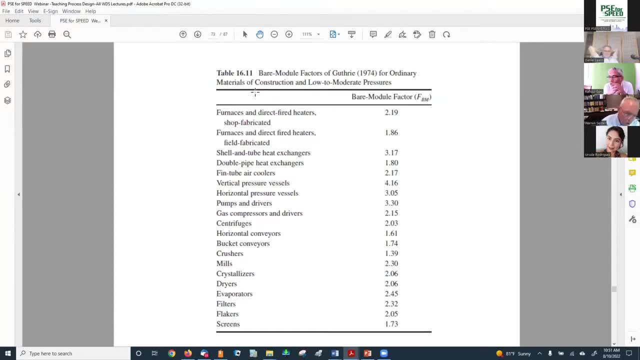 the purchase cost to the installation cost, and i won't take the time to do that now. um, in effect, we come up with a factor. it's called the bear module factor. if you take the purchase cost with the bear module factor, you have the cost of purchasing the equipment plus the cost of 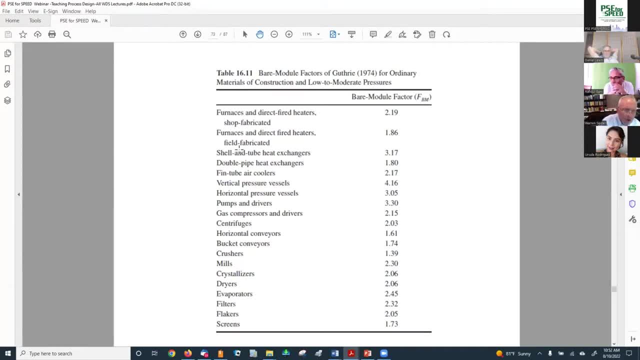 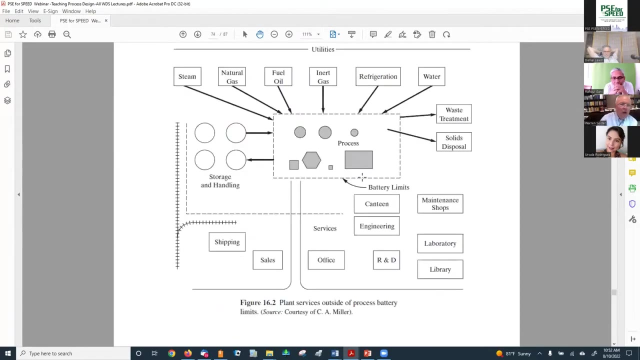 installation. this is so important. so you know this is for different kinds of vessels here: the vertical pressure vessels, the columns, all right, and then the compressors and drivers and sensors. so separate bear module factor for each. okay, now the students very badly need to understand this, in my opinion. 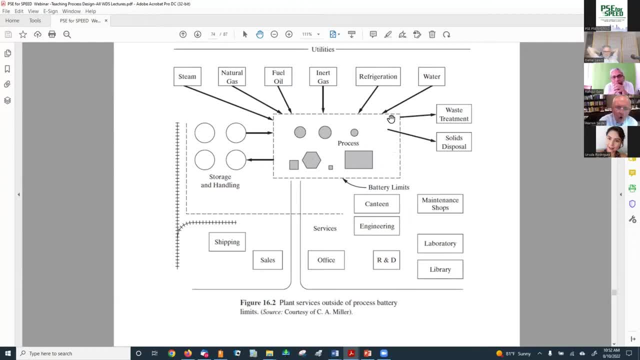 here's the battery limits. that's where all of their equipment in their process is sitting, in the battery limits. you've got storage vessels okay here at railroad tracks or the river or whatever, and you have now tanks okay where the feed chemicals are stored. those go into the process. 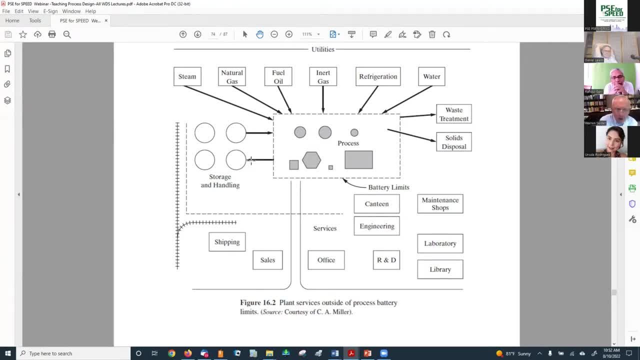 coming out of the process will be okay, um, okay, product chemicals. those will go into the storage tanks and they'll go off to for for shipping. okay, um now, uh, all processes will require utilities. so the students need to know about the utilities, all the different kinds of utilities. you can read this. i don't think. 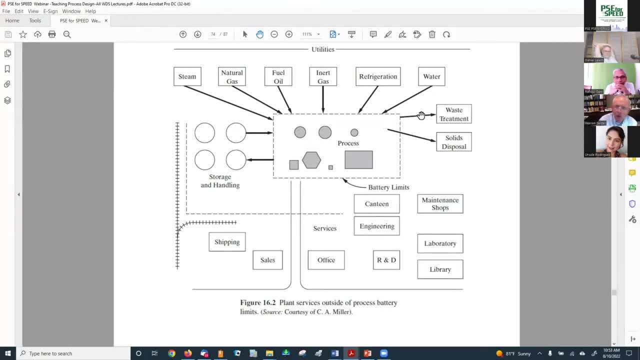 i have to tell you you need to be able to take waste streams and treat them, so we have to have a way of charging ourselves for that and and you need to have a way of disposing the solids and charging yourself for sellers disposal. oh yes, you do need canteen and maintenance. 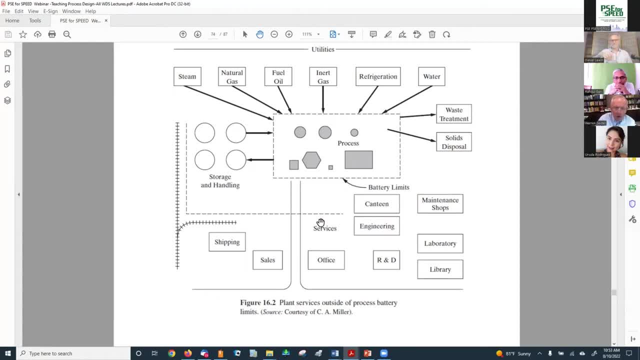 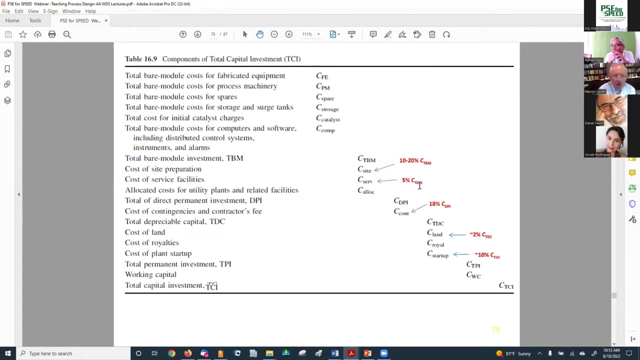 for the, for the engineers and the operators, and you need services for engineering, laboratory, library, r d office, and you need sales and shipping. all right, all of this is part of now what you have to include in in your total capital investment. okay, now to me. for my students, this is very 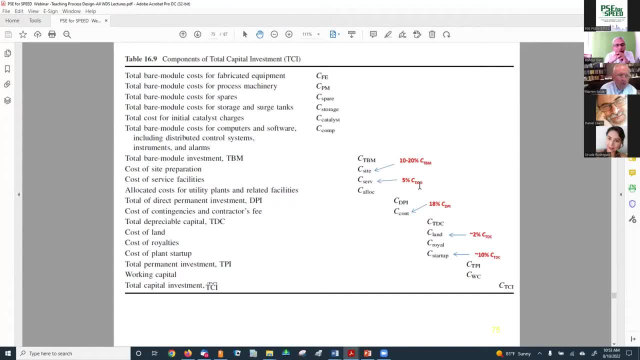 important. i think i'll take very little time for you. i think most of you all know that you need to be able to sum up the installation cost for each kind so you have the fabricated equipment, that's anything that is that doesn't have a moving part, you know, like towers for. 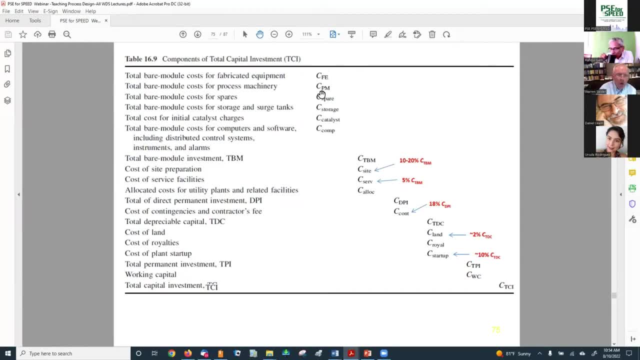 example. okay, and you sum those all up, you have now the, the, the installation cost for the uh process machinery- that would be pumps and turbines and things of that sort, anything that has movement. okay, you've got spares- you got to include. you have storage vessels- you have to include. you have the cost of catalysts that you have to. 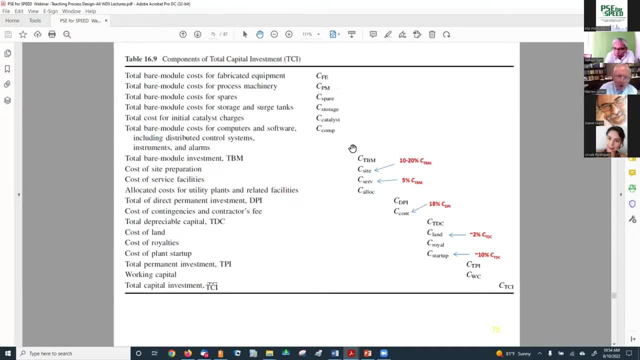 include and you may have computers and things, that you add all those things together and you get the total bare module cost and then you what you need to go and and estimate this, the cost of preparing the site for your plant. well, 10 to 20 percent of the total band module cost is. 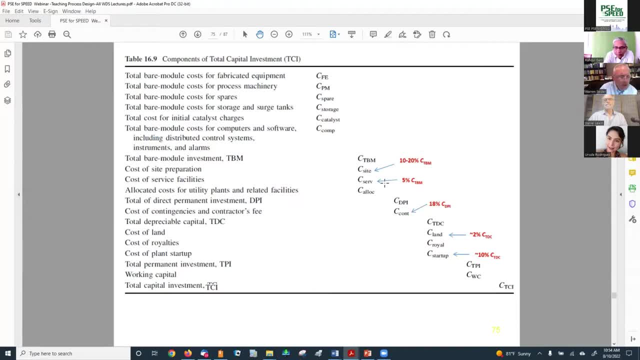 typically what's used. and then you, you need to be in a position to to for the service facilities. well, you need to be in a position to for the service facilities. well, you need to be in a position to- for the service facilities. i'll skip this, i don't have time. okay, and now you get the total permanent investment. 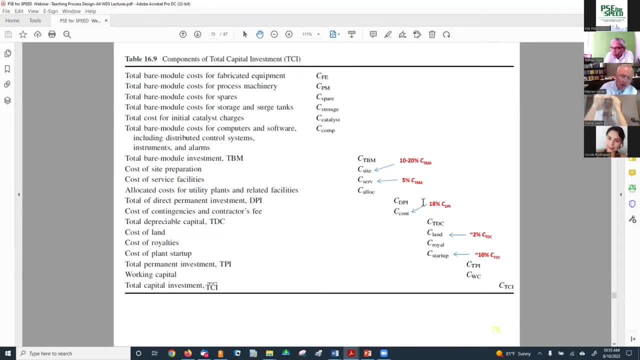 d, c, d, p, i, and you then take eight percent of that to get the cost of contingencies and contractor fees. you're in the early stages of design. you put it away an extra 18, okay, and that gives you the direct permanent investment. i'm sorry, what did i say? 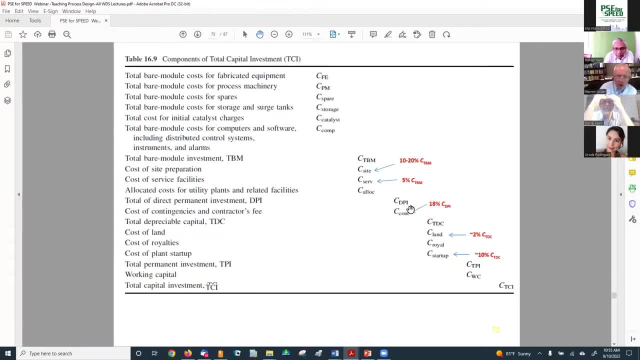 say: now, that's, there's the 18, my mistake, and that gives you now the- um, okay, the total depreciable capital. that's what i should have said. and now you have to estimate the cost of land and the cost of startup, and all right, we use these. we take a multiple of the of the total depreciable capital. 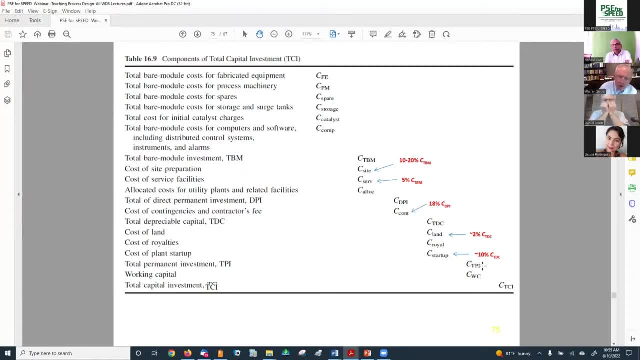 for them. okay, that gives us a total permanent investment. then, once you know the operating costs, you can then estimate the the cost of working capital, and you get the total capital investment. there's a very important part of our chapter 16 and it's discussed at length. okay, now, having done that, we asked the students 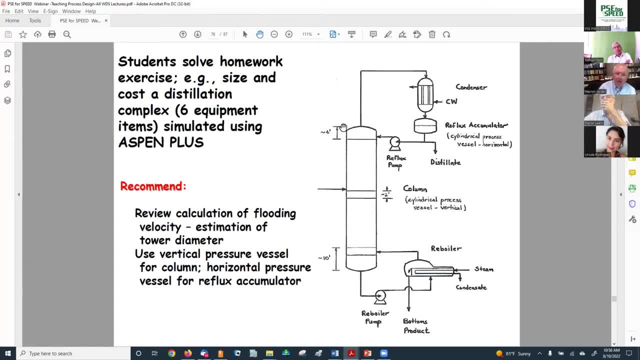 to solve a homework exercise. we say is a distillation complex. it's got the tower, it has the condenser. it has the reflux accumulator- a reflux pump. okay, the reboiler- a reboiler pump. there are six items they have to estimate. so if wejan andатель my зачем, i say that you need to. 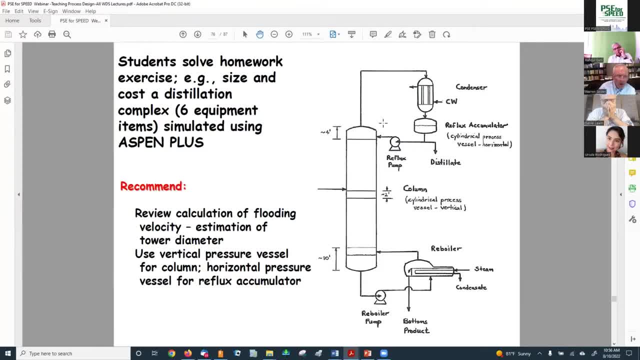 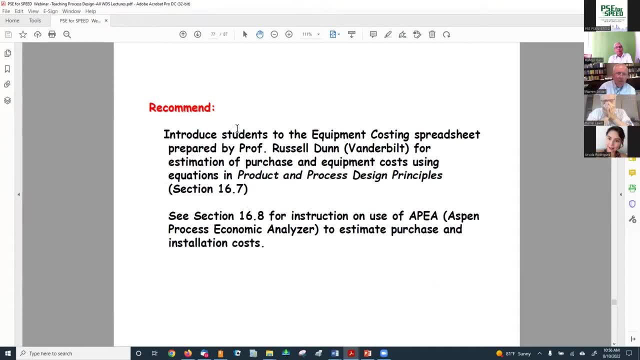 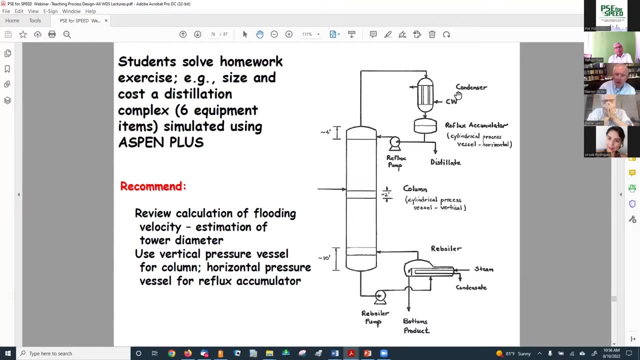 they have to estimate, So we ask them to do that And I won't go into detail at all about that. Okay, One thing that we do is, throughout our chapter 16, we have the equations that are needed to estimate the cost of each of these. Okay, Well, fortunately, Professor Russell Dunn. 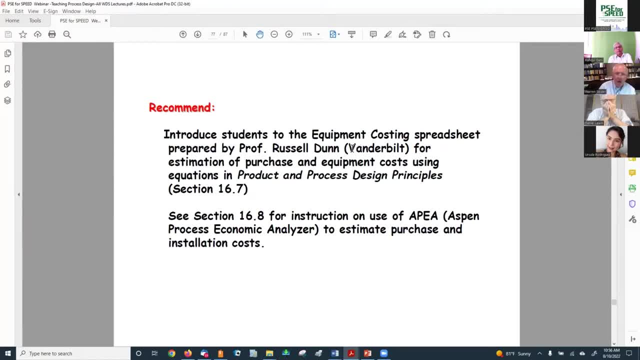 at Vanderbilt took all of the equations that we had and he programmed them in a spreadsheet and that's available and it's discussed in section 16.7.. The students use this very actively, Okay. Also, when you are running Aspen simulations, there is something called the 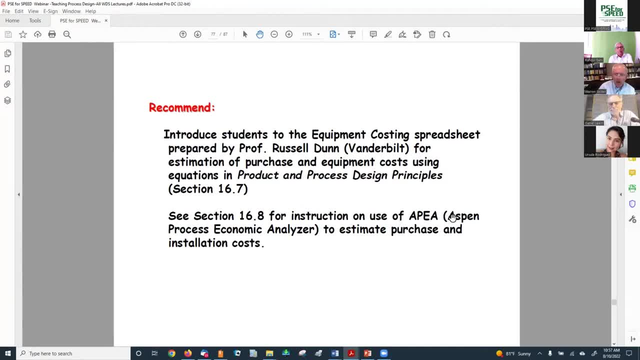 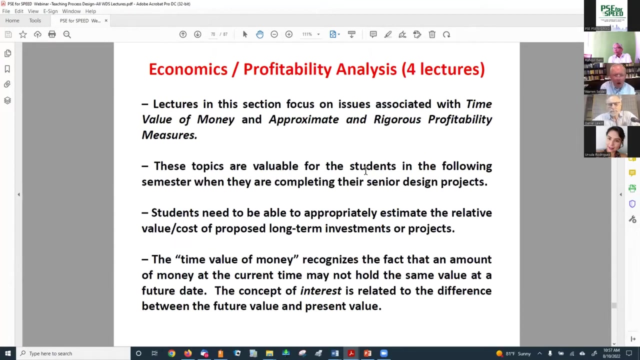 Aspen Process Economic Analyzer, APEA. You just simply ask it, okay, to estimate the purchase and installation costs, and it will just do it straight out. Okay, We give instruction in section 16.7.. 16.8 as to how to use the APEA. I wanted to mention that. Okay, Now for economics. 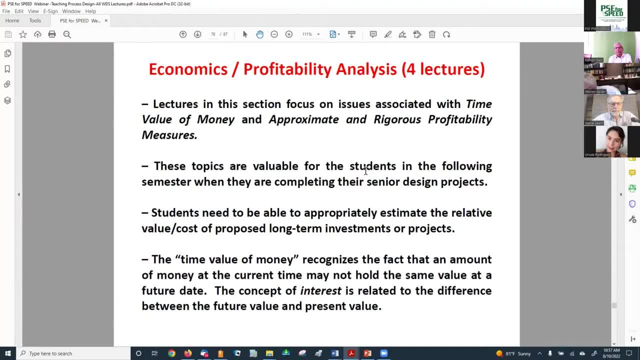 and profitability analysis. let me look at timing now. Okay, 57.. Where am I? Just a second Looking fairly good, All right. Okay, In this section, we want to focus on the issues associated with time value of money. 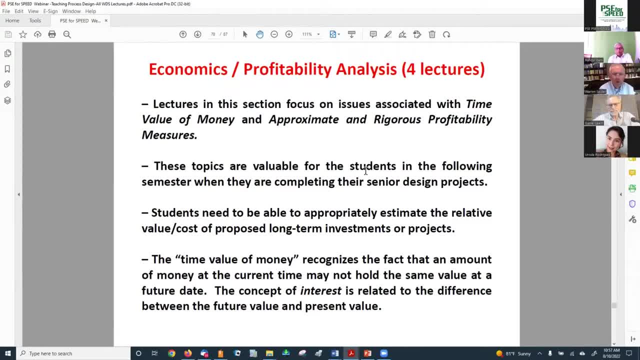 And approximate and rigorous profitability measures. Okay, These are very important for the students when they're going to do their design projects in the next semester. Okay, The students need to be able to, you know, appropriately estimate the relative value and cost of. 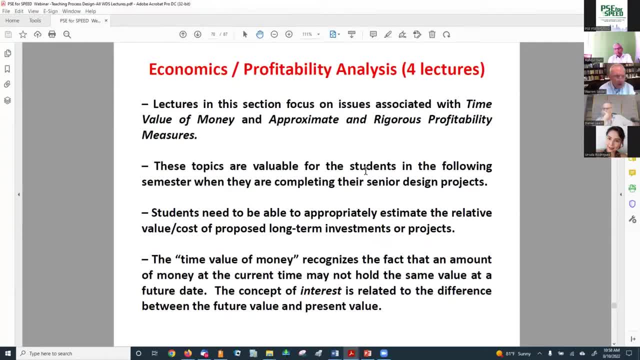 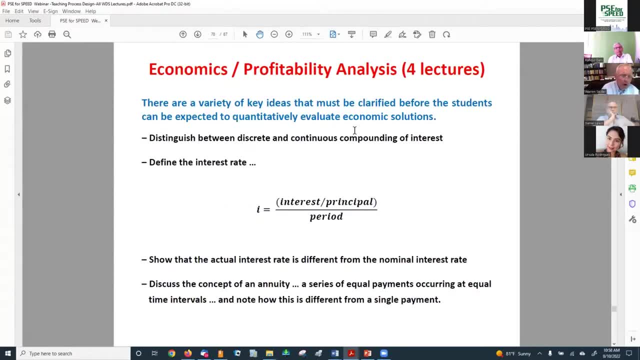 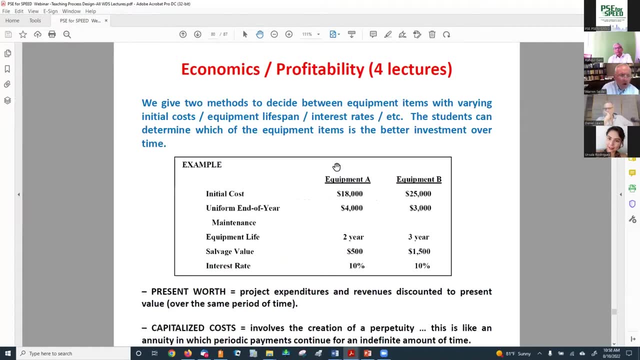 proposed long-term investments or projects And the time value of money becomes very important. So I think everyone around here knows what we're talking about. We mean by the interest rate, And I'll just simply skip past this, And we talk about how you can. 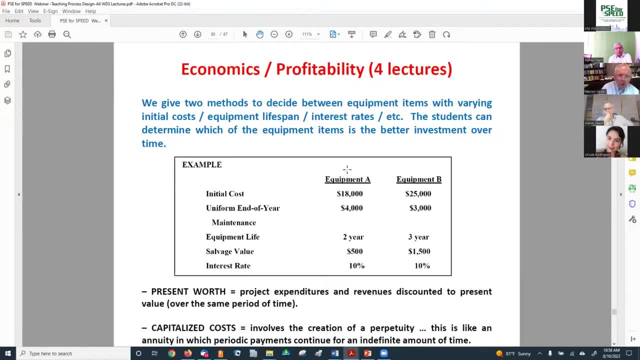 compare, okay, two pieces of equipment each having an initial cost, different initial costs- each needing a certain amount of money for end-of-year maintenance. Each one has a different equipment life- And we talk about how do you compare these, And we use the APEA. And we talk about how do you compare these And we use the APEA. And we talk about how do you compare these And we use the APEA. 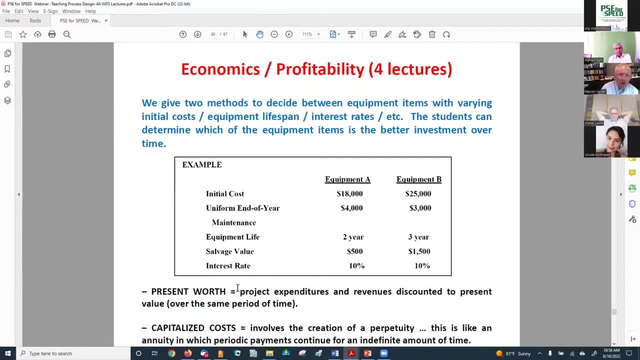 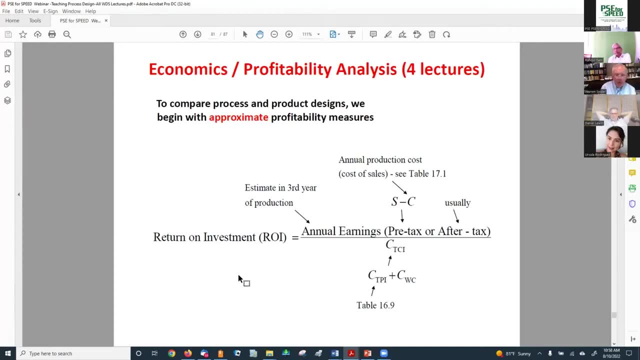 Present worth and capitalized cost method. That's a standard thing. Now, very important is when we're doing the profitability analysis. we do it approximately at first. We estimate in the third year of production the annual costs, the annual earnings. I should say 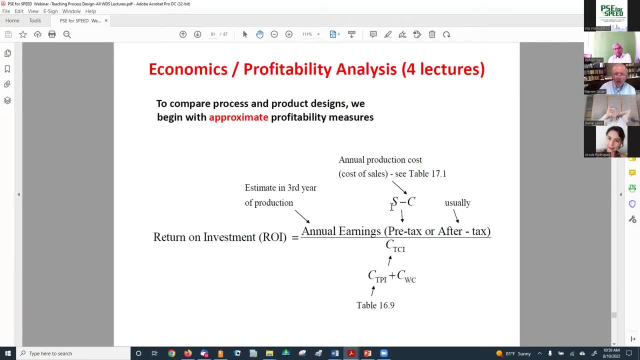 Okay And okay, how do we get that? Well, the pre-tax annual earnings is the sales, what you get in the way of sales minus your cost of sales. all right, And we discuss how to get the cost of sales in the lengthy table 17.1,. okay, Now, usually we use after-tax, so we have to take 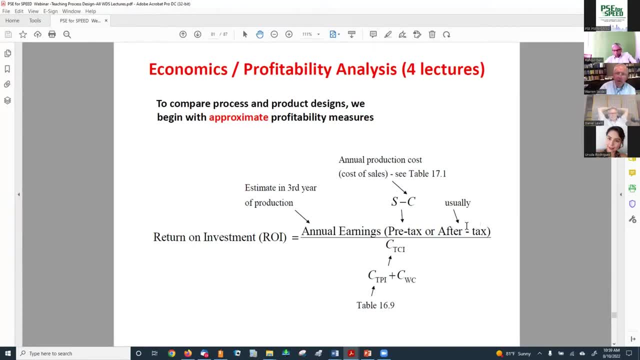 the pre-tax amount and multiply it by a tax rate and subtract that- okay. And then we divide through by the total capital investment. okay, That's the total permanent investment I just discussed and the working capital. This is the standard return on investment, ROI- Okay, other things. 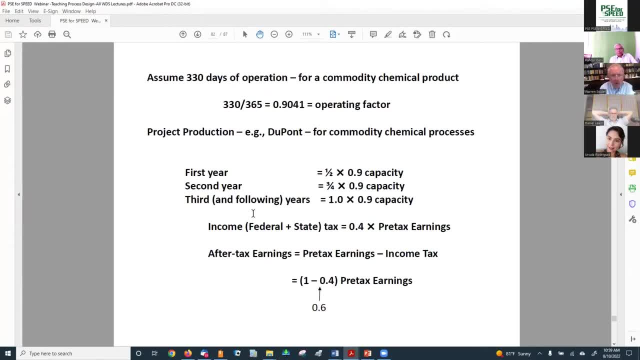 that we discuss with the students. very important things have to do with. you know just how, when you're estimating the cost of operating in the first year, the second year, third year, what we do is we say, okay, you designed the plan for 100% capacity, but you take 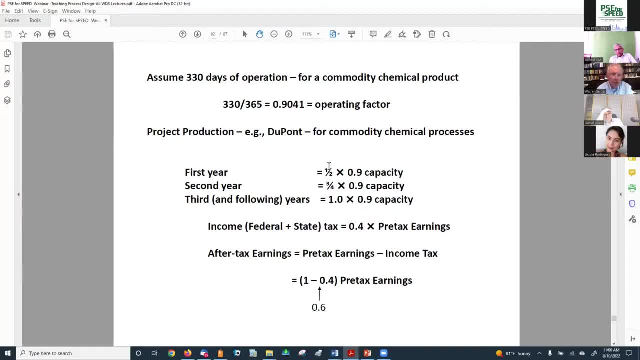 90% capacity And in the first year only a half of that, because it's going to take you a while to get to the point where you can get to 90% of capacity. you finally get to it in the third year. 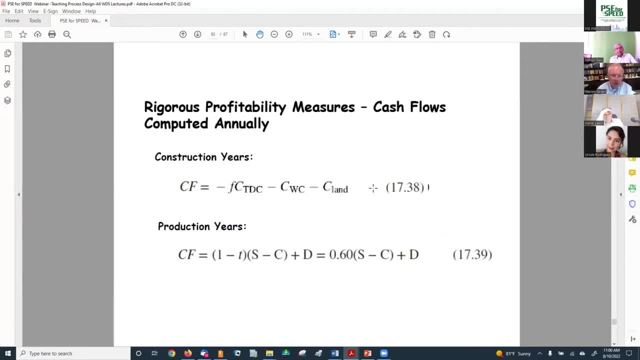 Okay, I'm going to skip past this. these things are needed. Then we, when we go to the rigorous profitability measures, we have to be concerned with the cost of sales. So you know, we have to be concerned with cash flows every year in the construction years and in the production years. 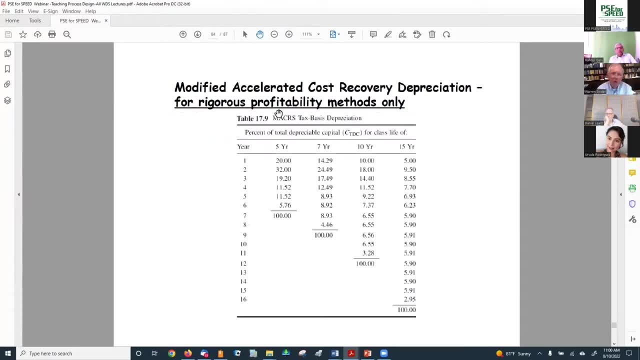 Again, I'm going to skip over that- And we have to know how to depreciate it. In the United States it's the modified accelerated cost recovery depreciation And we have a five-year schedule: seven, 10, and 15 years. Most everybody uses five years. We teach the students how to do that. 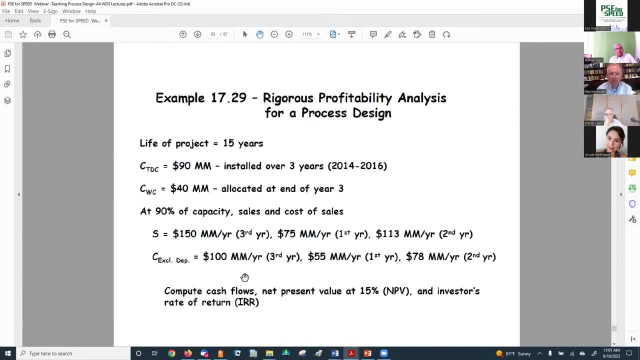 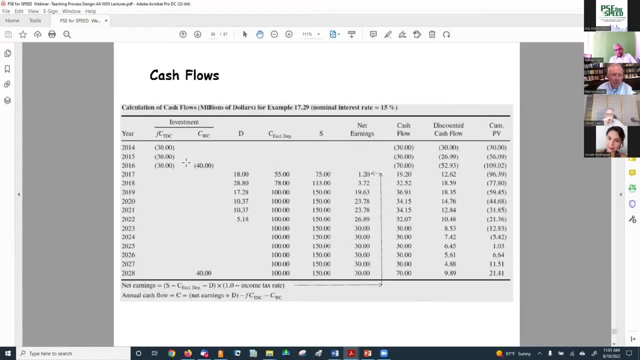 Then we take an example, a complete example, which you know, we discussed this example 17.29 in the book, and it just shows them over a 15-year life of a project. Okay, It shows them how to cap, how, in every year, how you compute the what. 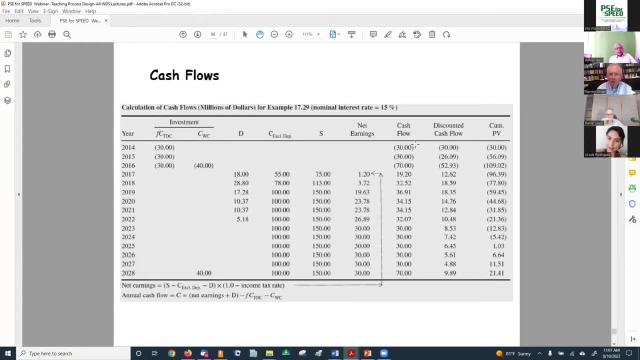 the so-called cash flow. And then what you do is you take the cash flow and you discount it to present value- All right, That's in the same value here- And then you take the cash flow and you your cumulative present value is just that 30 million. Okay, Now, all right For the second. 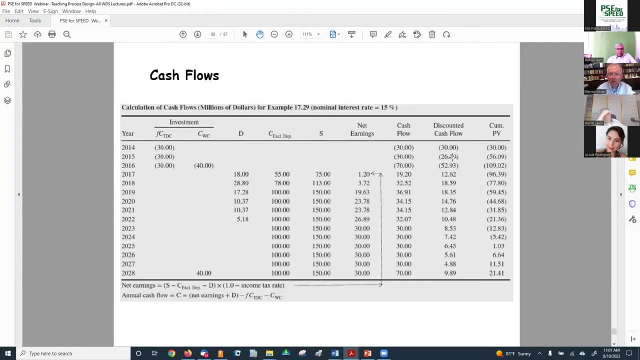 year it was 30 million, but you discounted back a year at 15% interest rate, And now these two get added together. Well, this shows them how to now take the cash flow for every year and simply discount it back and get the cumulative present value. Okay, This is a very important measure. 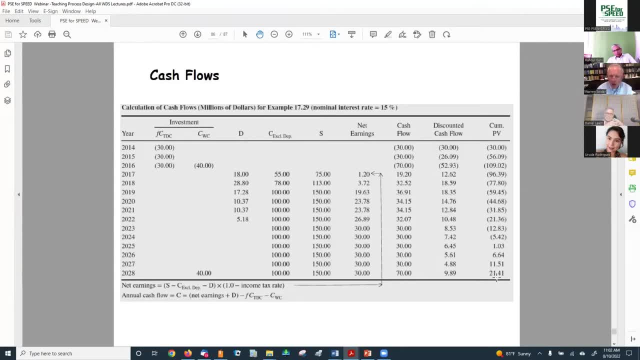 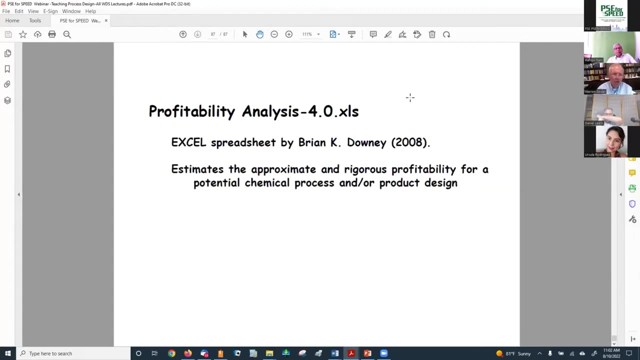 This is called a net present value And we then teach them: if you set the net present value equal to zero, what would the interest rate be? That's a very important point that we call that the investor's rate of return. So I'm skipping over that now with you And a very important part of what we do for our students. 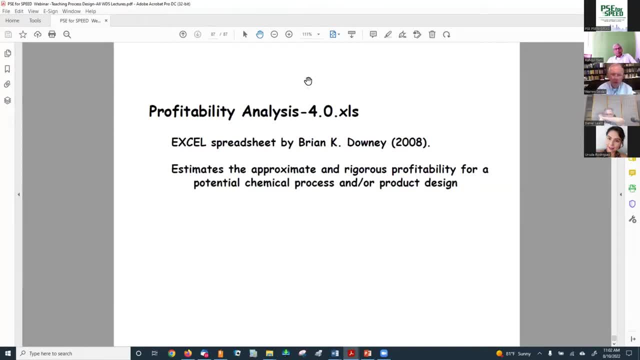 is we discuss in the in the book, in chapter 17 at the end 17.8, I believe, the profitability analysis spreadsheet that was designed by one of our former undergraduate students And this will estimate the approximate and rigorous profitability for a potential chemical. 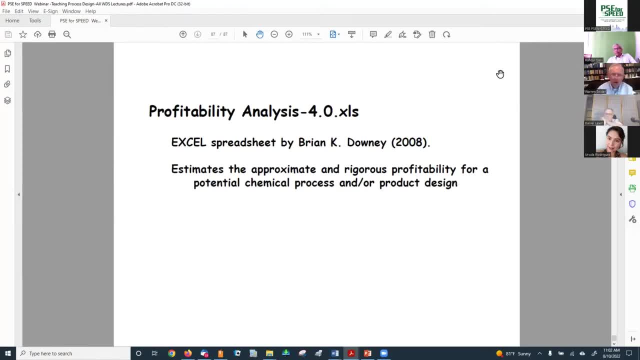 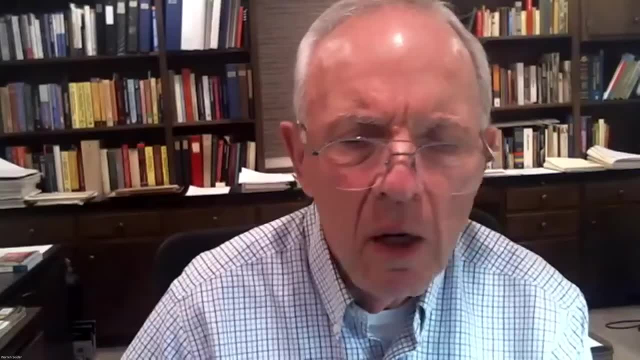 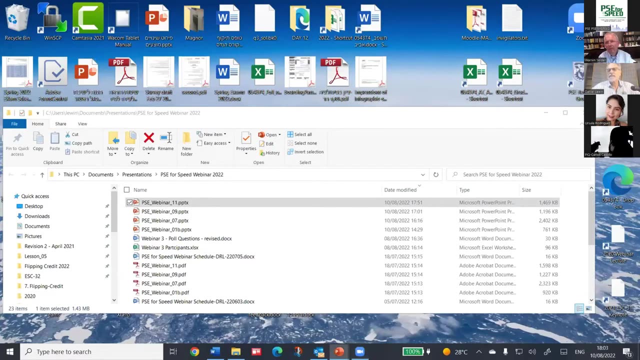 process and or product design. So that's it. That's all I have to say for that. So now I'm going to stop the share and I'm going to turn it back to Danny. So, Danny, in the interest of time, can you just briefly say the importance of plant-wide control, And then we can take the 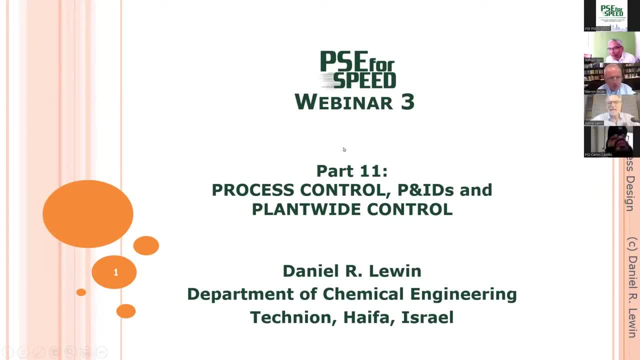 questions. You're muted. Yeah, actually I am reading my chat, So I know what you want me to do. I'm going to give a very, very brief description of materials that we teach in the 10th and 11th week of the capstone design. 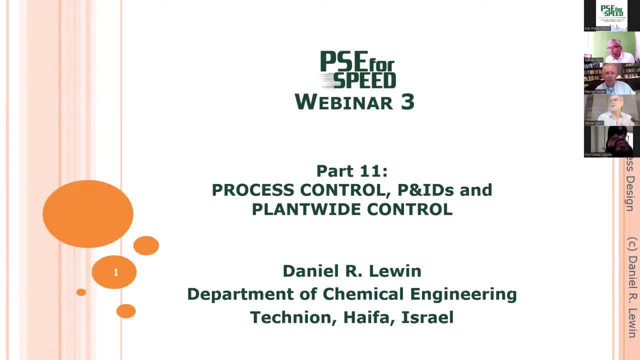 course. Basically, it covers process control, considerations for individual units and complete processes, as well as teaching students to draw process and instrumentation diagrams. I will give you a very short overview Of what is covered at the Technion in four hours of online lessons, four hours of class meetings with students and six hours of active tutorials. 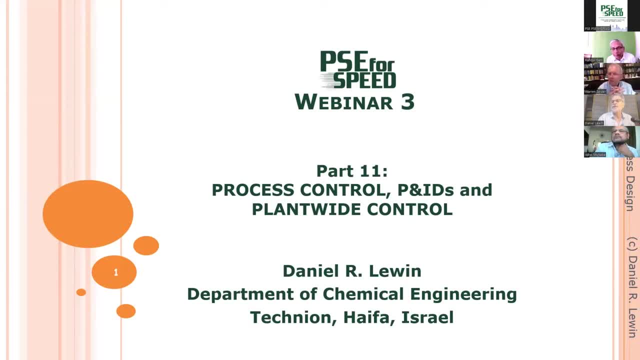 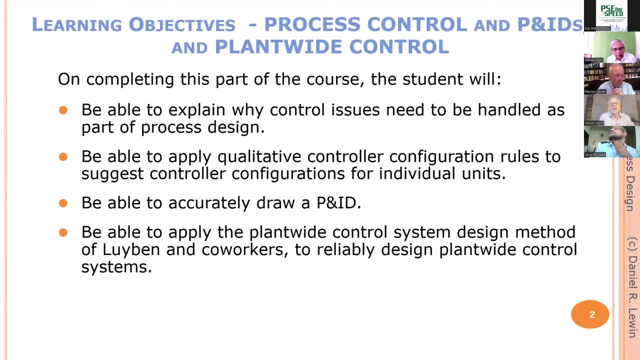 Much, but not all, of the materials that we teach in this part of the course are taken from chapter 20.. So the learning objectives are quite straightforward. On completing this part of the course, the students should be able to explain why control issues need to be handled as part of the process design. 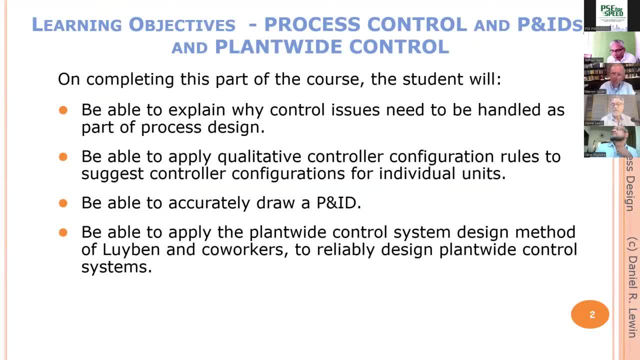 They should be able to apply qualitative control of configuration Rules, to suggest controller configurations for individual units, to be able to accurately draw a P and ID and to be able to apply the plant wide control system design method of Lloydman and coworkers to reliably design plant wide control systems. 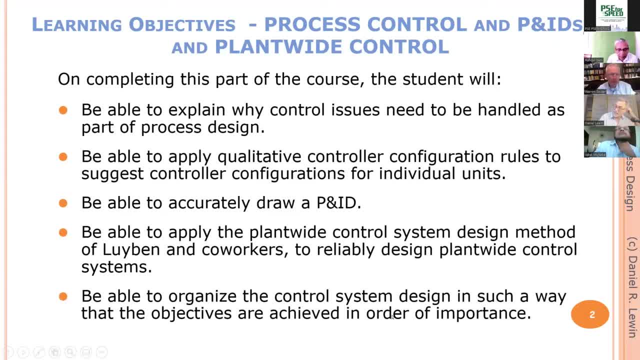 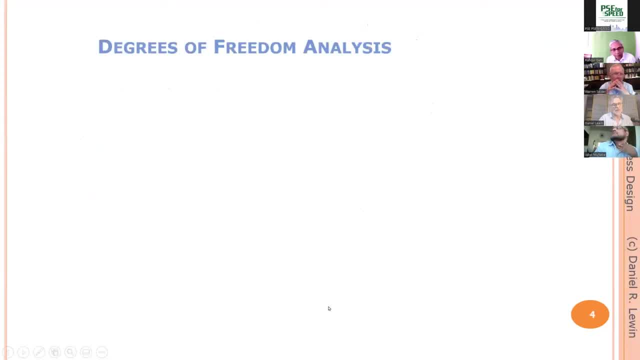 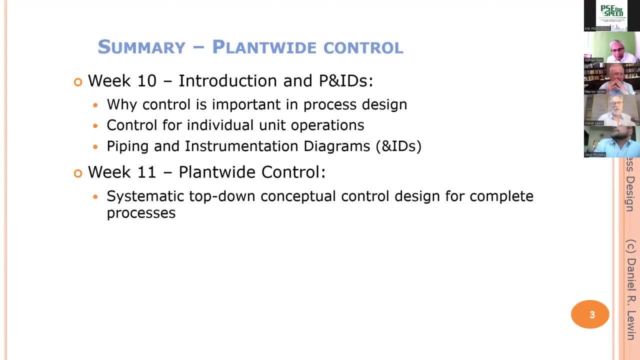 And basically, this allows the organization, the control system, design, so that the objectives, the controller objectives, are achieved, in order of importance. So, in summary, this is what we do in two weeks. Why is control important in process design? Basically, if we are not able to control our process, there's no point in doing the design. 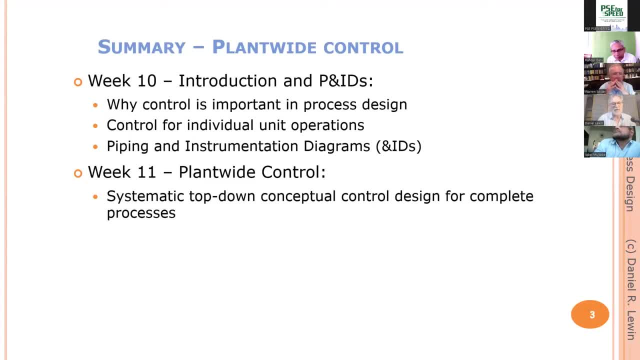 In order to ensure that our design is is appropriate, we need to be able to show that we can control what we design. This may require the additional addition of more degrees of freedom- bypasses on heat exchanges, for example- which will change everything in the design. 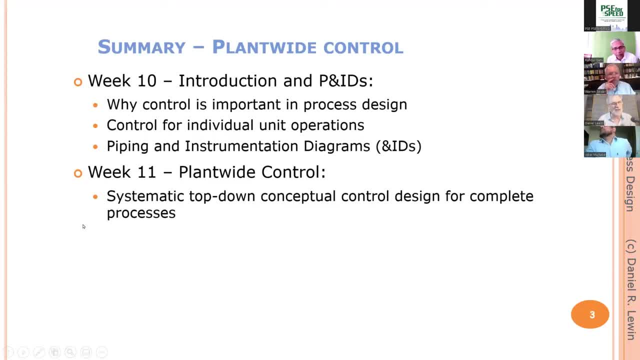 So, therefore, that has to be done in advance. in my plant design course, which is the extension of the capstone course, The first task that I give my students is to design a complete control system before they do any design at all, any detailed design at all. 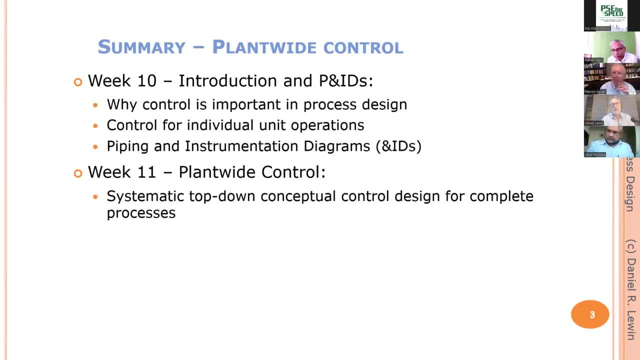 This involves controlling individual unit operations and also learning to use the piping instrumentation diagram, which that's a P and ID, not an ID. There's a P missing In the second week of the two-way segment. basically, we cover the Lloydman approach. 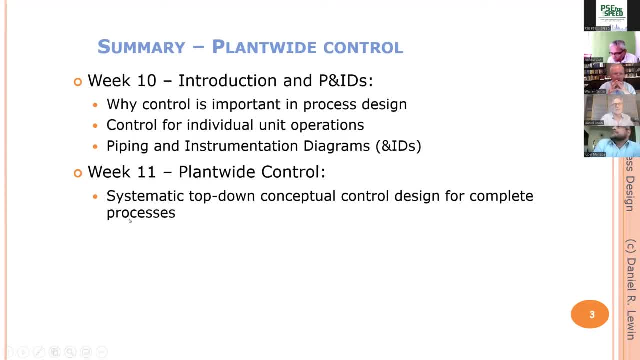 to conceptual control system design for complete processes. That's a very, very short summary. I prepared obviously more material, but we are really running out of time, So with that I will close my discussion on control system design and how it is included in the design course. 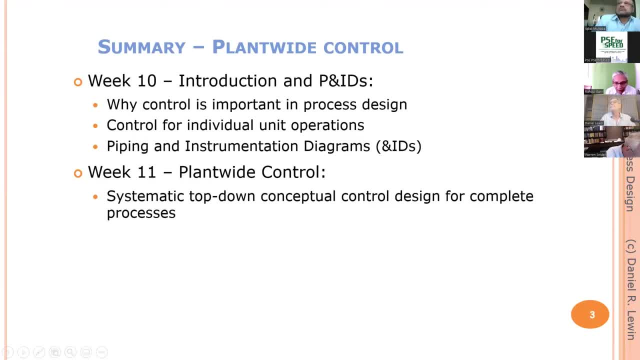 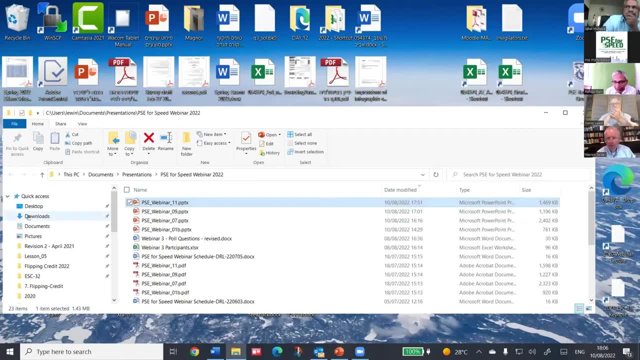 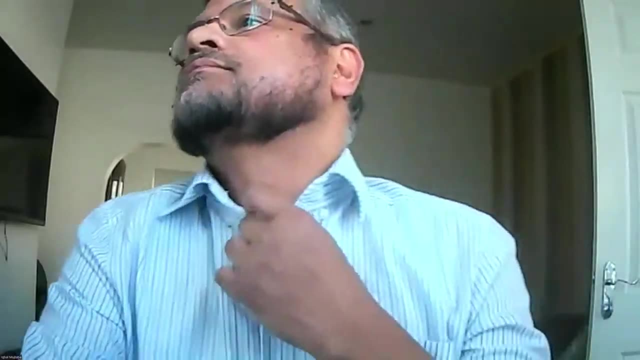 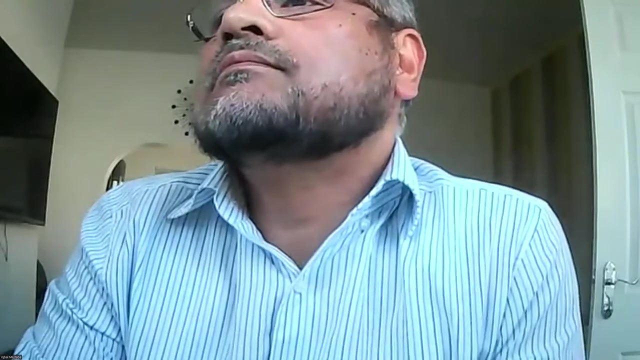 Thanks. So thank you very much, Danny and Warren. Before Iqbal starts with the discussion on the third part, And he will take the questions that are still in our system, I just want to remind all the participants that you will now receive the poll for this webinar. 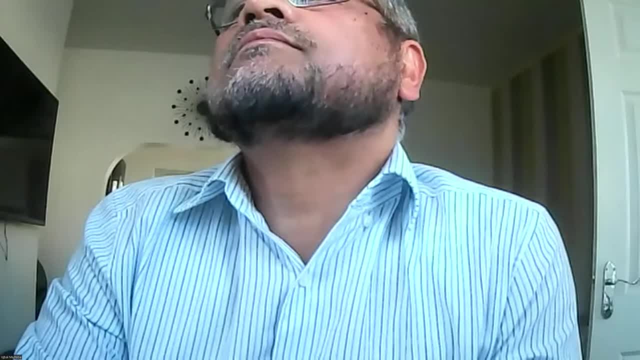 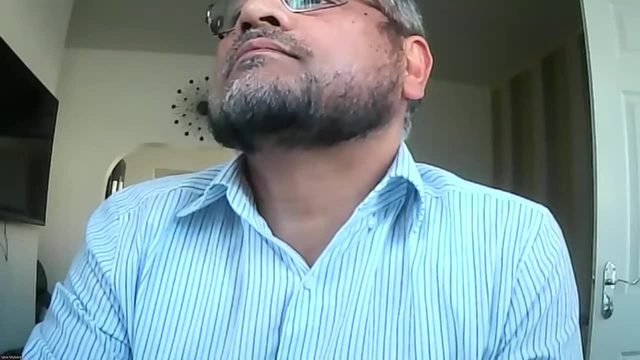 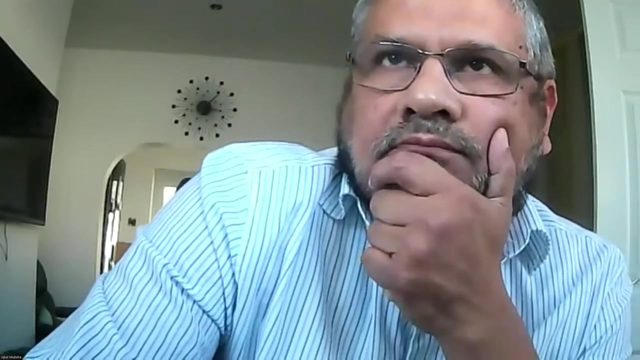 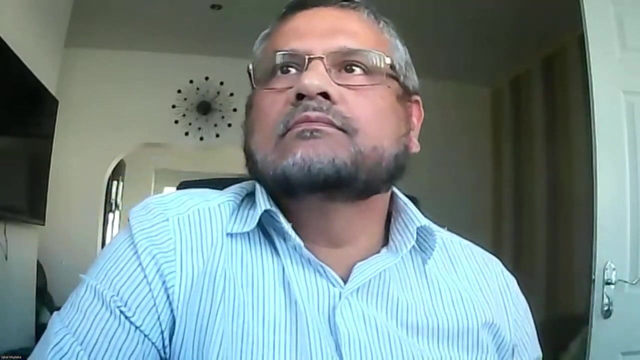 There are eight questions. Please answer the poll, so it will be useful for us. And then Iqbal will start and I will give Iqbal about 10 to 15 minutes And then after that, Edwin will start And we can continue as long as Edwin and all of you are interested. 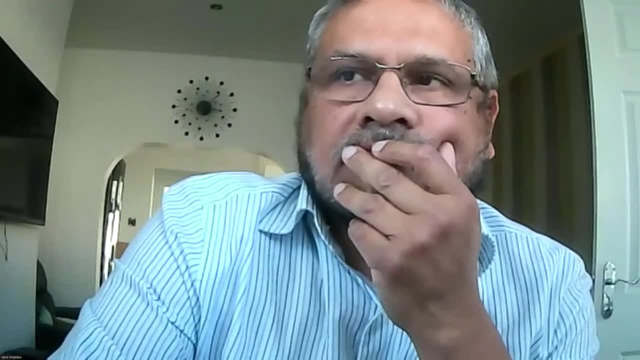 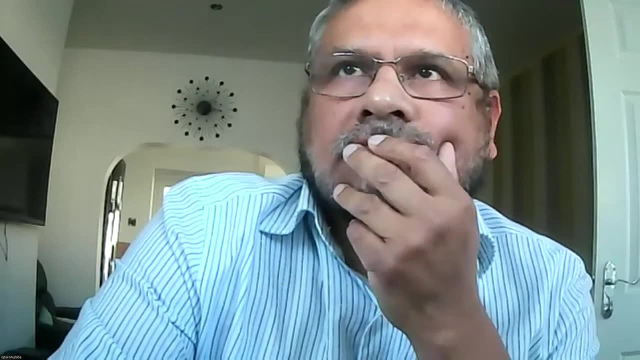 I know that Edwin has to attend to a birthday party also. Just for the record, right now there are 66 participants. I'm going to keep looking at that window now See how many. Yes, Yes. So we have to also think that people should not leave. 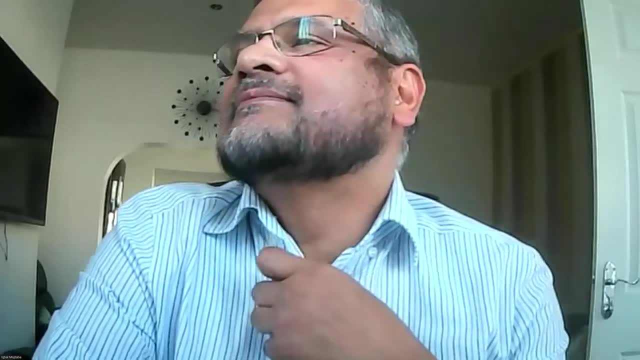 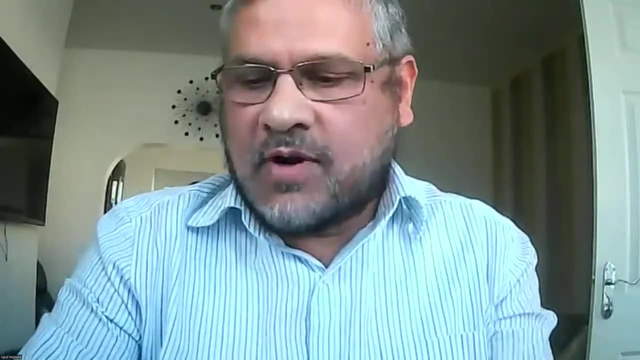 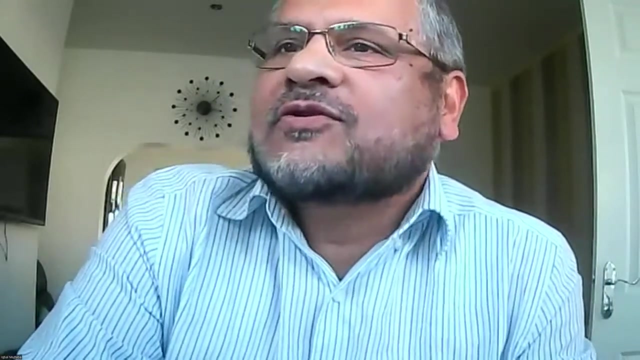 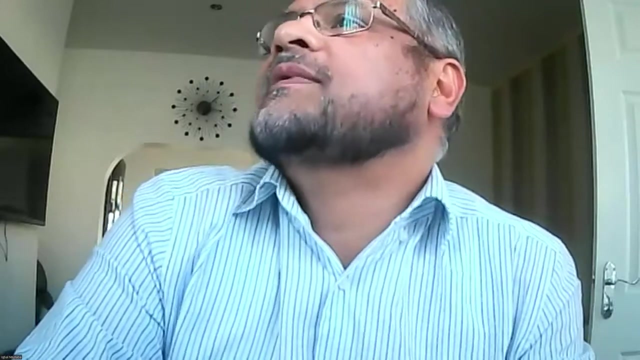 Okay, Okay, Iqbal, please. Good afternoon, Good morning everyone, And thanks Danny and Warren for very useful insight in heat and power integration, as well as costing and control. I can see a number of questions on the chat box that I would maybe pick a few of them. 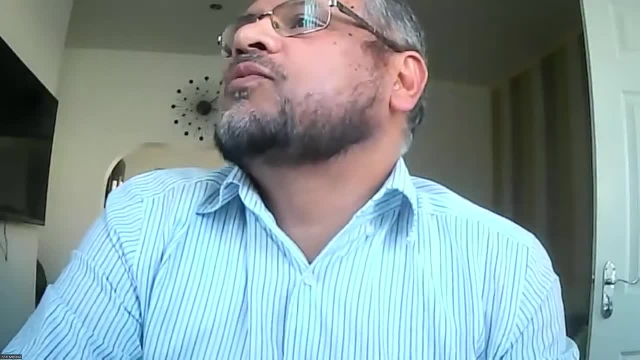 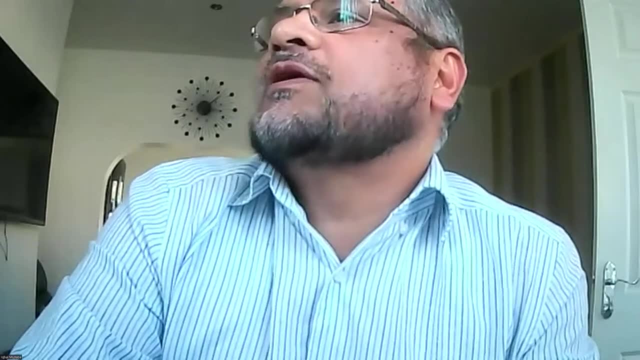 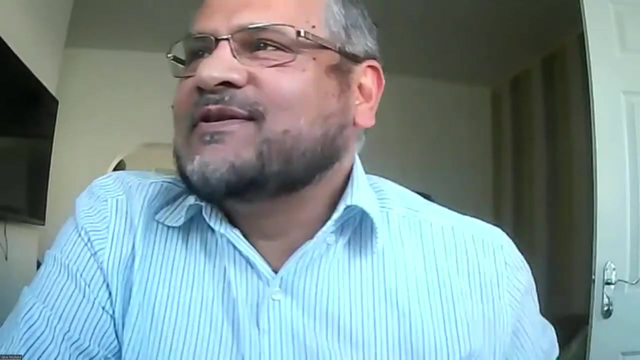 The one we left with from Shesha- From Shesha Gary Rao, where the question was whether a specific design course is required for a Bachelor of Petroleum Engineering program. I think this question is relevant to us at Bradford as well, as we are planning to embark. 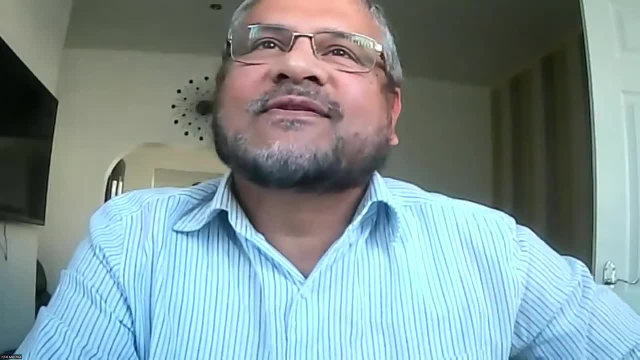 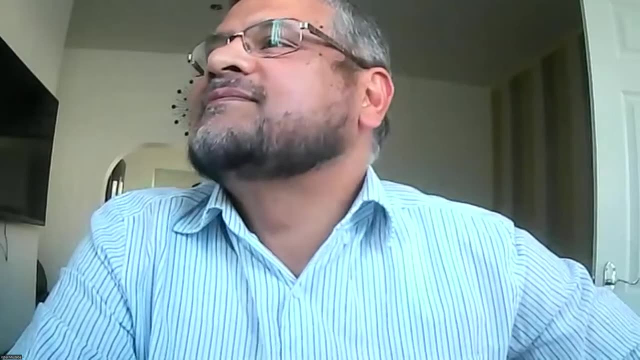 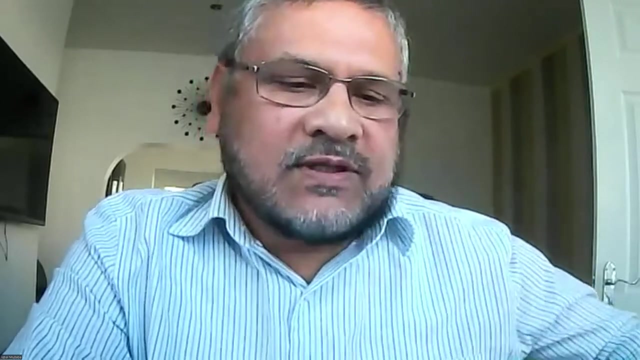 on new petroleum engineering program. So to the panel. I'm not sure that I understand the question. I'm not sure that I understand the question. For example, For example, Danny, if we'd like to introduce a course in Bachelor of Petroleum Engineering. 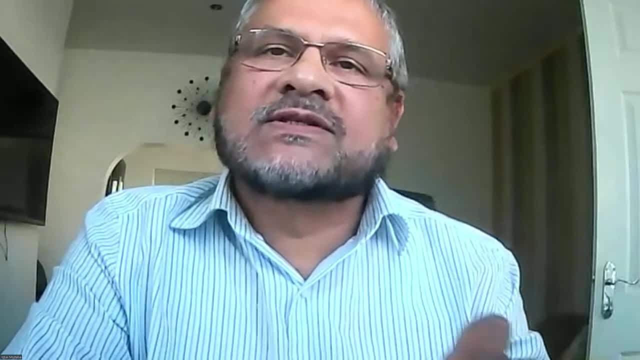 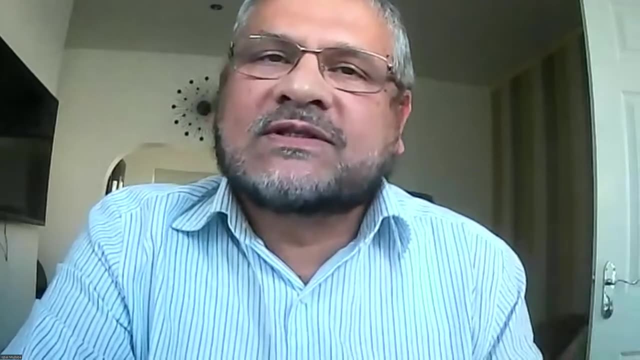 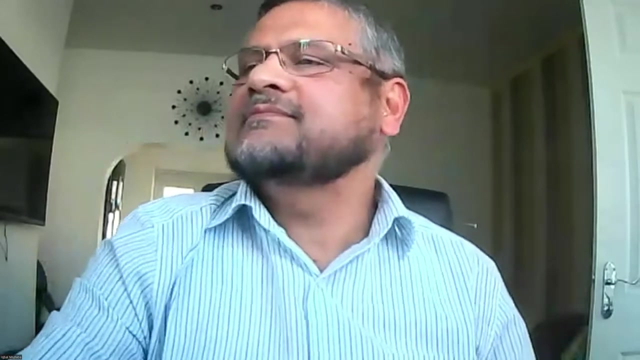 will the similar process, design or design project will do, or do we need a separate or a more specific process, design course or design project? My take is that, unless you're talking about petroleum extraction, which would require additional segments to be added, If you're talking about petroleum extraction, 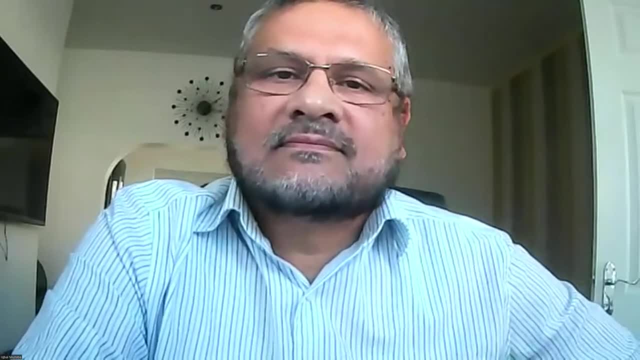 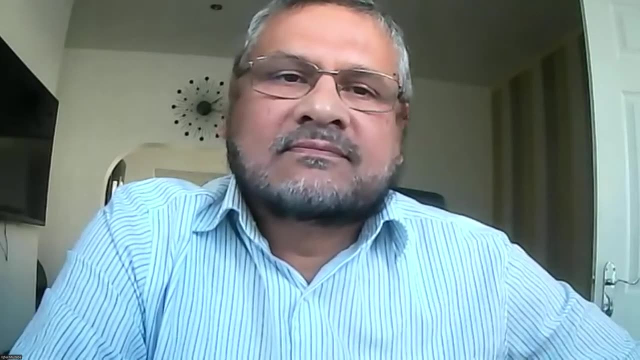 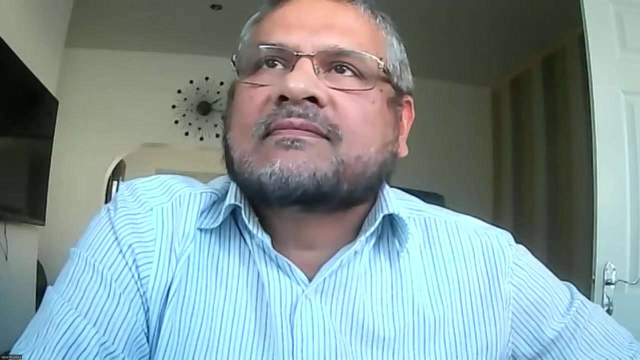 If you're talking about processing, it's in, It's all in, And I think the way to make it real and relevant to your course would be to make the design project relevant to your course. You have to use a process simulator that can handle modeling of crude oils for as long. 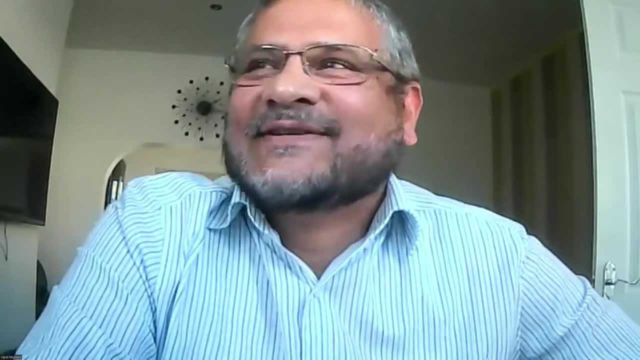 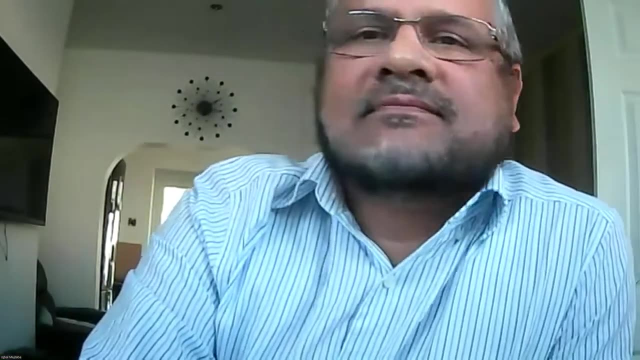 as we'll have crude oil to process. of course, Yeah, but I mean I think they all do that. I know Unisim has that capability. I'm absolutely certain that Aspen also has this capability, So there's no problem giving students a petroleum based project to work on. 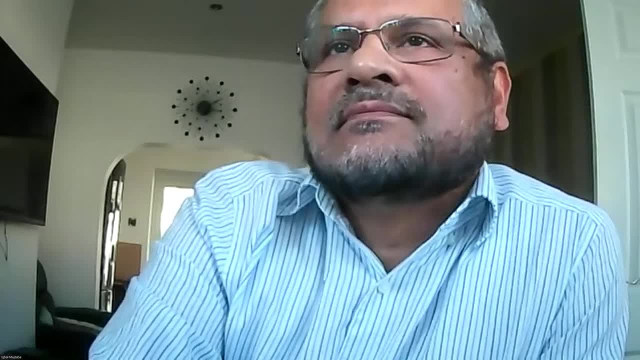 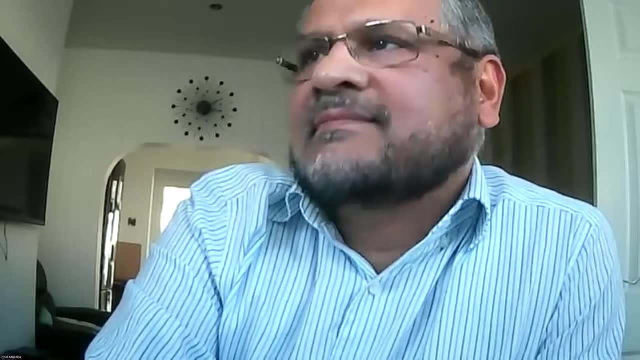 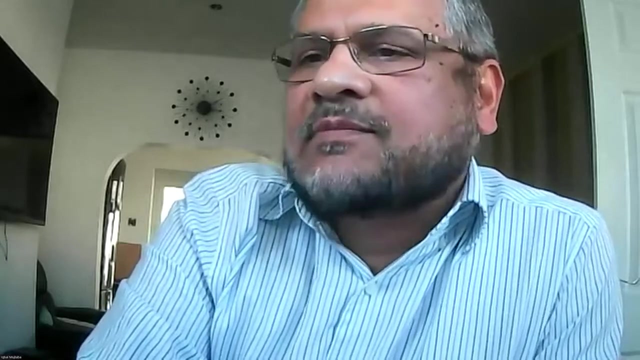 And that that's what will make the course real for them, because they're working on an absolutely relevant project. That's my take. Maybe Warren has other. No, I agree with that, Danny. Thank you, I've got a question on engineering ethics which you can see on the chat box, but you 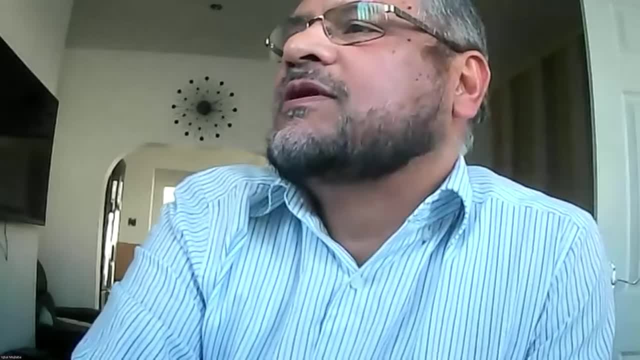 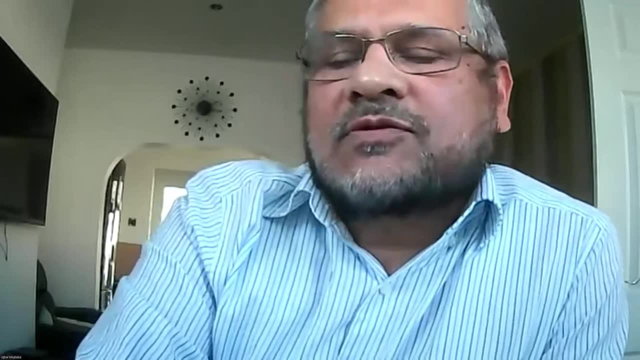 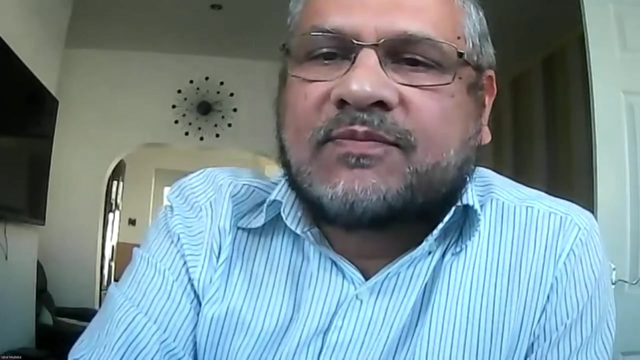 may want to respond in writing, So I'm not going to go into that and move on to the next question from Dr Juarez Romero. It is about whether we should have one design project for the whole class or separate or multiple design projects. 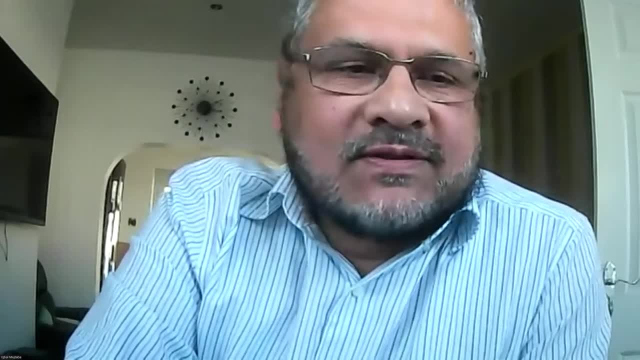 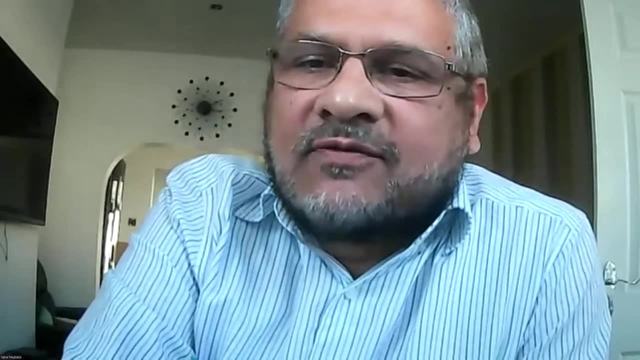 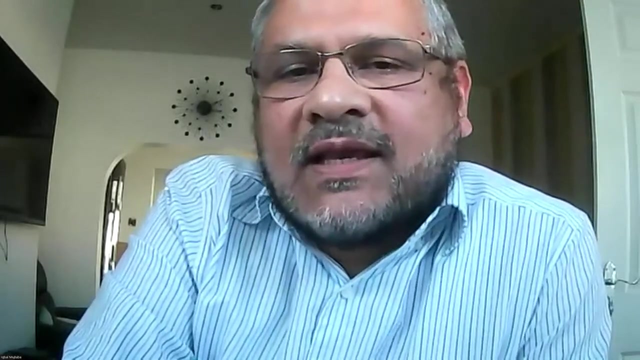 I can share with you our experience in few UK universities. For example, at Bradford we have got multiple design projects, about eight to 10, for a class size of 70 to 80. Well, I know that Hull University they have got one single project for all of their students. 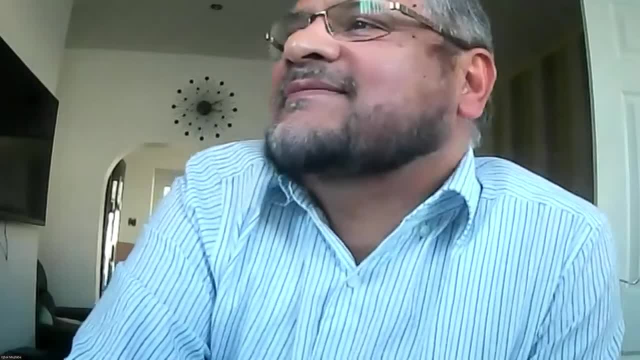 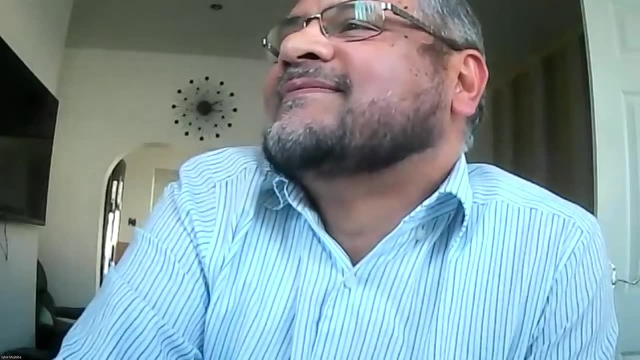 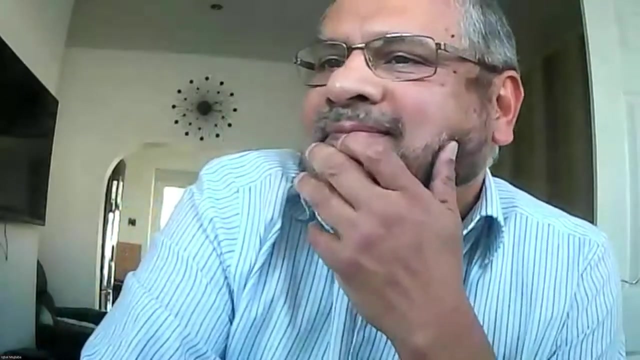 Is there any view on that? Warren, you answer first. Well, you know I have spent at the University of Pennsylvania for the last 75 years, has had separate projects for groups of three students, And you know I've been at Penn now for 54 years. 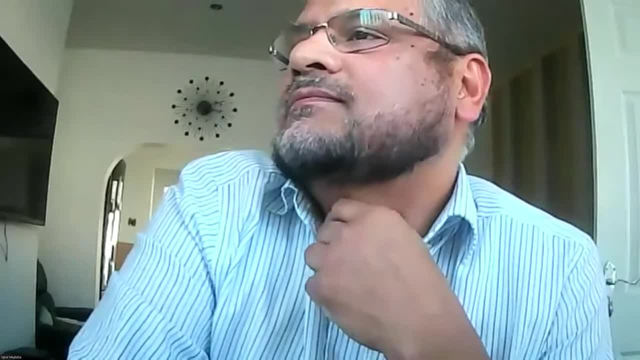 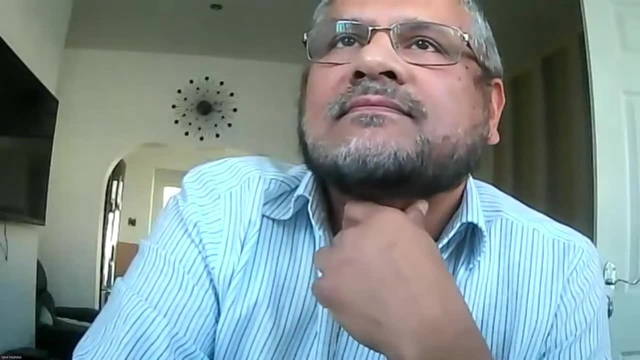 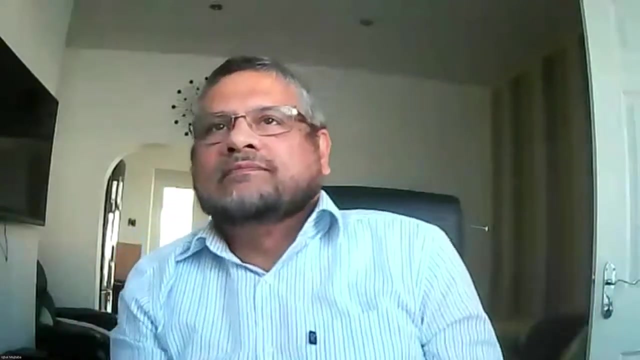 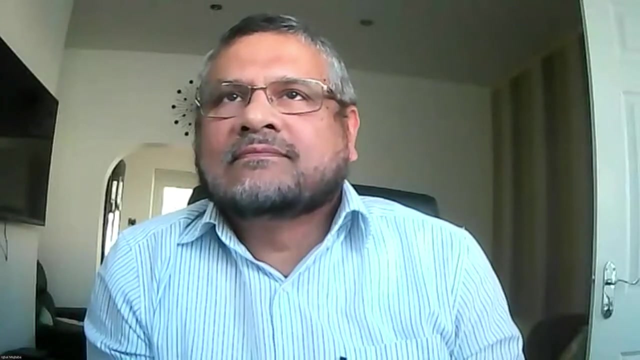 So this clearly is an approach that I understand and appreciate. In the early days we could do that because we had so much chemical industry up and down the Delaware River in the Philadelphia area. So the people from the companies would come and they would consult with our students as they were working on their problems and give them advice. 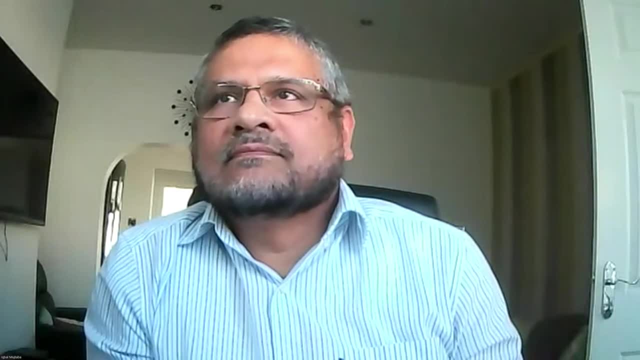 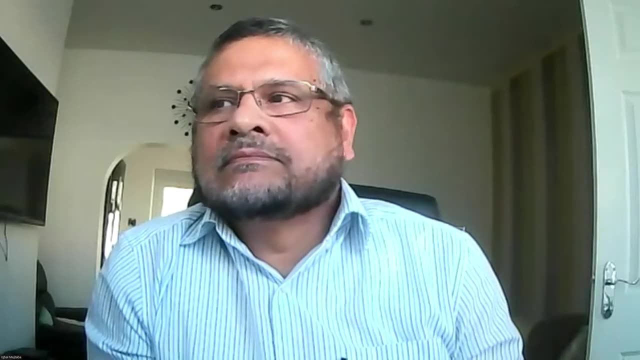 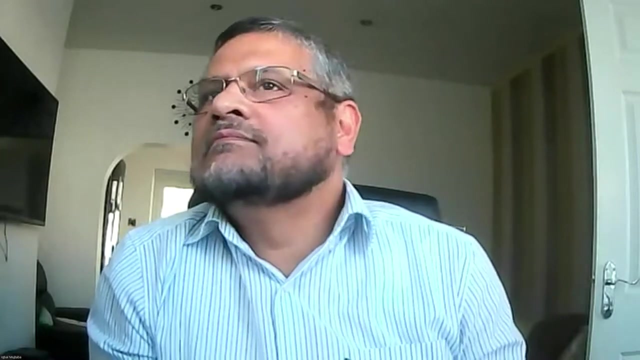 Okay, As years have gone by, though, We now have the Zoom communications. It doesn't really matter where they are, And so it is now possible to get a group of consultants together from all over the world, And we do have them from Beijing. 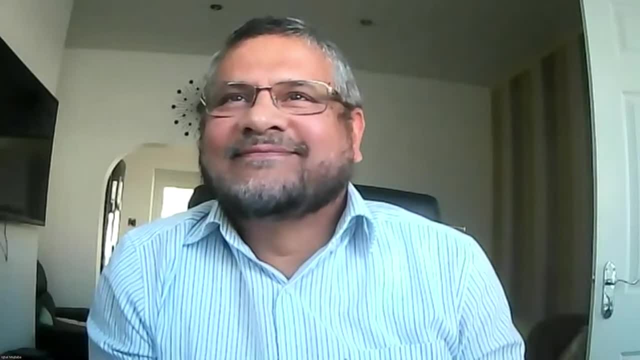 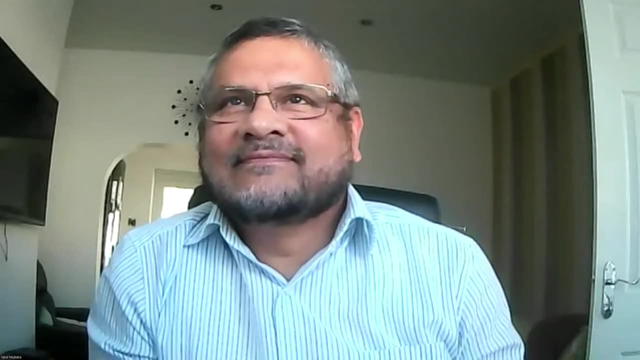 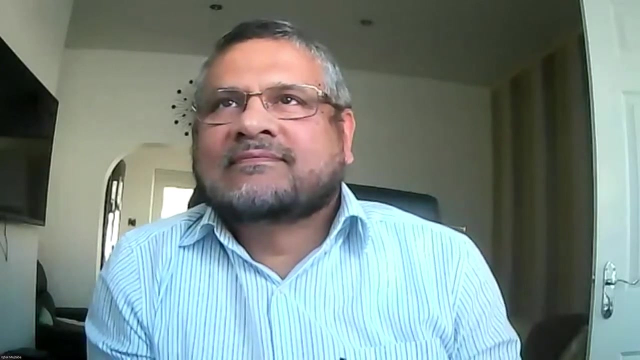 They call in at 4 in the morning at Beijing time to work with a design group at 4 in the afternoon at Penn. You can do that, So I think it does make it possible now to have multiple design projects. Okay, It's much more easy to have multiple design projects in a course. 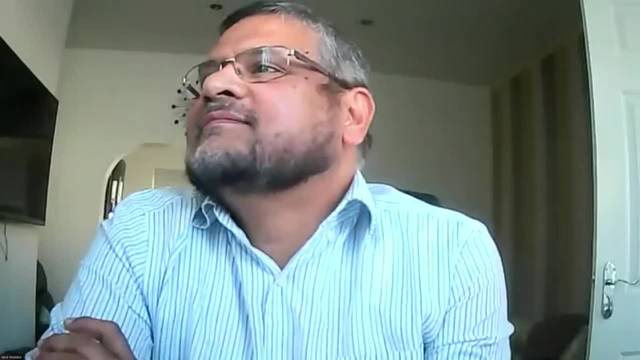 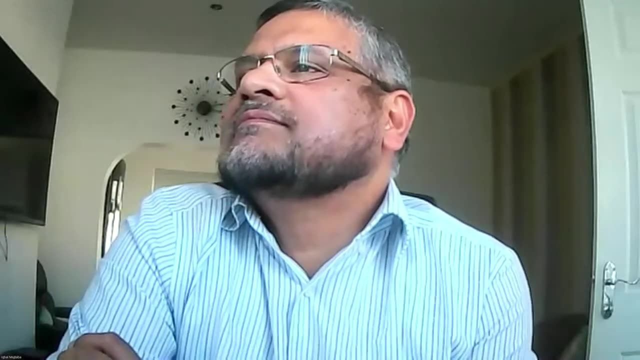 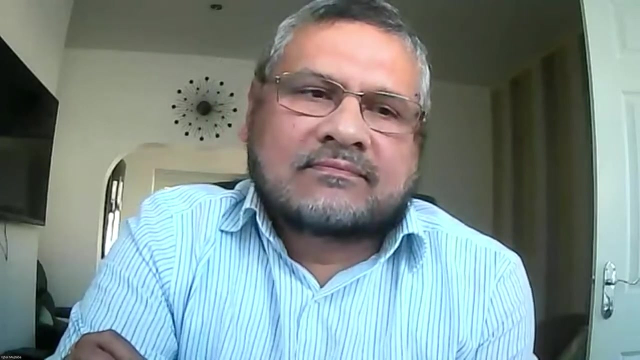 Thank you. Thank you, And I'd like just to add one comment: So long as there is one faculty member per project that is assigned to make sure that there is reasonable grading across the projects. If all the students are working on different projects, there has to be some common basis to give students grades. 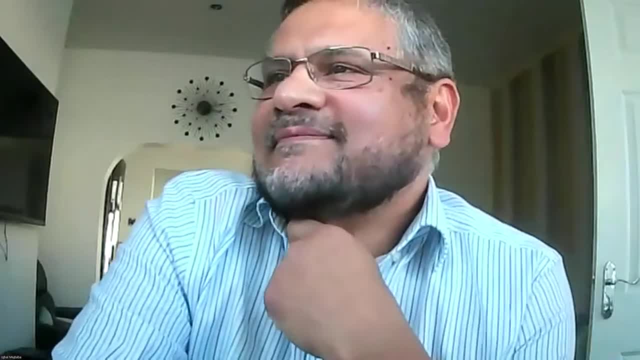 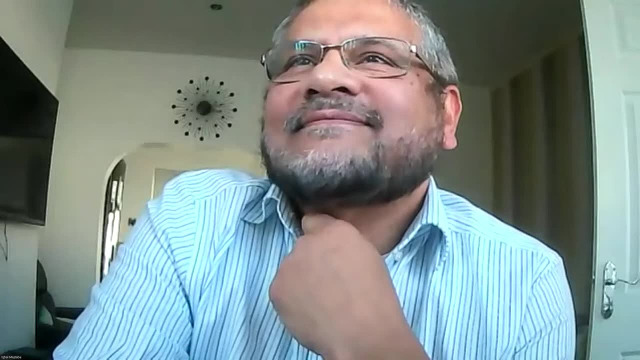 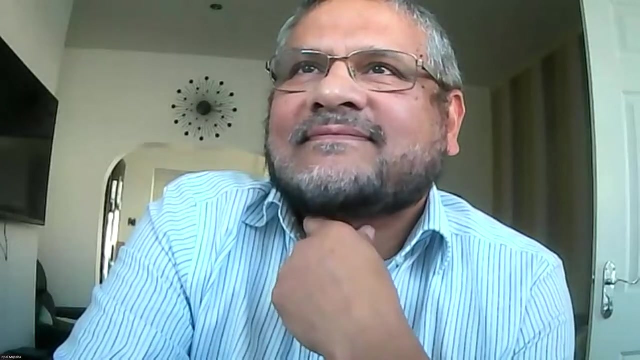 Okay, We have the following: Danny, We have an adjunct professor. You already explained the system, But not every university has the luxury of, you know, harnessing the entire faculty in favor of such a venture. At the Techno, we do not have this luxury. 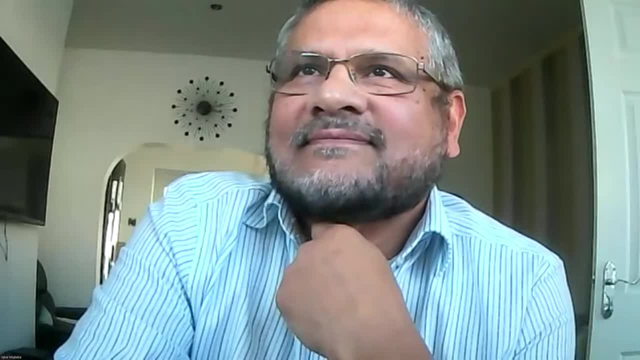 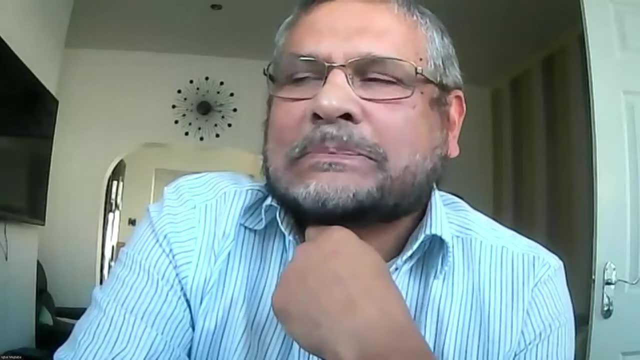 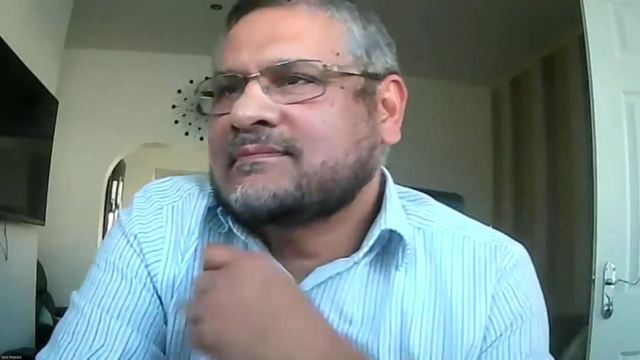 And I think that if you have one teacher handling the entire class of between 50 and 100 students, it is not practical to give individual projects. It's just going to be totally beyond the capability of one faculty member to reasonably grade Reliably all these projects. 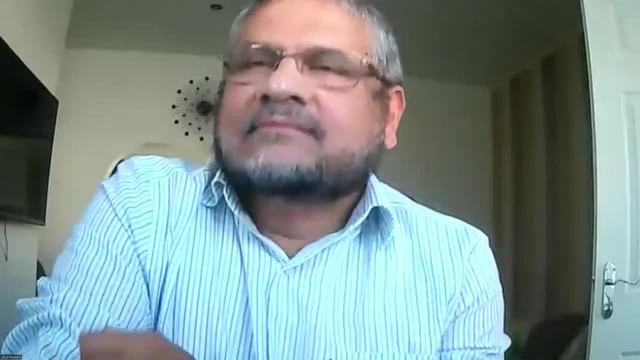 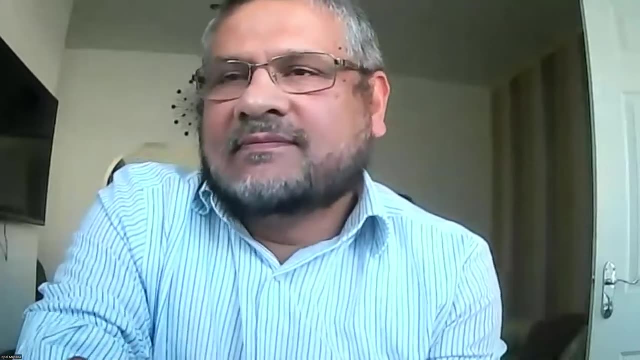 That is the reason why we do things differently, And I guess that would be the difference between Bradford and Hull right Iqbal, In Bradford, I'm sure you're not on your own with this right. You have a number of faculty members. 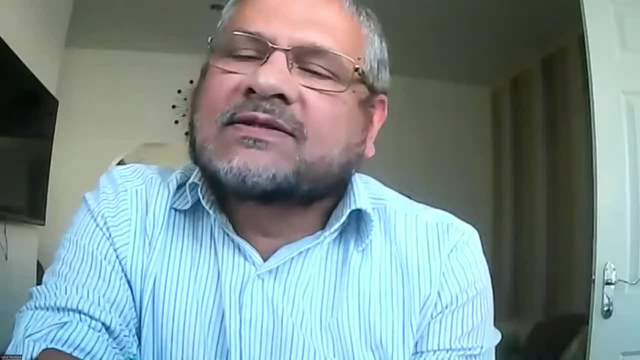 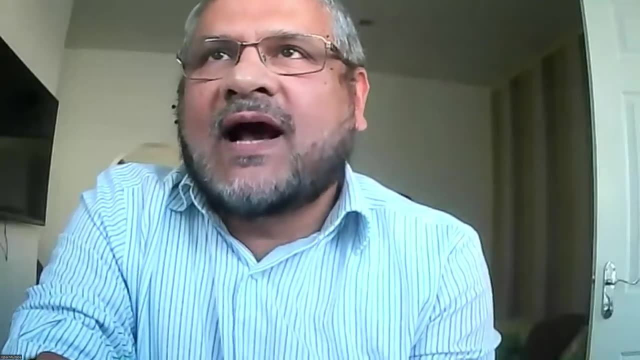 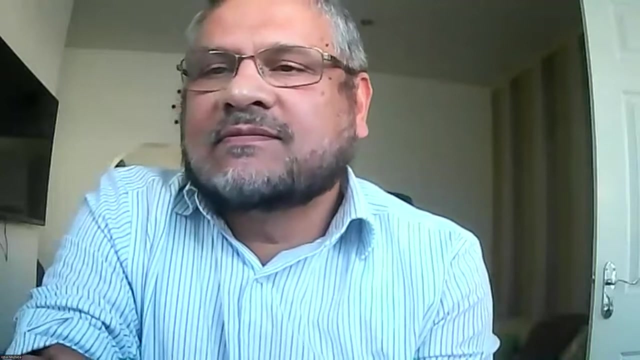 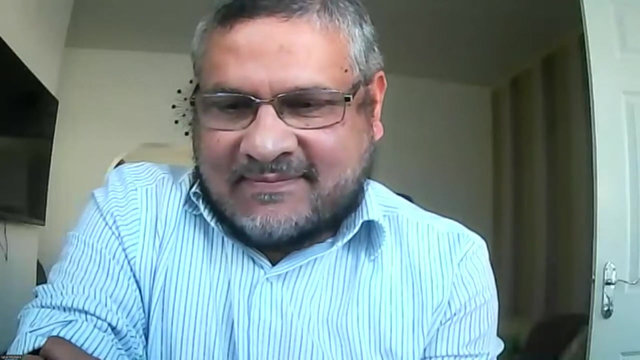 Yes, At Bradford our take is that all members in the core chemical engineering team has to supervise a design project At Hull. you are right. There's only one or two colleagues who actually take care of it. Here I will add one of my experiences when I was teaching. 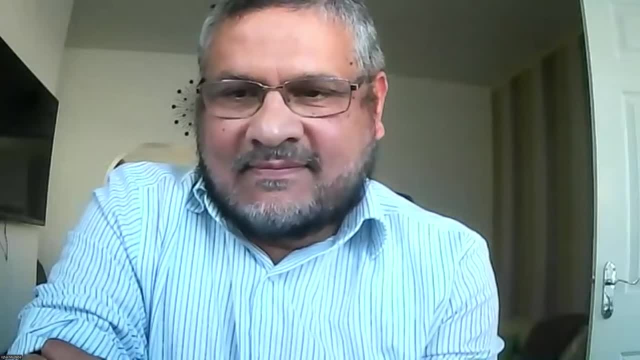 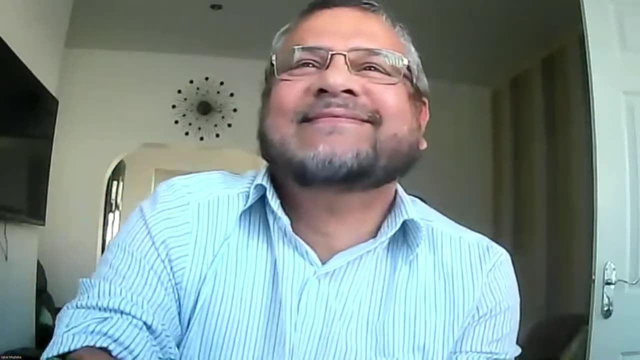 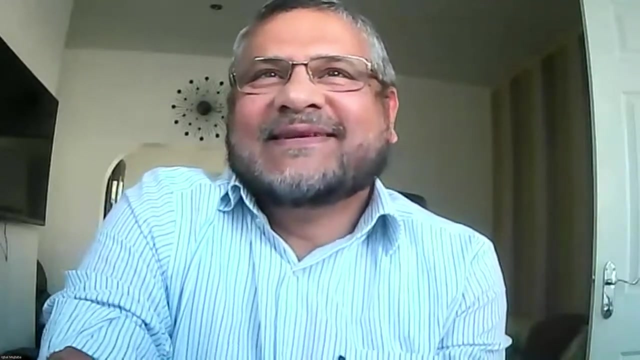 So one year, despite the objections of the teaching assistants, I said we will allow the students to choose their projects themselves And there were 20 groups. Wow, They're different projects And these were all very, very fancy things that they would like to make. 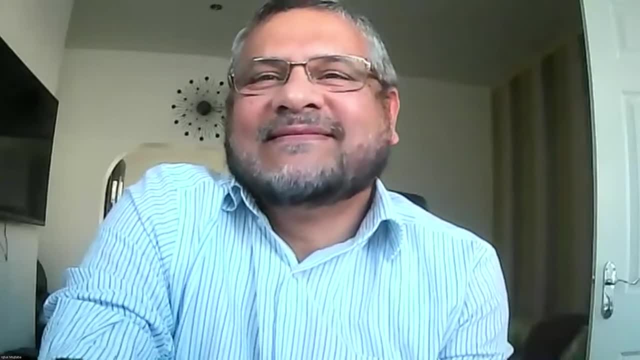 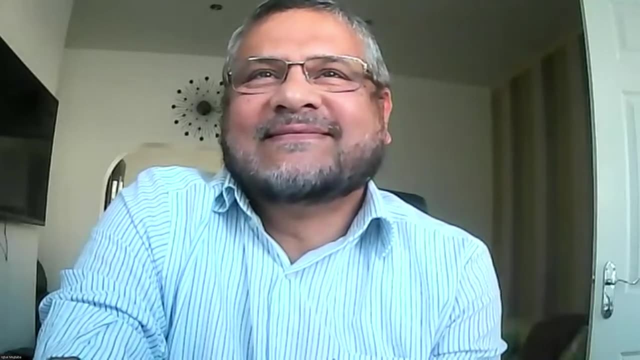 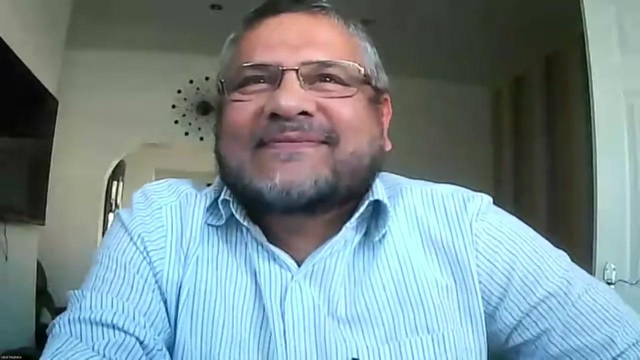 And then, once I introduced them to the simulators and the chemicals that are found in the simulators, they came quietly to me and said: can we change our project? Because once they found out what to do with the chemicals that are not in the simulator and all the extra work that they have to do, 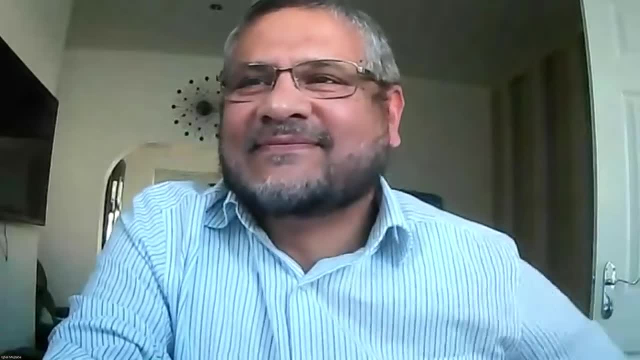 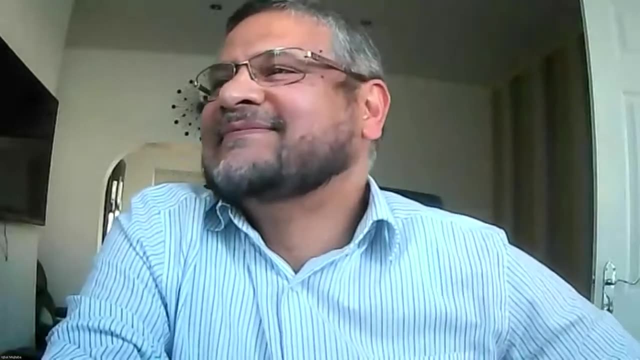 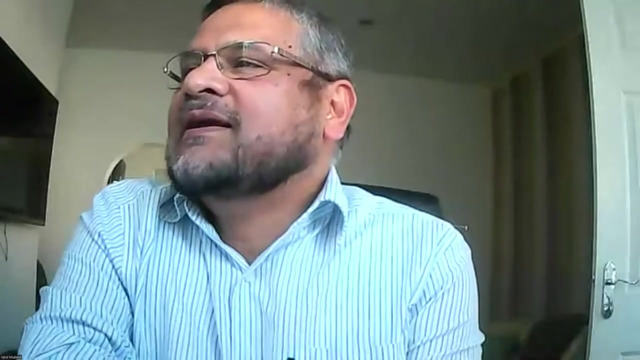 and the models of the unit operations that are not there. they all changed to the same old commodity, chemicals, to make. Thank you for the contribution. Let us move to the next one, which came from Denmark. Said Mansouri Said: if you are around, can you please just explain your question? 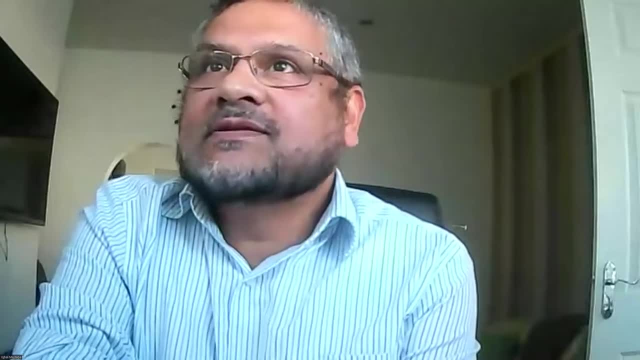 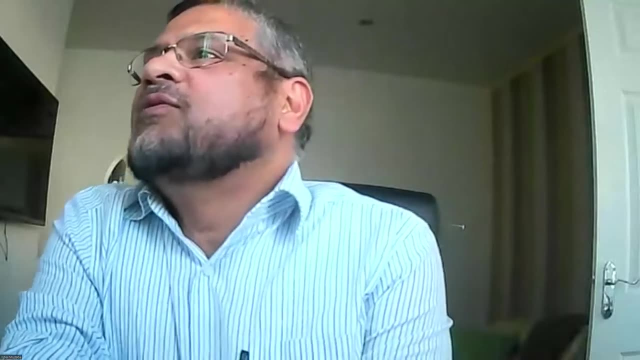 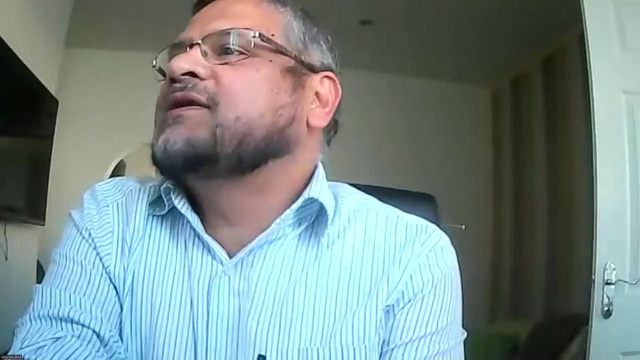 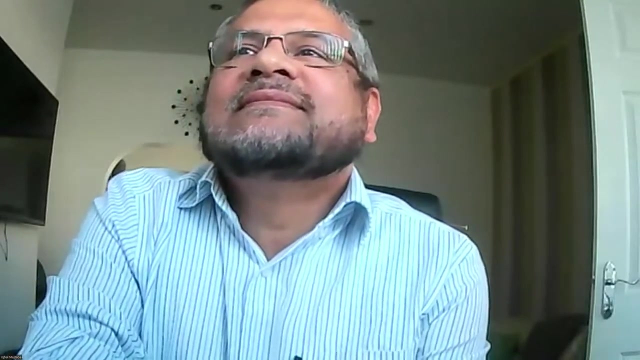 I think I did not get it quite right- Said: are you there, Right? Okay, So the question is: how would be setting in combined programs where, for example, students take part of their education with the industry? Maybe we can leave it in case someone comes back. 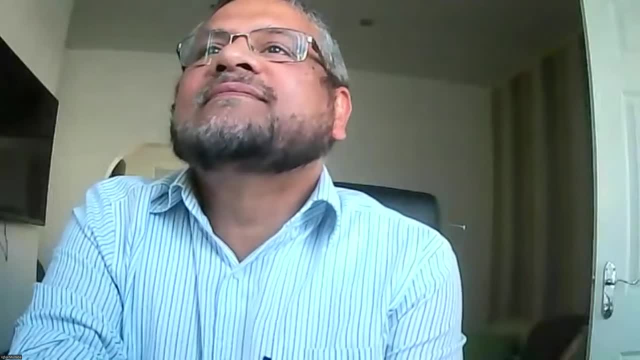 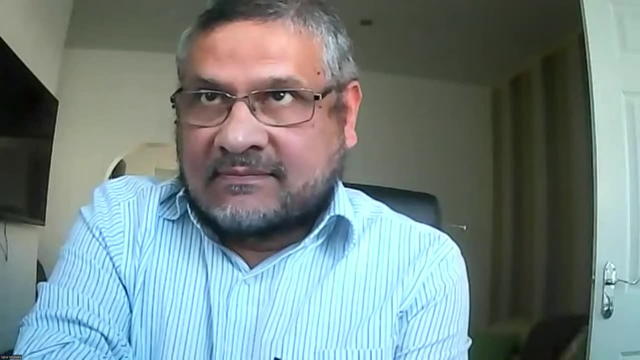 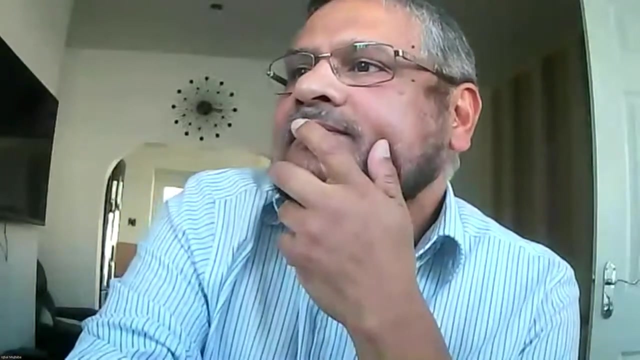 Okay, Go on. No, no, My experience in this is different. My experience in this is very limited because very few of our students are working with industry in a way that would make them capable of taking on a design project of the scale that we require in our faculty. 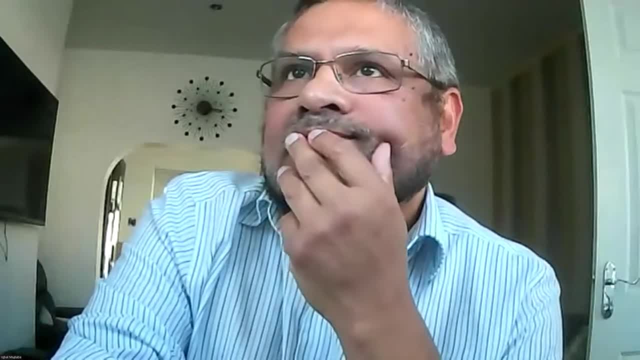 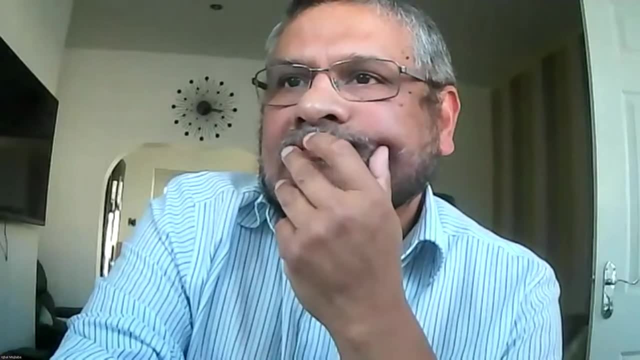 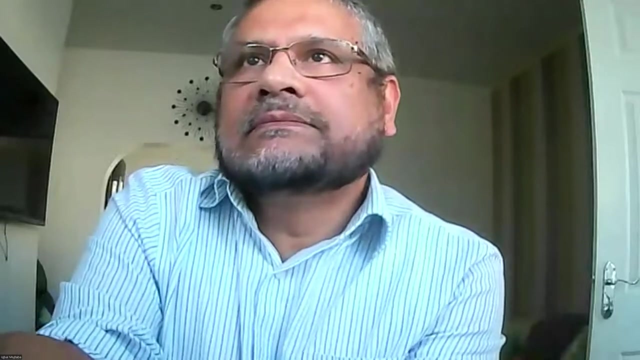 In principle, there's no problem with that. Again, once you start allowing students to do different projects, you have to make sure that you have staff available to support them reasonably. And that's going to be the bottleneck, I think, Not so much what students are capable of doing or not, but whether you have the people in place to manage such a project, such sets of projects. 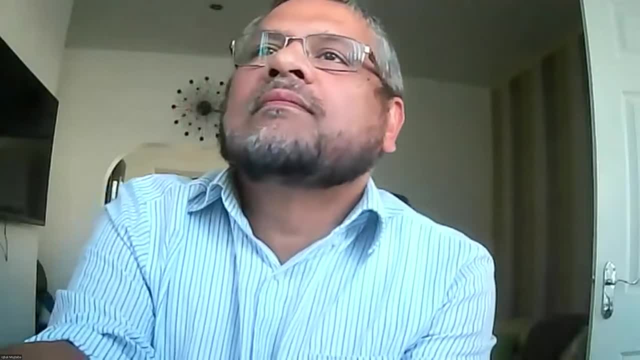 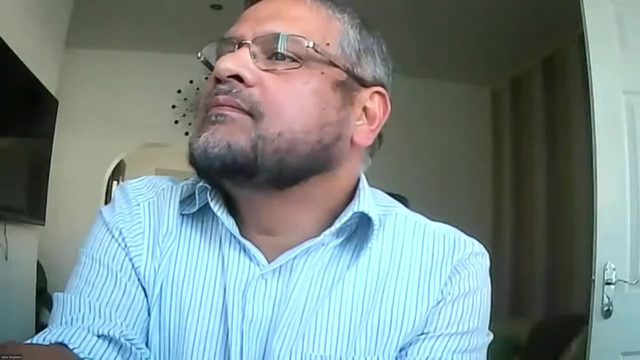 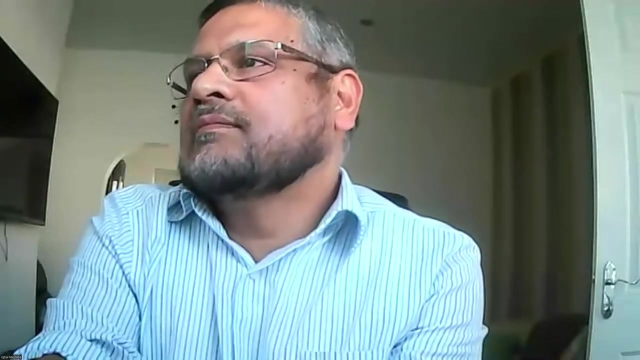 Warren's university is handling this extremely well over a long period of time, but that's because that's the way things work there. It doesn't work that way in every place. Maybe a side comment to add there to what Danny was saying. One thing is the ability to provide quality advice to the students. 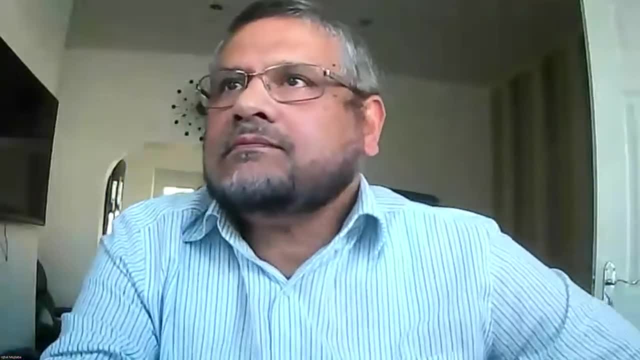 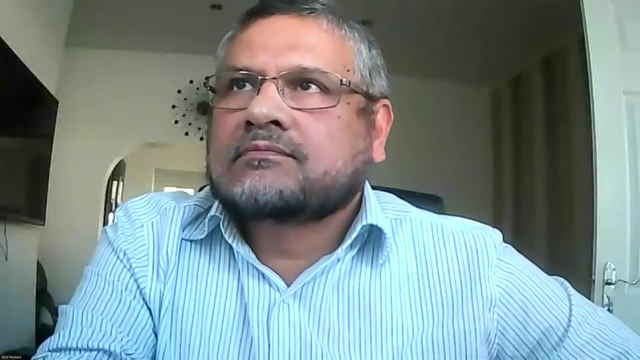 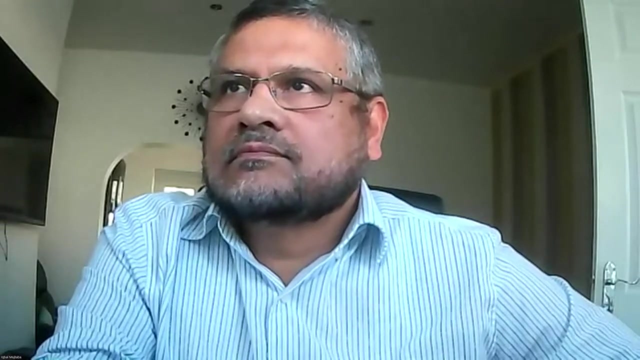 The other one is to have consistent grading and assessment of the work, which is important from an accreditation standpoint, but also in terms of fairness and equity for all the students involved. For example, one of the things that can happen is, from an academic standpoint, we may focus more on plant-wide design or land-wide design. 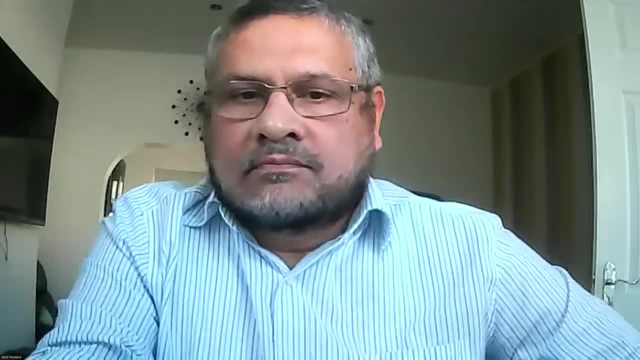 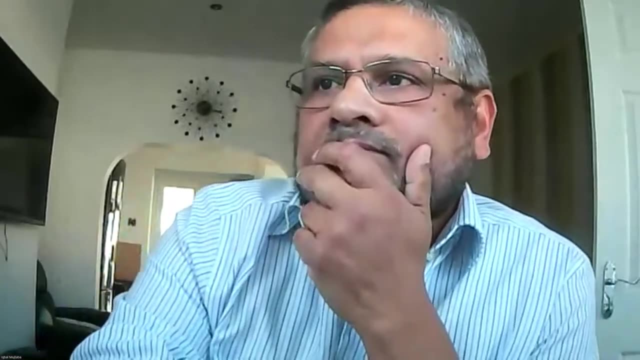 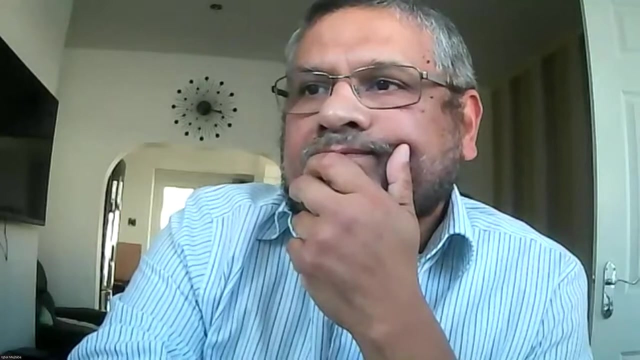 Or large-level integration, Whereas an industrial engineer may focus very, very specifically on a little bitty detail in the P&ID that we may not think is as academically interesting or what we intended for- the course outcome. So there's an issue of fairness and equity across those things. 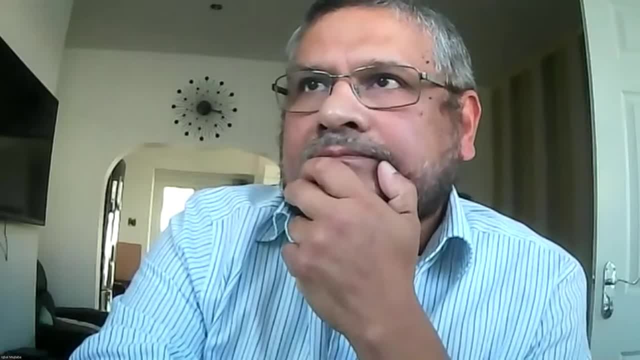 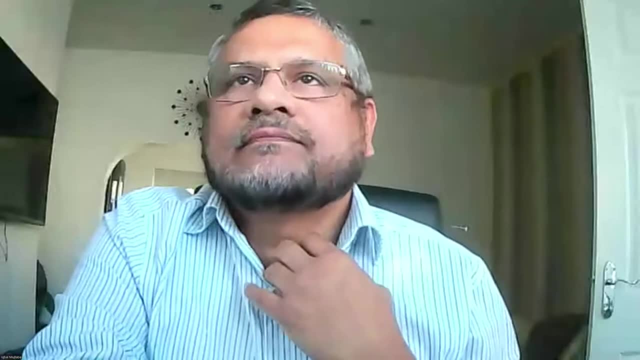 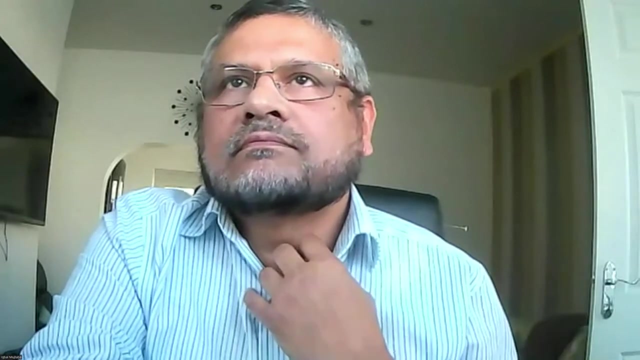 And, as Danny said, having enough bandwidth to provide the students the right support. So A quick thing: We have an adjunct professor who is in close contact with all of the people in the local industry that advise our students. They suggest the design projects. 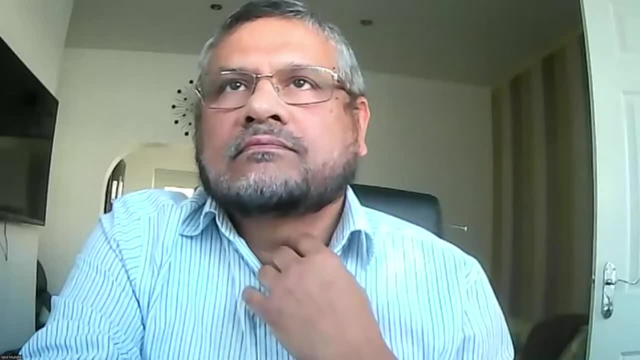 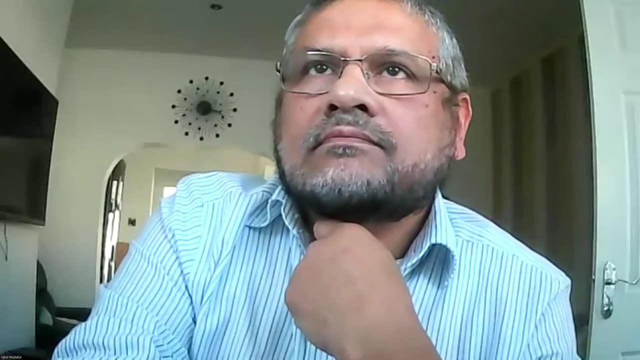 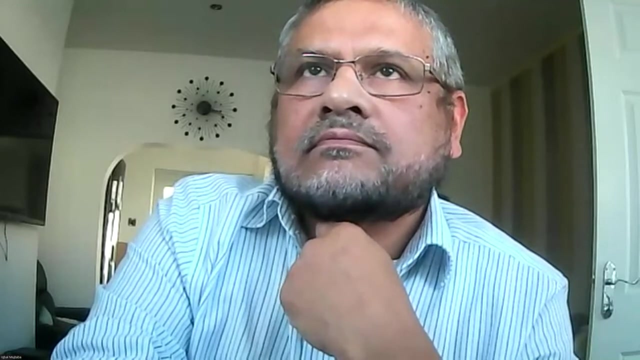 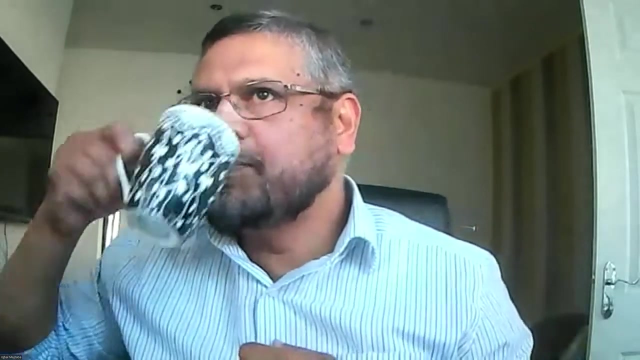 He looks them over carefully and essentially offers them as students to choose a project. Okay, We schedule in such a way that he can attend many of the design meetings And in the end, after the advisor has had a chance to read the report that they write, this adjunct professor reads every one of them. 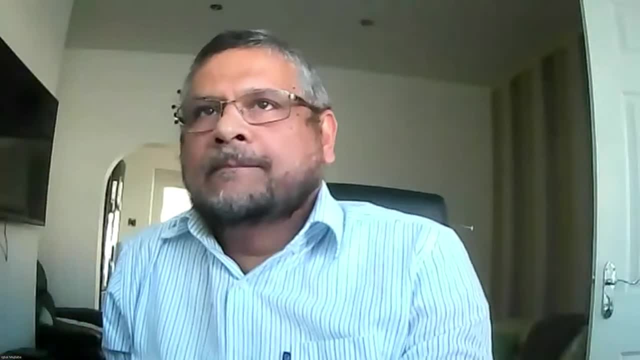 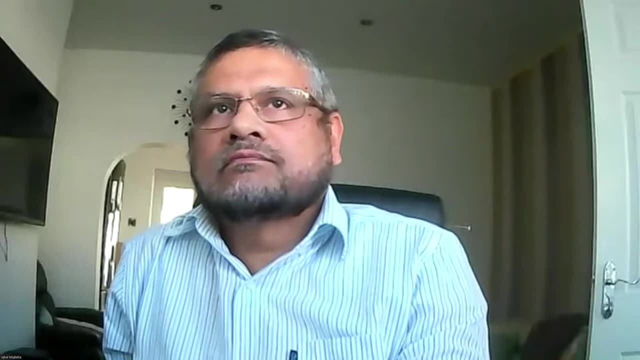 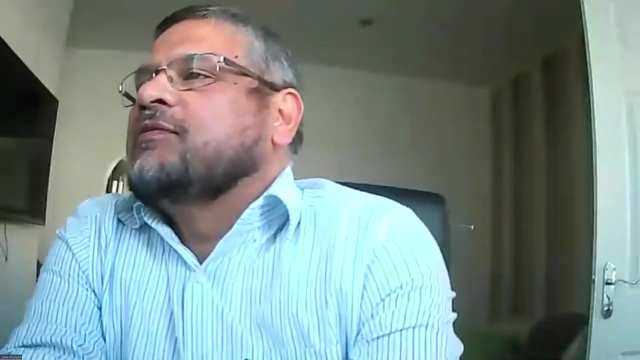 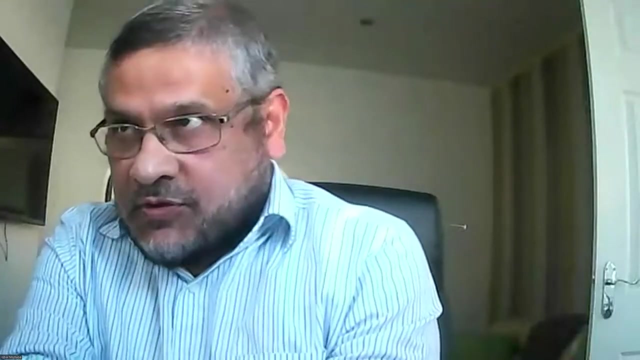 And he is the first one to assign a grade And then asks the professor who did the advising, if the professor agrees. So that's the way we do that. Thank you for the contributions From the speakers and the panel members, Right? So the last question, I think, which I will ask to the panel members and I can share my own experiences. 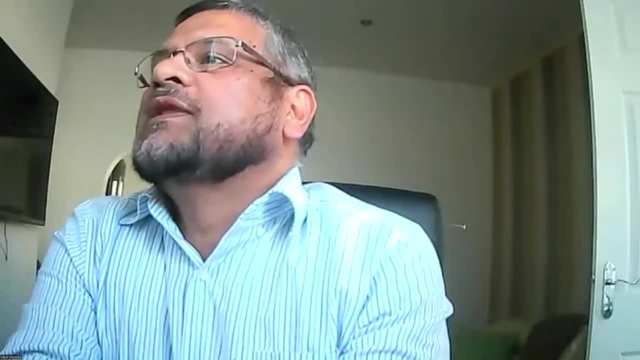 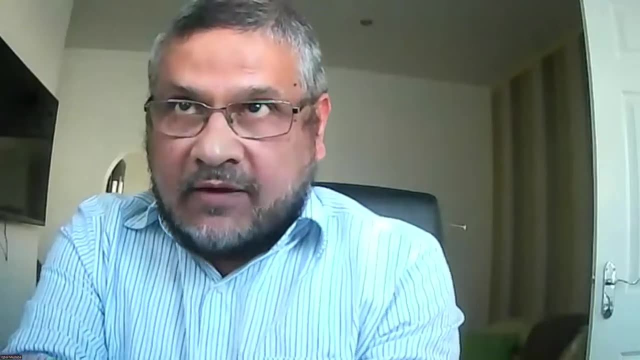 Came from Sheffield University, Mozambique- How individual student contribution is assessed in group projects, particularly in case of online projects. So you may have a group component in your design project and the students are assigned to it, And how do you assess? What are the practices? 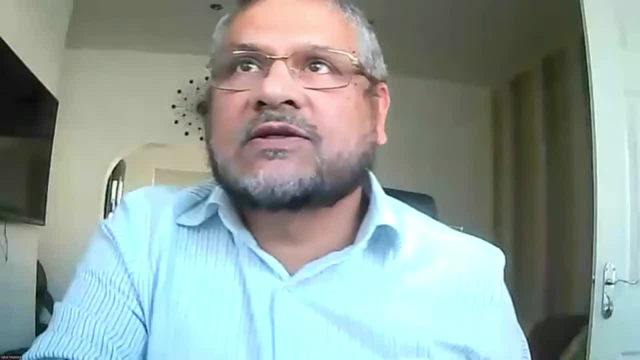 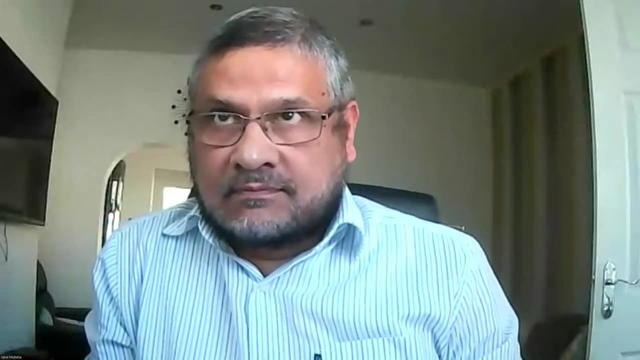 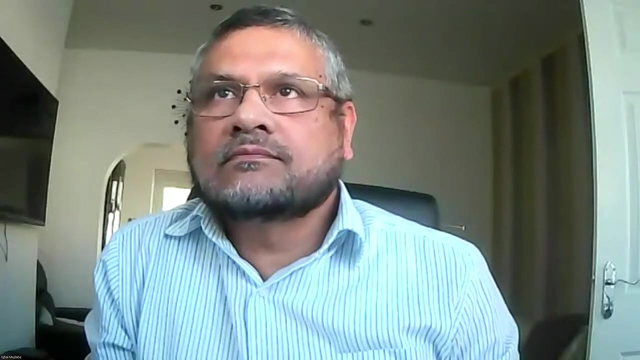 And I can share my Blackboard experience later on. That is really a tough question. In the capstone design course at the Technion, all the students get the same grade. It is their responsibility to pull weight. It happens very often that there will be some students who do not pull their weight. 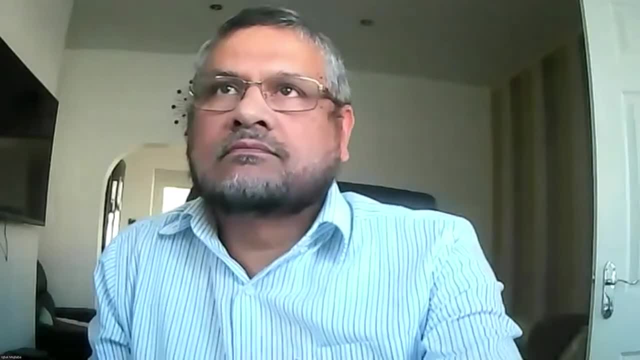 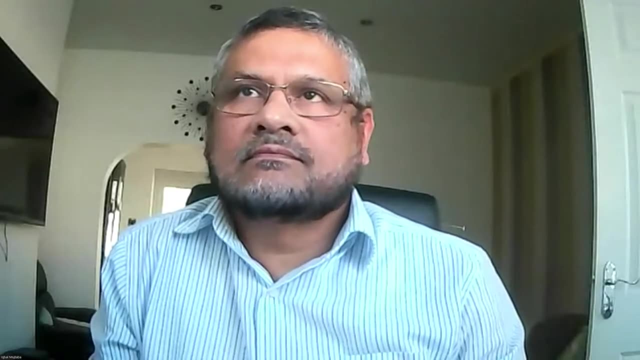 How do we know this? If we look at the grades of the projects plotted against the grades of the projects Plotted against the grade in the final exam, Typically every project grade will have a spectrum, almost the entire range of possible exam grades. 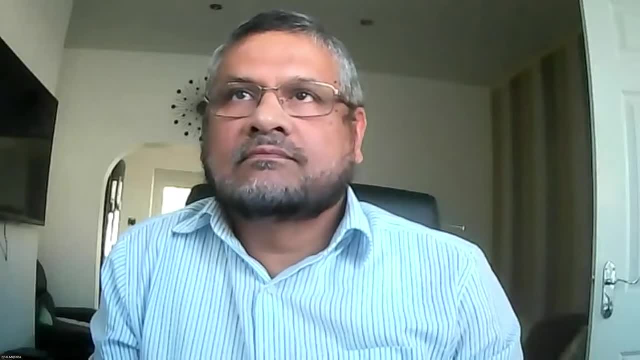 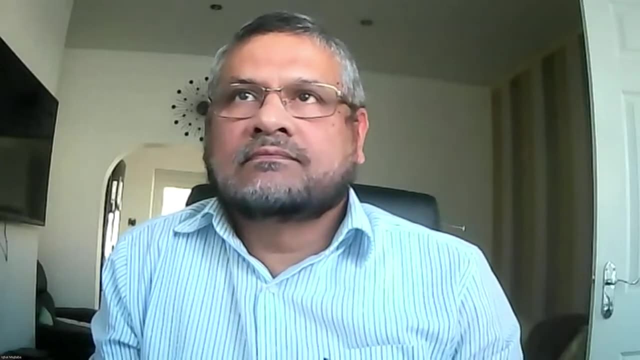 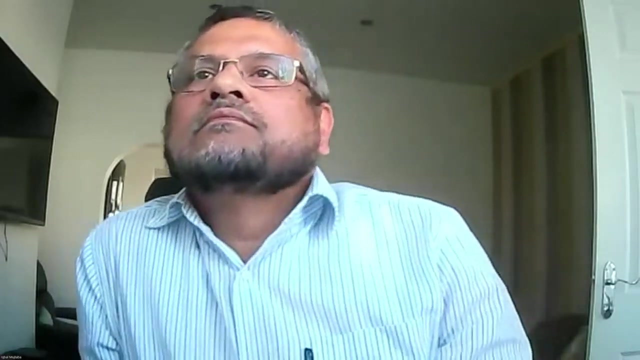 In fact there is almost no correlation between the exam grades and the project grades. That is an unfortunate result, But the bookkeeping and the support needed to make any change in this is a problem. In the plant design course I am a little bit smarter. 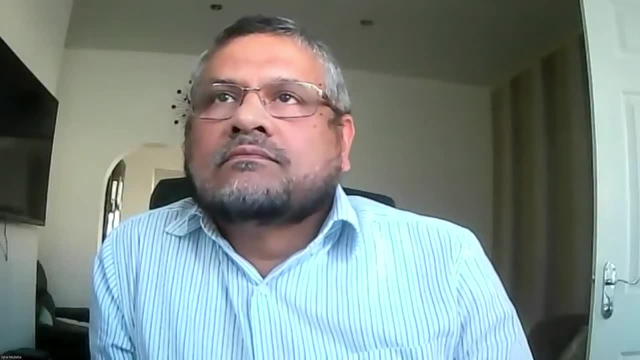 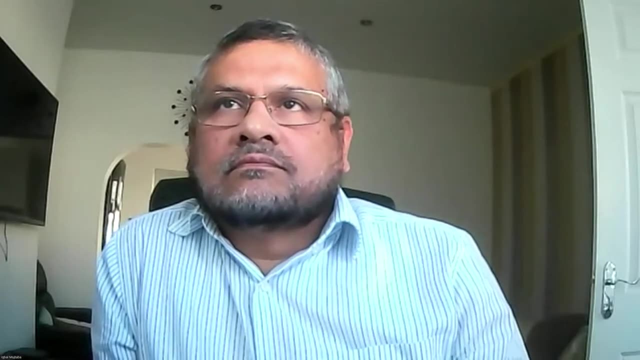 First of all, a percentage. First of all, a percentage of the grade is awarded by the students themselves. That can work partially, Although our students are very, very unlikely to give low grades, even for non-performers. But you do see this. 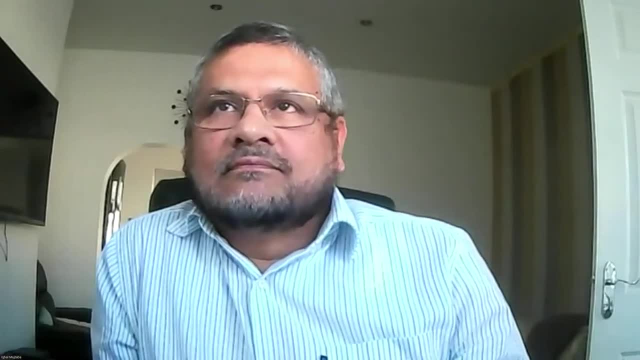 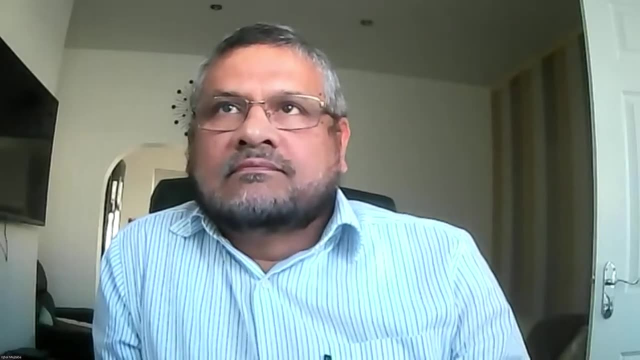 At least there is some variation. Those are internal checks within the group. To do anything else will require a lot of work. from the point of view of the course staff, It would mean repeated interviews of the entire group, Some kind of audit, Some kind of oral exam. 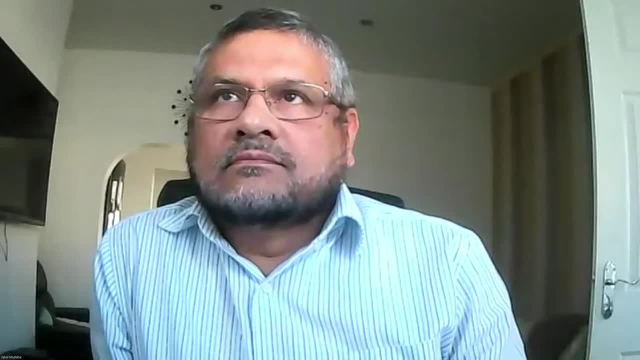 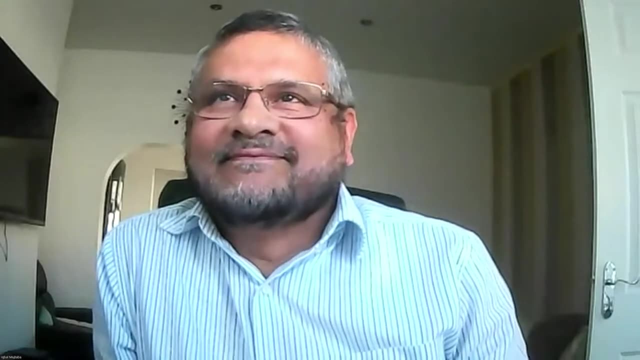 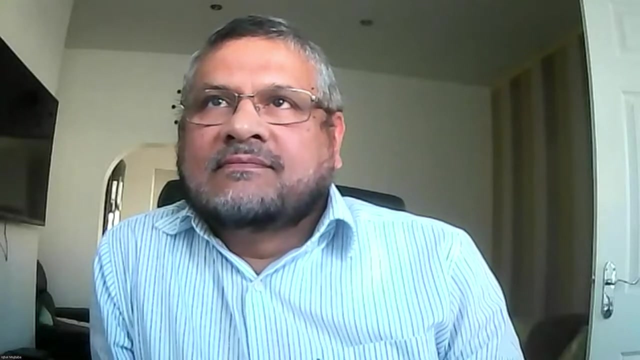 It is just the headache involved. We used to do this. The headache involved in this is very, very large, especially if you have a large number of students, But it is a problem for sure. One way to resolve this problem in some ways is that if a student fails the exam, his exam grade is his course grade. 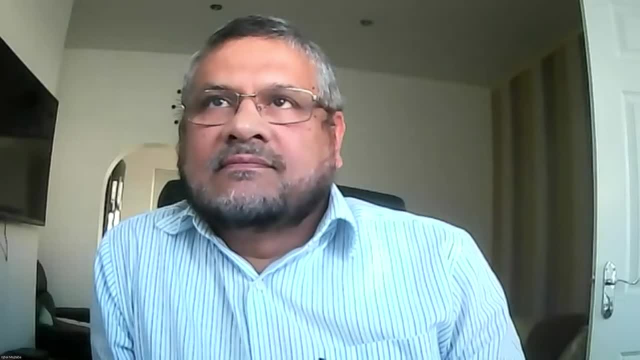 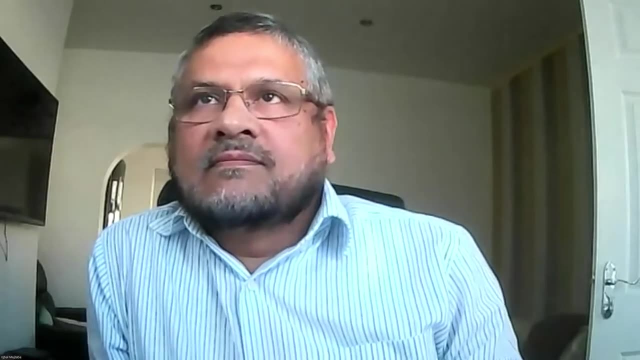 Therefore, the project grade will not count unless he passes the exam. At least he has to know enough to pass the exam. This is generally an accepted thing in all our faculty courses. Of course I am very happy to use this ruling as well. 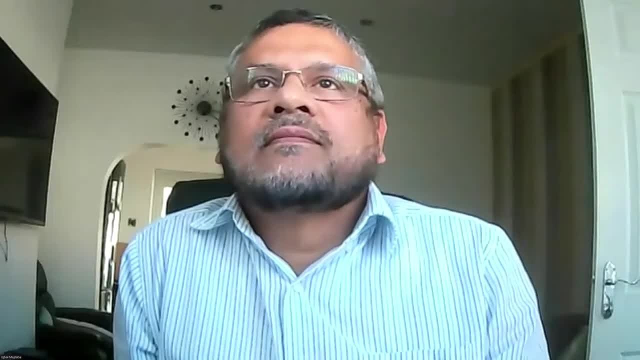 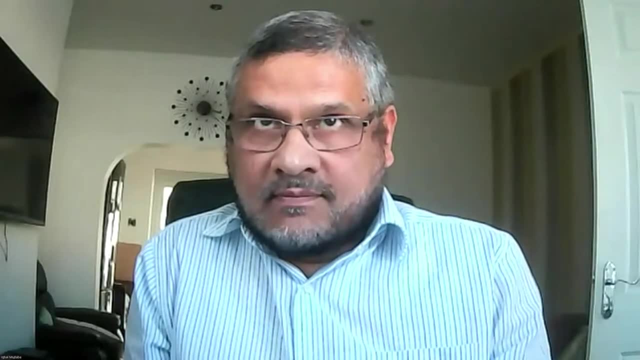 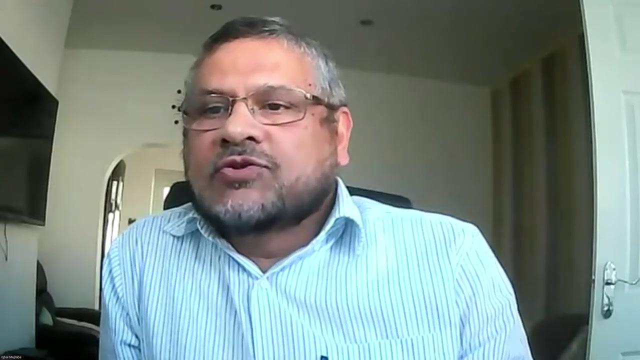 Thank you. Can we shift to Edwin now? I can see Mario has a point. You can give Mario and then Edwin can take over, if you don't mind, Iqbal, Yeah, sure, Mario is to you. But before you speak, just briefly share our experience at Bradford. 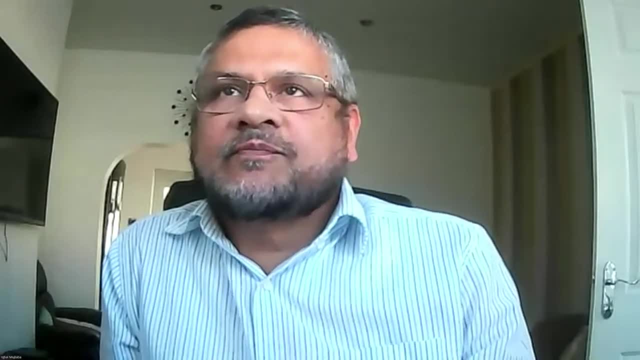 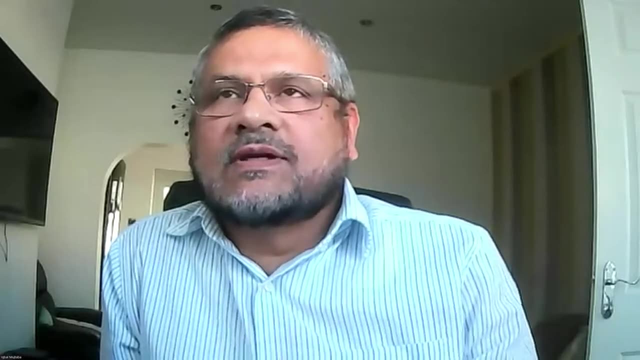 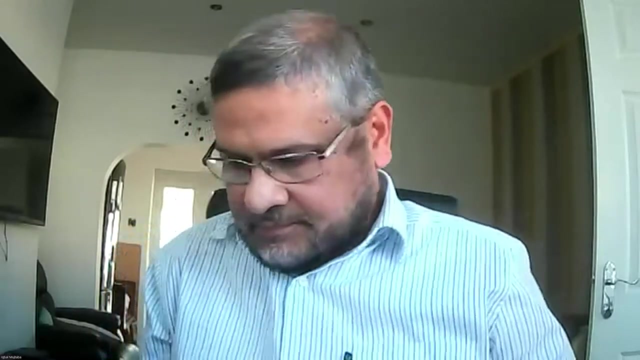 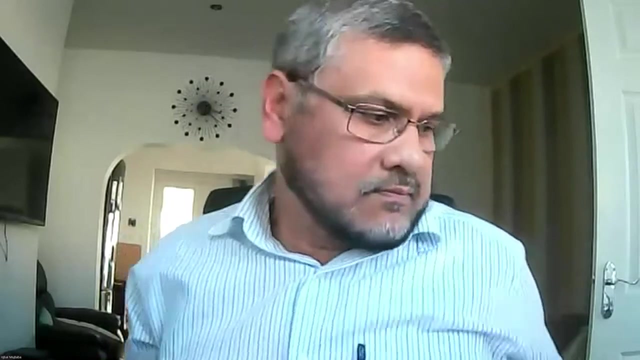 We have got to use digital peer review platform where the students peer review each other, And we have got a factor which we use to actually adjust the group projects much or assign individuals. I was just going to add: we do something similar. Even though I don't teach design anymore. I am involved because it's something I'm passionate about. 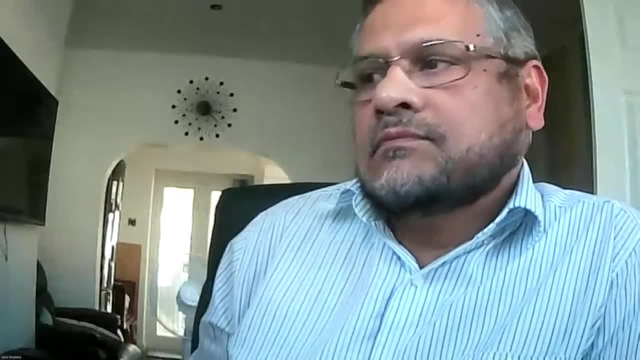 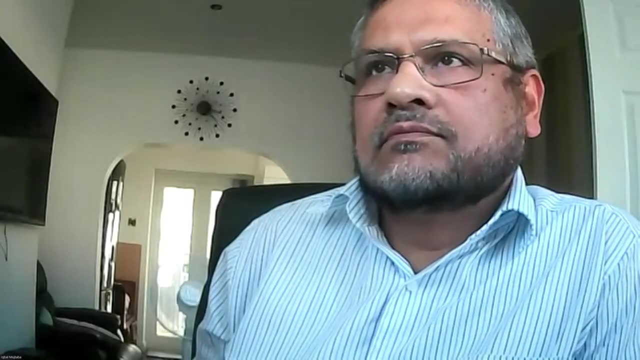 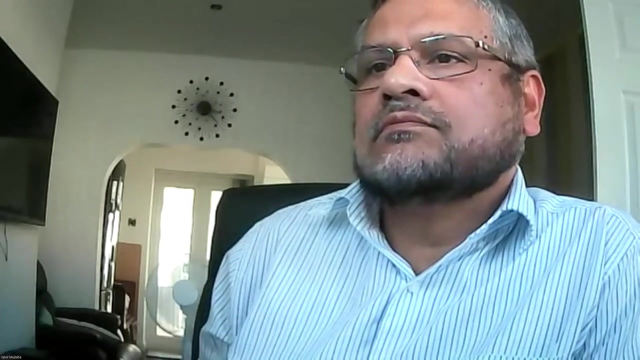 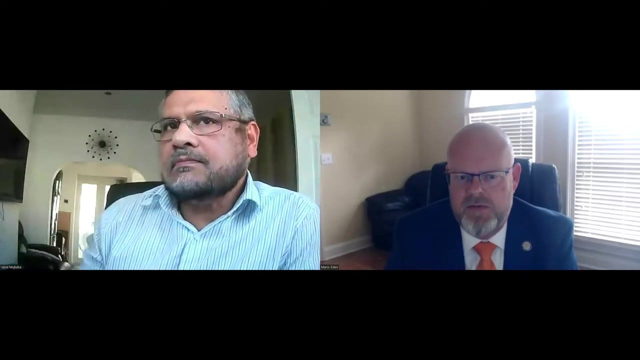 We use a combination of a digital tool that was developed at Purdue called CATME, which is a survey tool that they developed for doing internal assessment of teams, where the students do a self-assessment of their contribution along with the other team members contributions, And whenever there's discrepancy, it provides an opportunity for the instructor to have a discussion with the team. 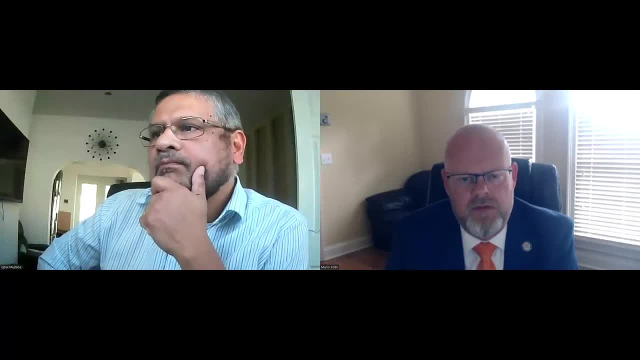 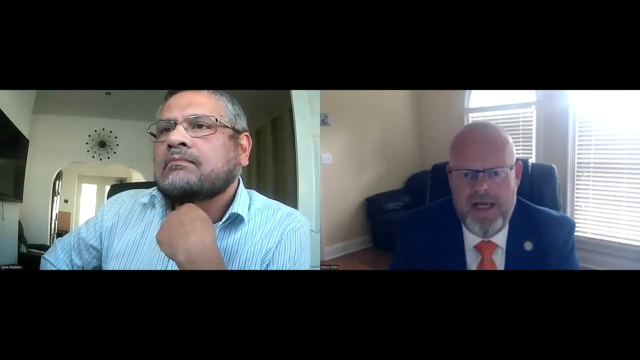 So that's proven very helpful. Another thing that we do is, on every report for the capstone class, the students will write out what areas of the report they were responsible for And very quickly, once you've taught the class once or twice, you realize and you inform the students that it's not a number of having an equal number of bullets, because we know that you know you could have one bullet. that said, I did all the simulation. 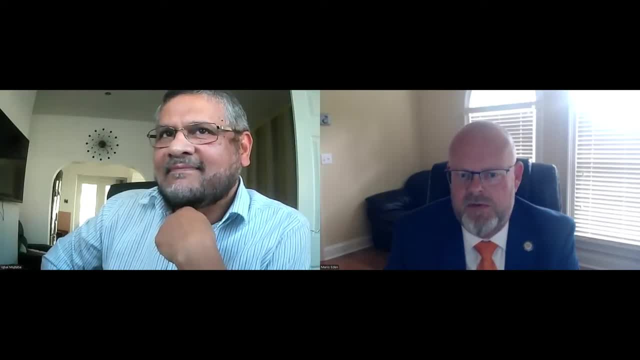 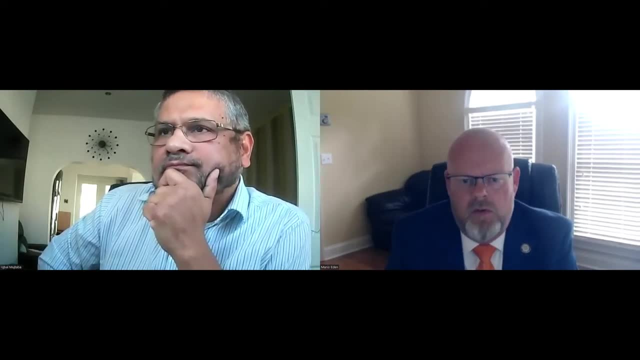 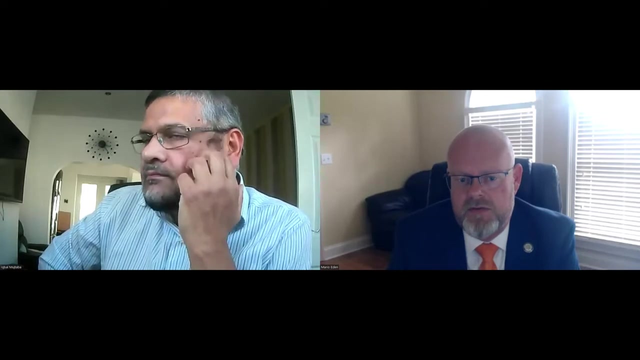 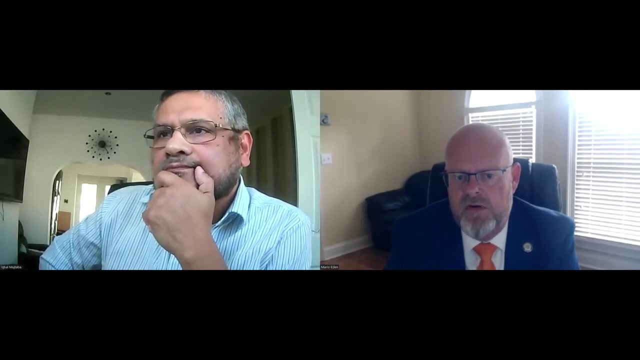 That may be a massive contribution compared to the number of bullets. That's a huge contribution compared to having been the one to write the abstract, do the proofreading format, the graphs and so on. And so when you hold those two things up together, it provides an opportunity to have discrepancy in the grades for a team, because you can point out that a certain- like Danny said- a certain portion of the grade comes from a level of contribution and equity there. 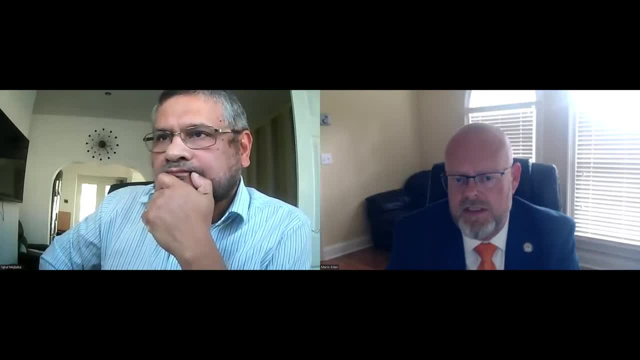 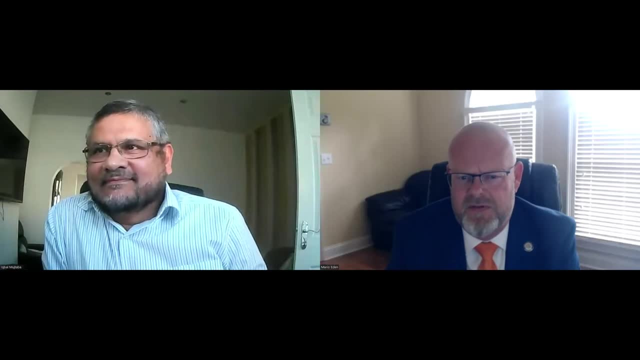 So the CATME survey has worked really well for us for at least the last 10 years And it's not that expensive, I think it's. I think you pay like it's like 150 or $200 for the year and it covers all students and it can be used across the curriculum is not tied to a single class, so that certainly something I would recommend. that's been working really well. 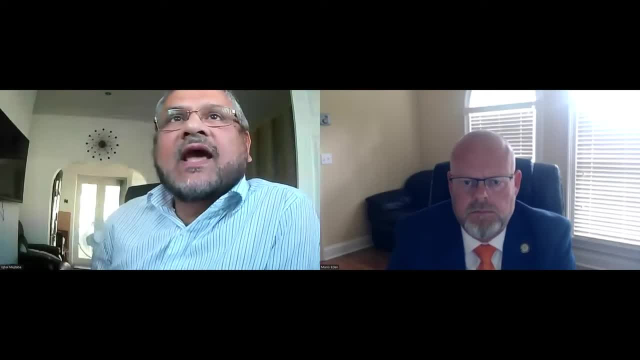 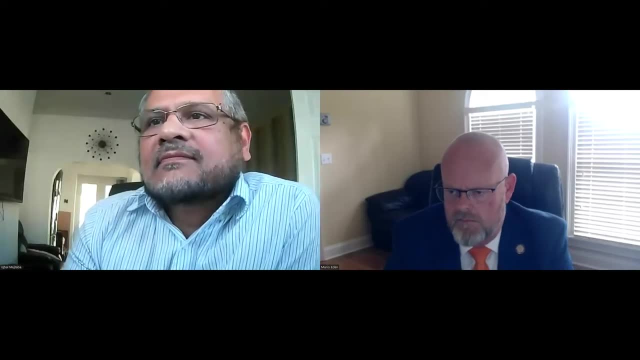 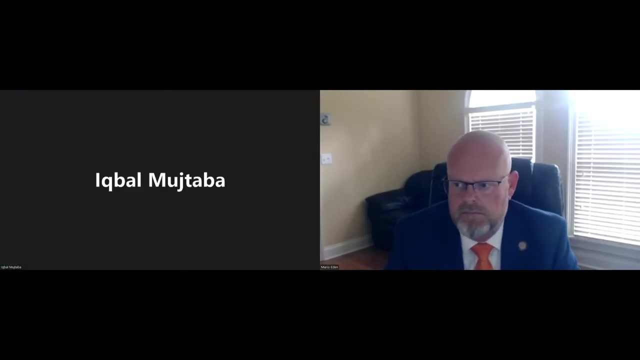 Thank you, Thank you, Thank you for the contribution, Thank you, I'll hand it over to Edwin. now for the final session. Edwin, to you, Thank you, Thank you, Yes, Yes, Thank you, Edwin. I think in this seminar we were covering the Americas up to the Asia, so maybe it should be good morning, good afternoon, good evening to all of you. 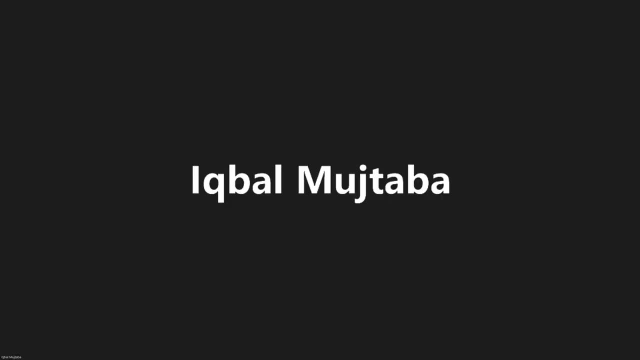 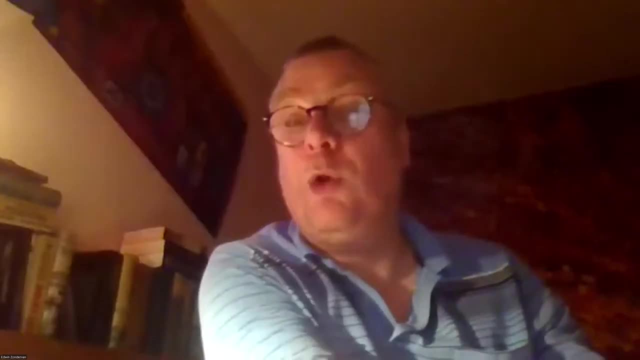 I have considered myself as the official scribe of today's seminar. Rafiq was saying: you know I have other obligations, but no, no, I prepared monologue of 45 additional minutes. No, no, I will keep very shortly in the summary. 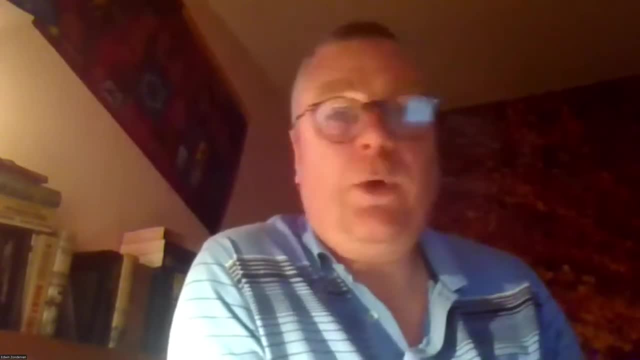 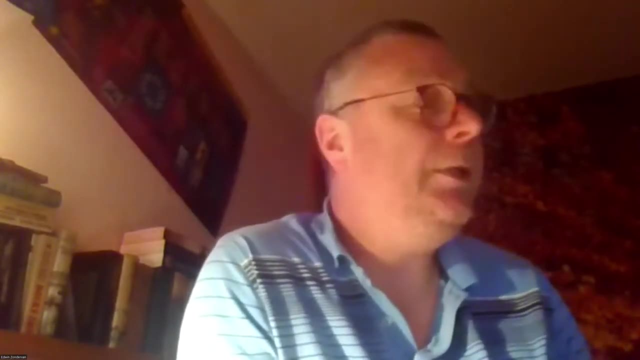 And also to put some of my personal notes. So you have been viewing in the last three hours, a seminar organized by PSC for Speed with two main speakers, and we have, of course, this panel, of which I'm also a part: Mario Eden, Igbo, Muitaba Song Lu. 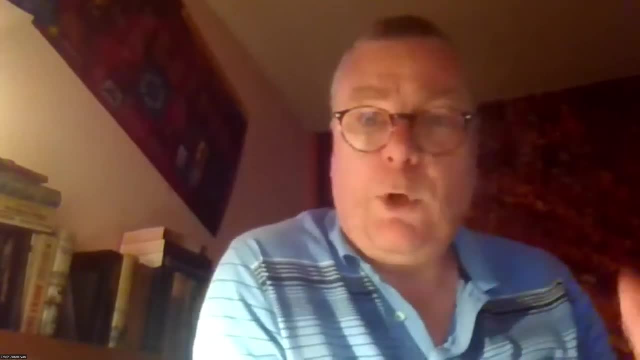 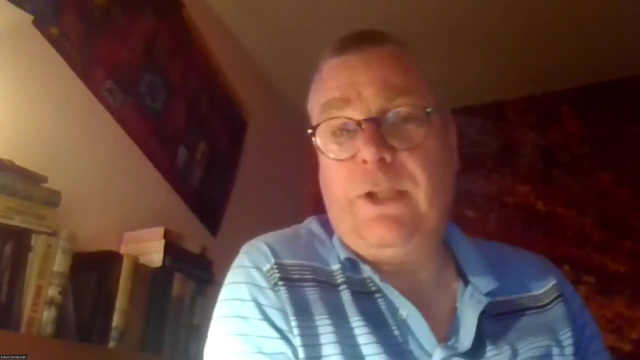 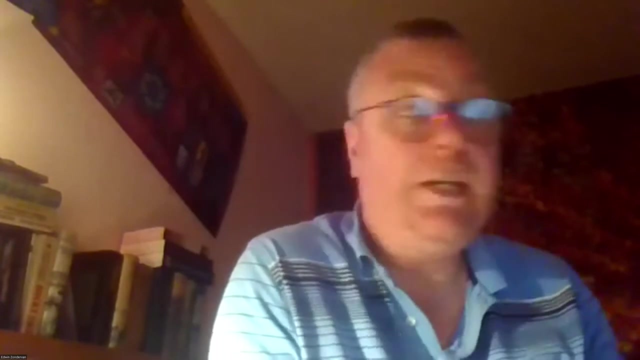 And yeah, they were up front, asked a couple of questions So to give also an impression of who we were facing today. I think we were having on average 80 to 95 participants in this meeting. Around 70% is actually involved in teaching lecturing. 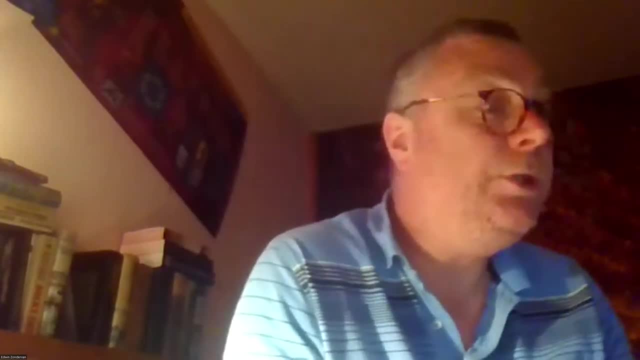 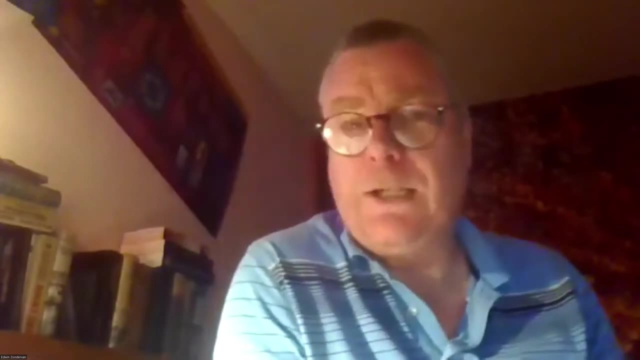 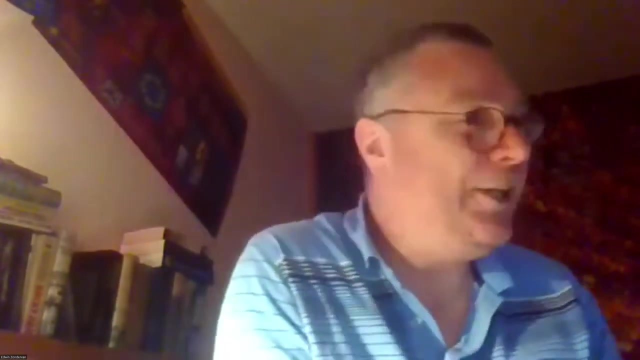 Around 25% is in the role of students and more or less 10% on the industry side. I noted here that actually not so many questions were asked from the student side in this workshop, So there is still some opportunity to post questions, especially for students. I would suggest. 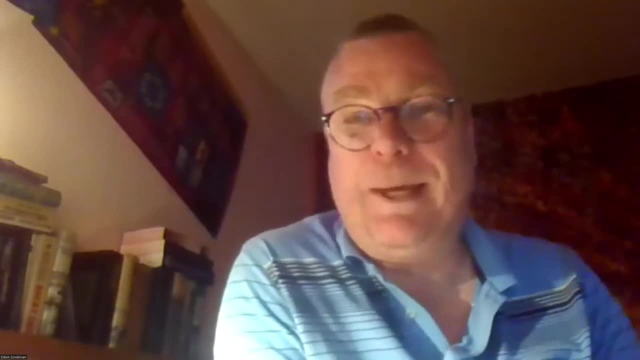 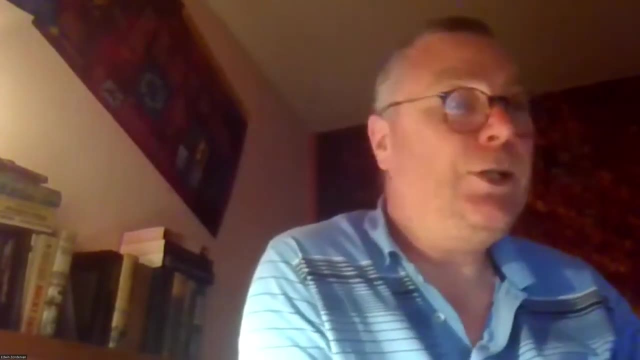 And you all, apparently, were here to learn to listen and to participate in this event, So let's see what can happen with the participation Now. we were listening to three parts. The first part was a general overview in the process design courses. 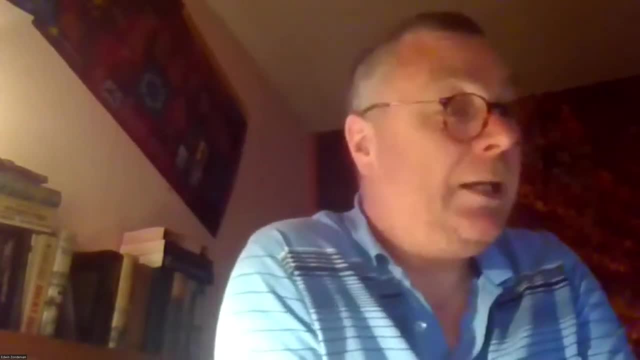 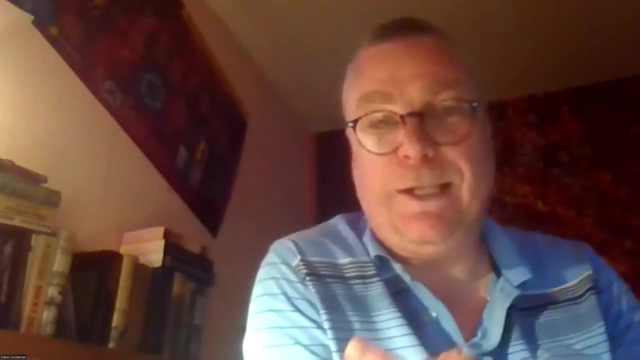 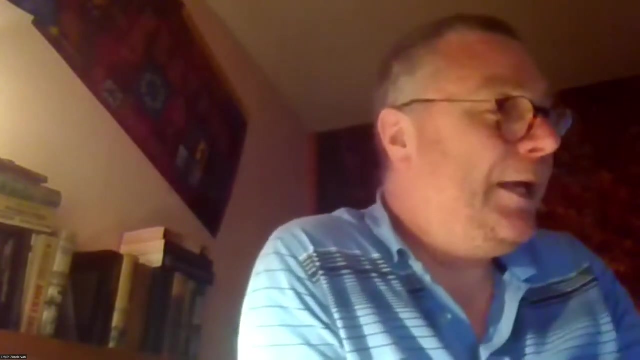 The general structure of process design at Penn and at Technion. to a certain extent, I think they were following, of course, the famous textbook. It's for me very special to see the three authors of the famous textbook here present today. There are in total, I think, five. 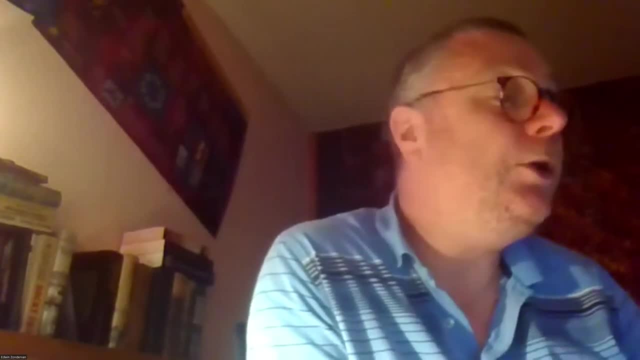 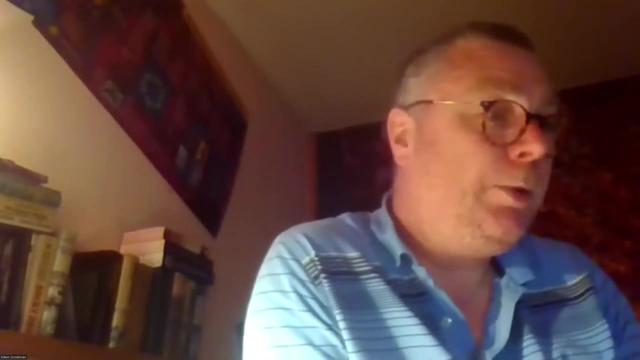 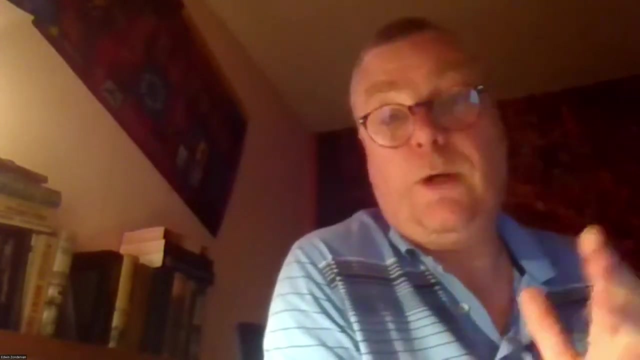 And these lectures. they include the lecturers. They included also a lot of multimedia and flip learning concepts in the lecture And they were describing the balance between traditional, new approaches with challenging case studies for the students. I noted, for example, the development of COVID vaccine, or carbon capture and then carbon into CO2, related to the current world challenges. 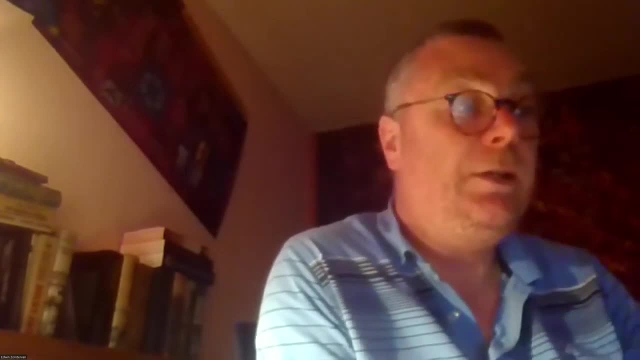 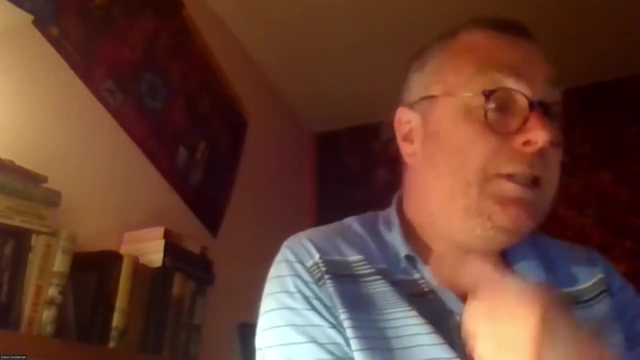 And the traditional approach is, of course, typically designed for batch or continuous: to define inputs, outputs, To do the conversion, design the separation, To design the recycles, design the heat, integration, economic analysis, safety and risk, plant-wide control. 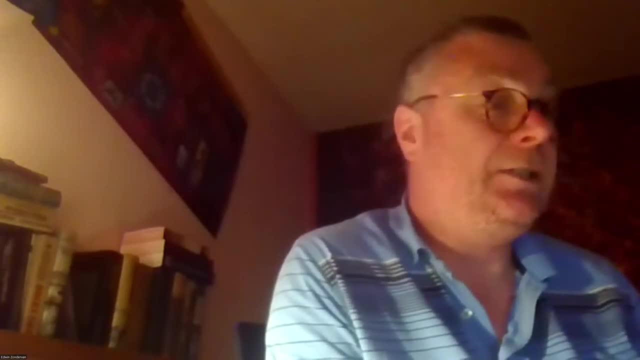 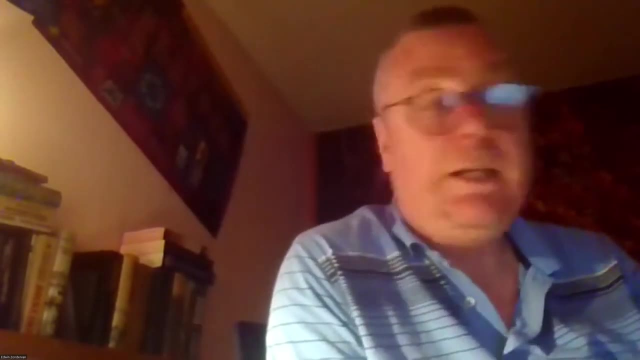 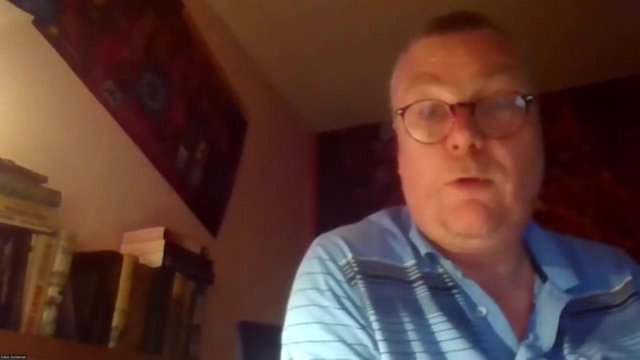 But also life cycle assessment and the use of heuristics were mentioned multiple times to limit the number of alternative designs. Daniel Lewin also mentioned something about that. future teaching goes beyond the country borders, And he was involved in a course that was actually split between Israel and China. 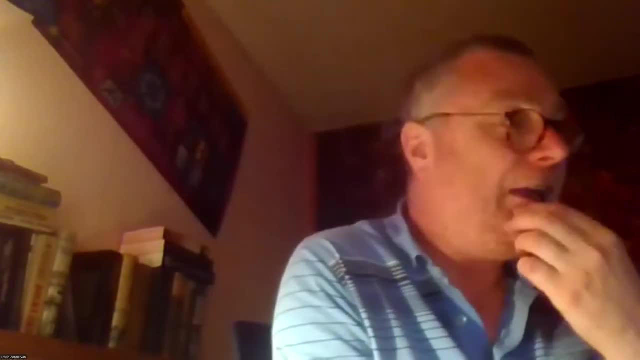 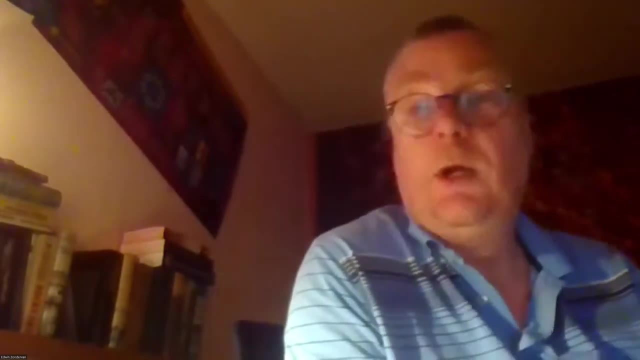 And the people communicate and form teams. Yeah, And that's what we learned by internet. We also learned about the intertwine between product and process design, For example, what to make and how to make it, Starting from the chemical supply chain. 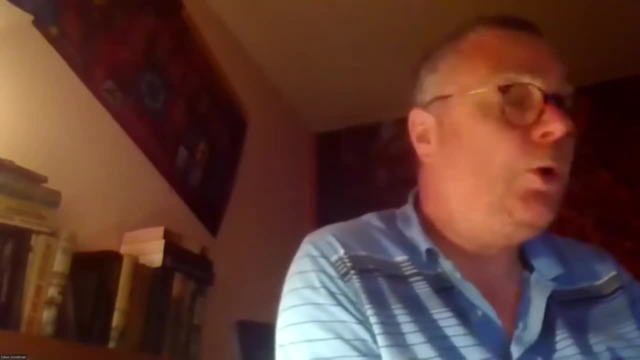 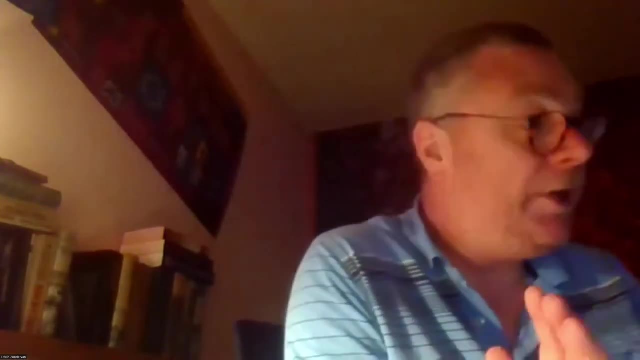 That not only the product specifications are important, or the composition, but also the functionality of the product. Then, after this first block, a couple of questions and discussion followed Very shortly. typical outline of a course: the size, the duration, the breakdown, the prerequisites. 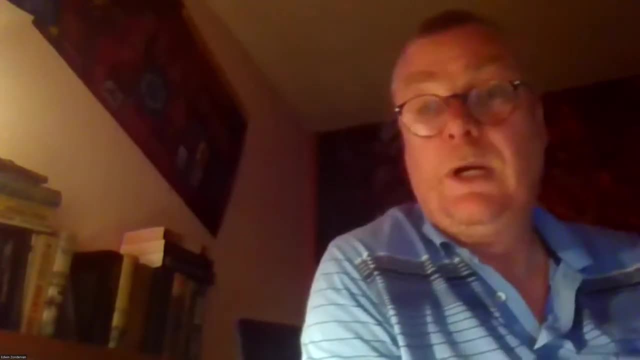 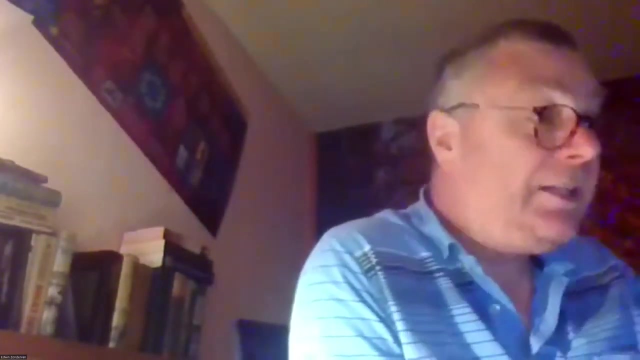 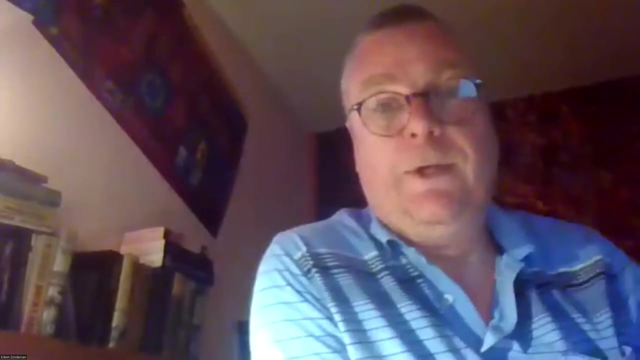 How to track progress and motivation, How to assess students, What is the role of LCA and sustainability actually within a course? What is the aspect of ethics in relation to geographic location, for example, was mentioned And I took from this part as kind of a one-liner. 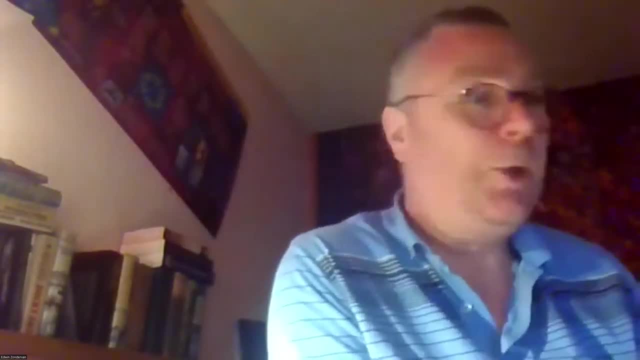 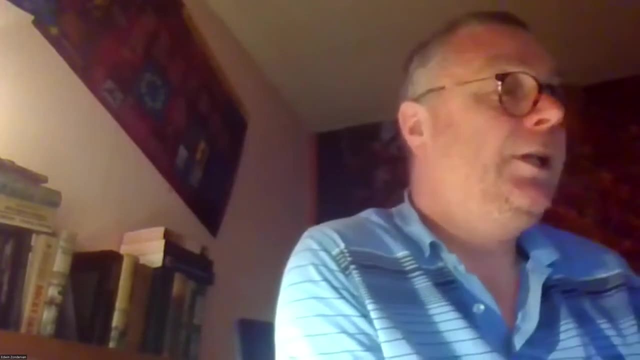 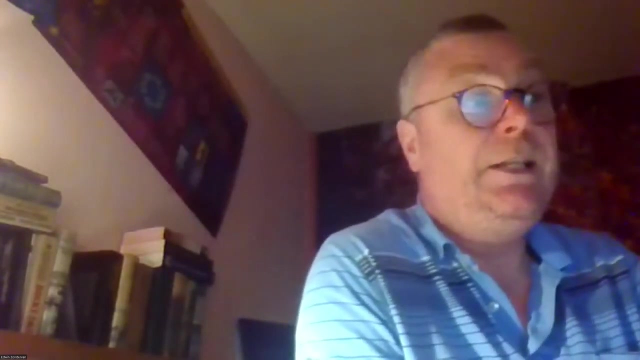 Future education is not so much toward books but much more in the direction of new resources, For example the internet. Then a second topic followed. It was simulation for process creation. And yeah, I think the process simulation here takes a leading role in the design process. 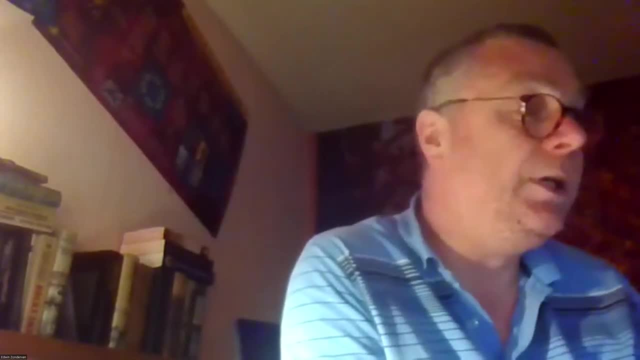 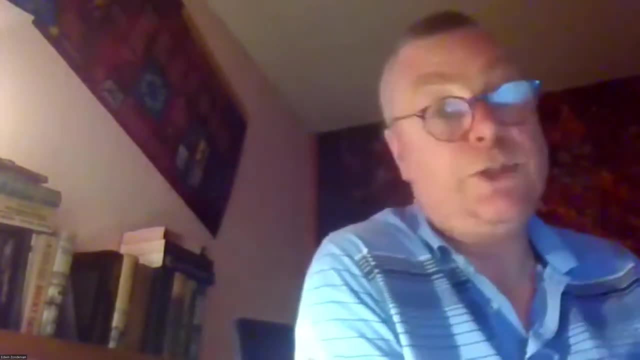 By calculation of mass energy balance, liquid sizing and costing. There was mention of different softwares. I think one of the last questions was also about what kind of software you might use. It's not always Aspen Plus. It can be SuperBroad Designer or Honeywell Unisim. 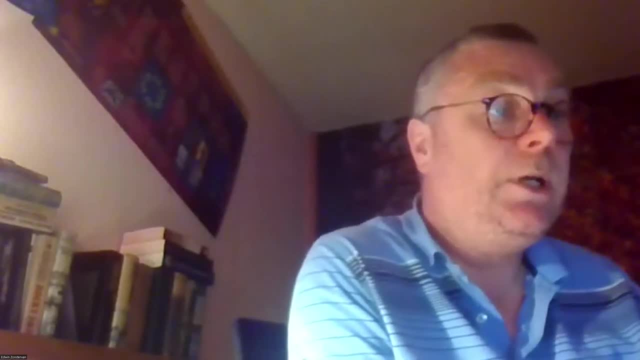 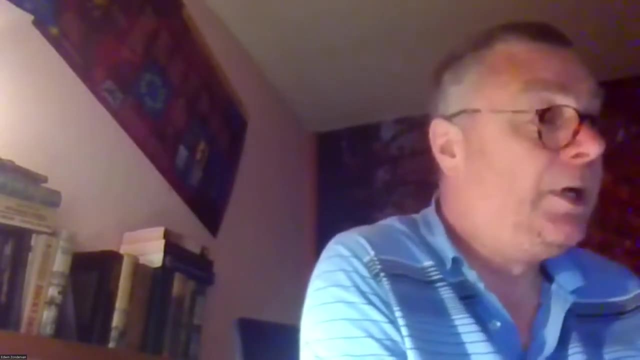 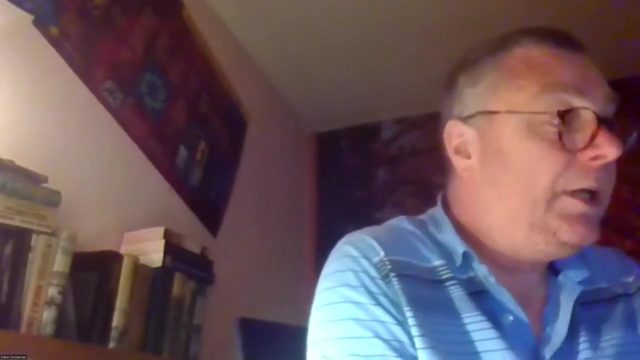 The basic features in the course in relation to process simulation are Also to understand what is the degrees of freedom concept, How to set up design specs, How to perform sensitivity analysis, How solvers work, Tier variables and tier streams, And a short demonstration followed from Warren's side. 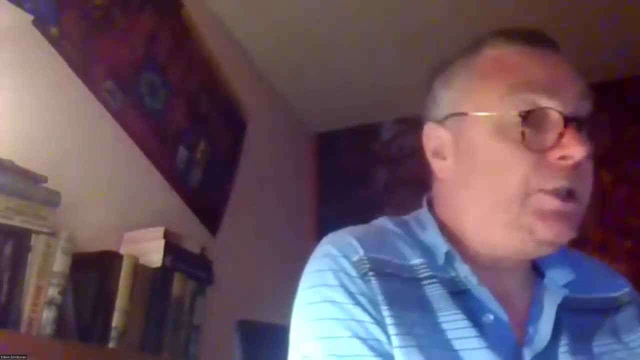 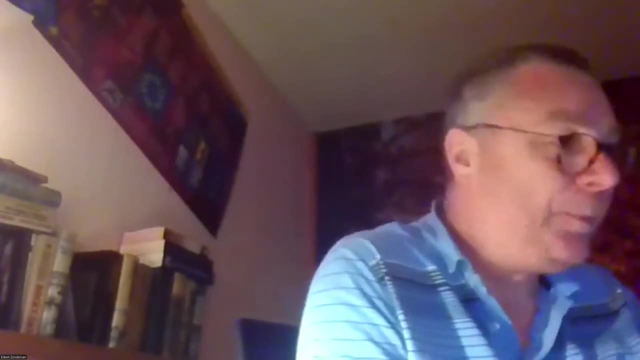 In a multimedia environment on how to set up a process simulation. in Aspen There was a very short- maybe too short- note on the aspect of batch process design and scheduling. I think it's important to understand How simulation packages can be used to sequence separations. 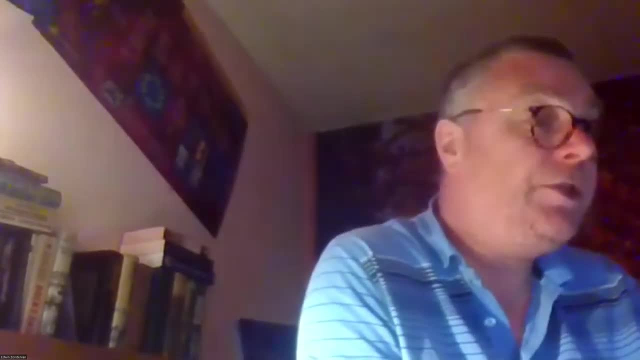 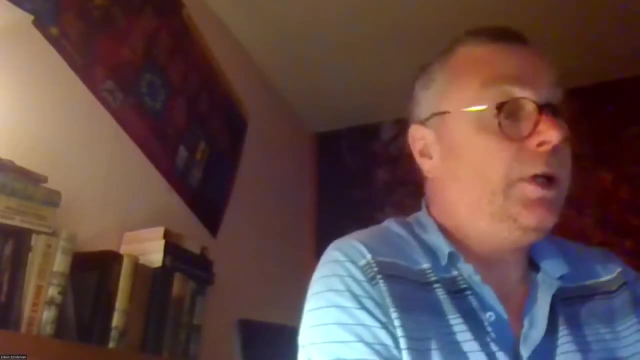 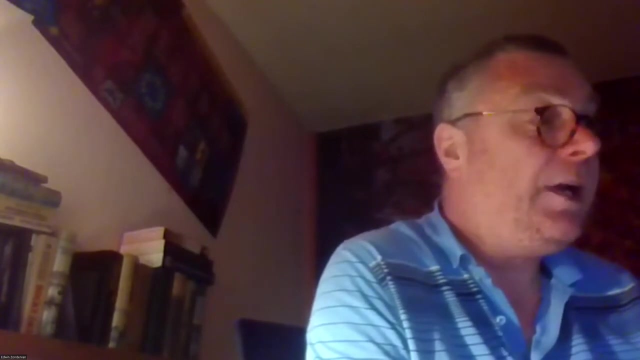 Especially in distillation columns, How to estimate physical properties, Thermodynamics, And then a discussion followed from Daniel's side on Yeah, isotropic and zeotropic separation, sequencing, How to use a residue curve, maps And ternary diagrams to identify regions of suitable distillation processes. 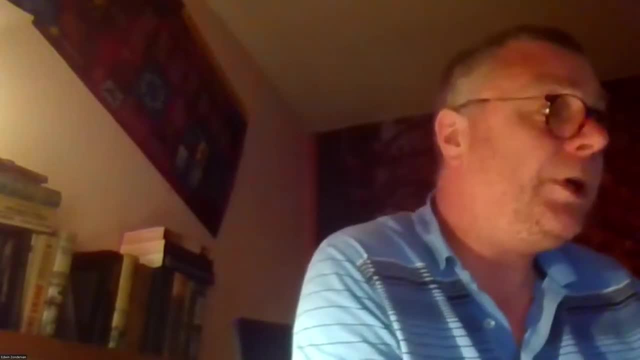 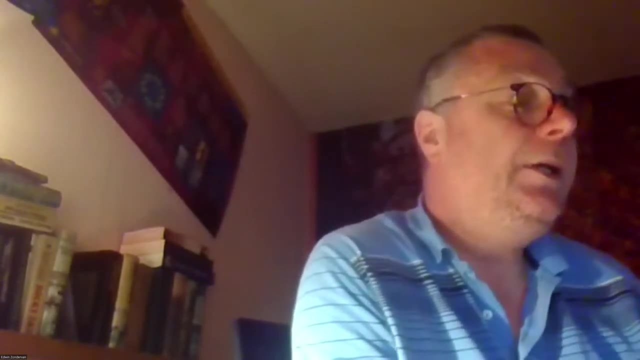 Last item tackled in this second topic Was the second law analysis, Where material and energy streams are valued as a function of the work that is available. Here also a discussion was led by Sun Moon On especially the heuristics for new technologies. 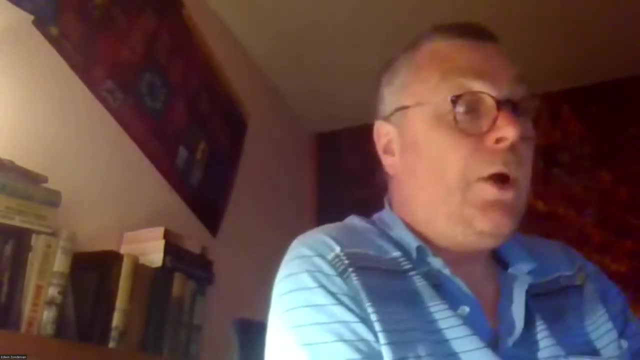 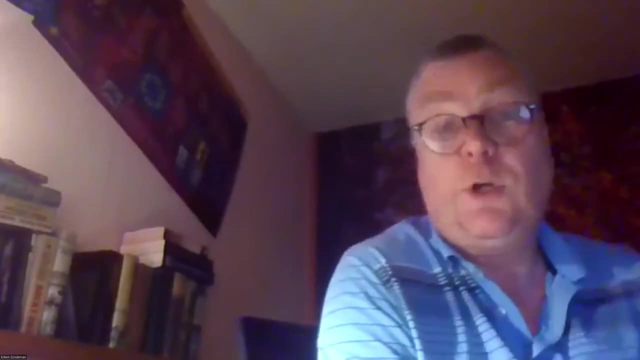 For example, electrolysis, And there was a question on how Using benchmark processes available from patterns already, So how to use something existing to come up with new designs For here. I took as a key message or a takeaway is that Other disciplines 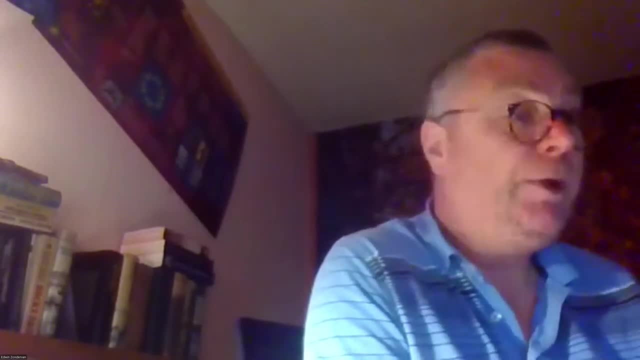 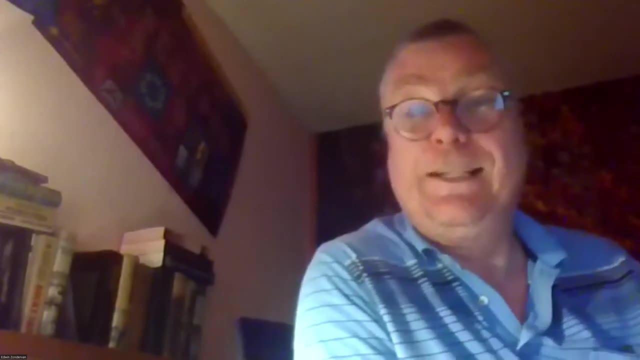 Such as nanotechnology, might come in very handy When understanding and designing new processes, For example, vaccine manufacturing. And then the last topic, that was really accelerated Because we ran out of time. I think we're running out of time also now. 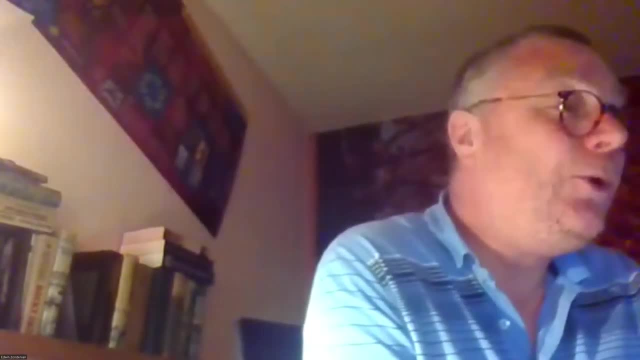 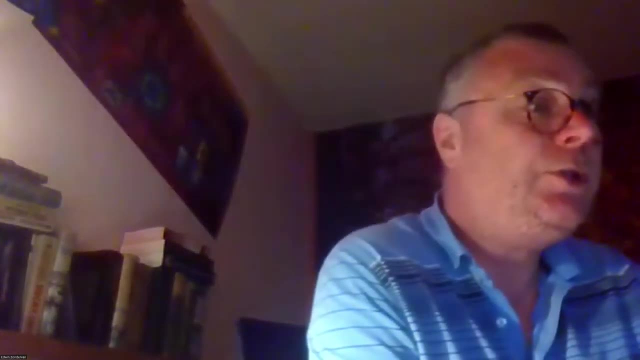 So I will speed up. It's a short outline on how to design efficient heat exchange networks, Doing heat integration by mapping source and sink temperatures, The basic idea of the temperature interval method, Pinch analysis and threshold columns. Then there was a very brief 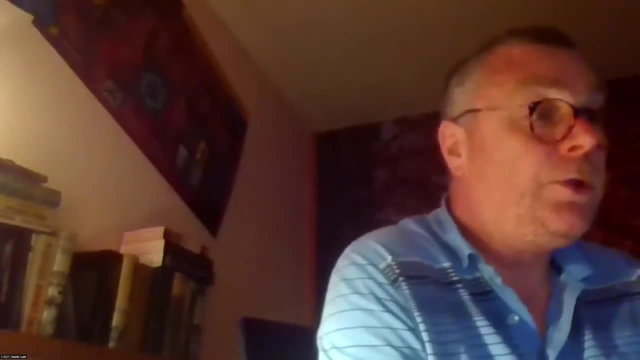 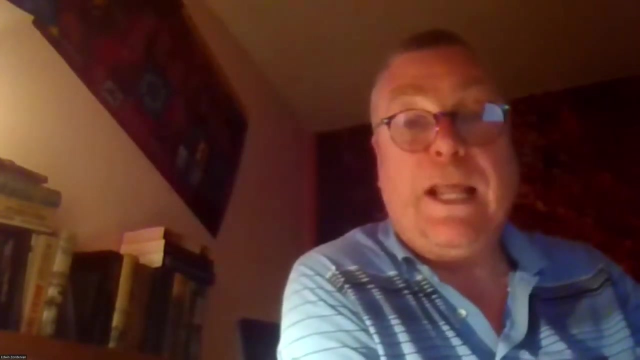 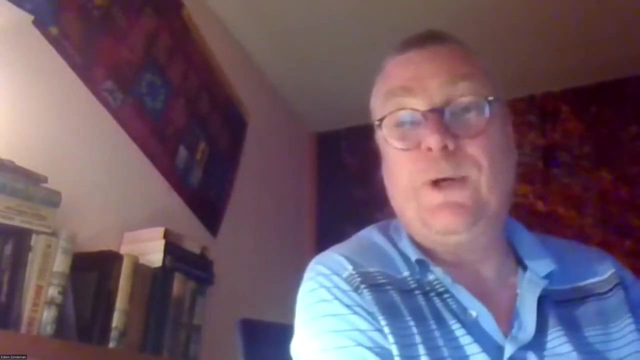 Announcement on How to do the economics: Capital cost estimation, Profitability analysis, The time value of money- And then, in two slides, The aspect of plant wide control, Which I think is a cornerstone, Because we are dealing more and more with safe variability in feedstock. 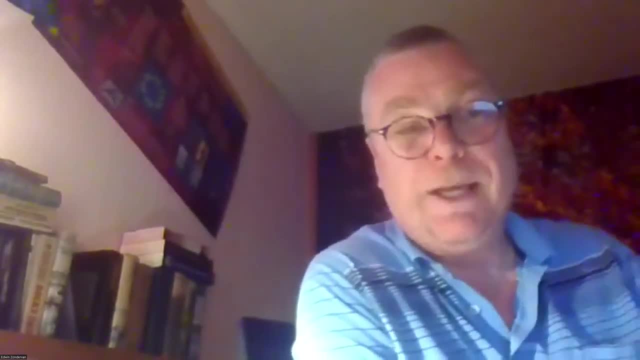 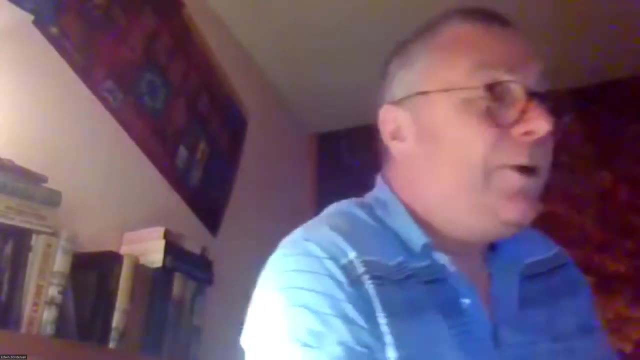 Biomass, But also think renewable energy Control. maybe, Maybe we should flip. If you talk about flip teaching, Start next time with plant wide control. So for the economics, I took a takeaway: It will take more than pressing a button. 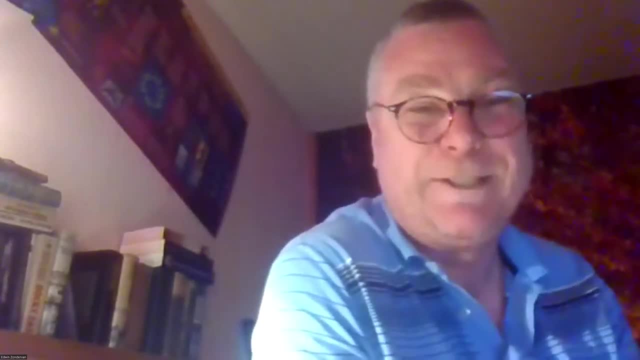 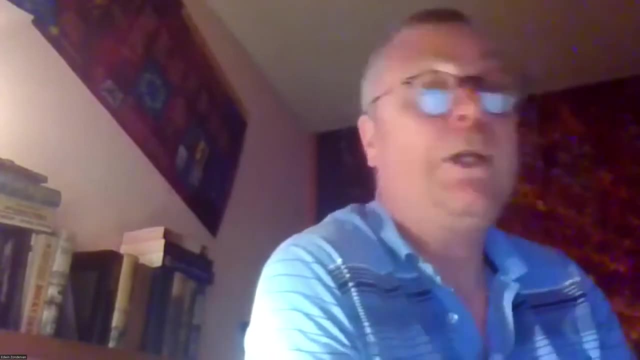 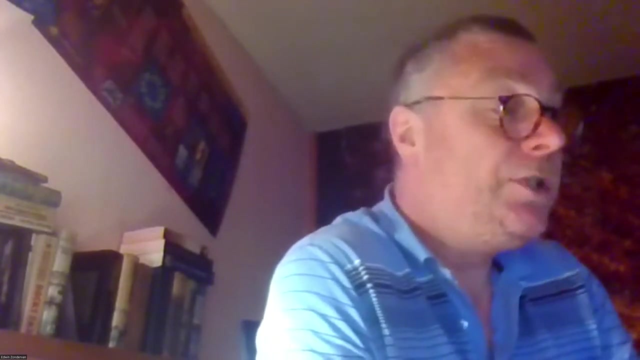 To get accurate economic estimates For your design. So my personal closing remark here is that we just witnessed a very Complete but also very classical way of conceptual process design, Focused on traditional chemical industry And besides all concepts and tools that we have at hand right now. 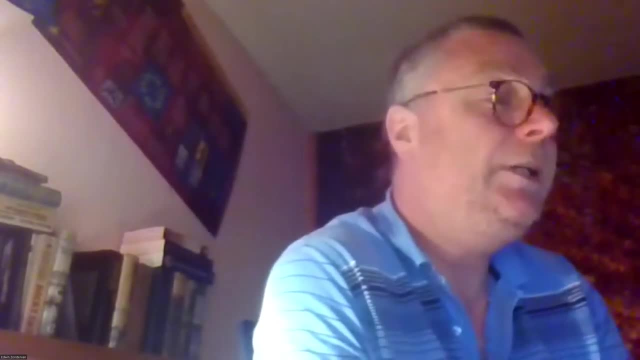 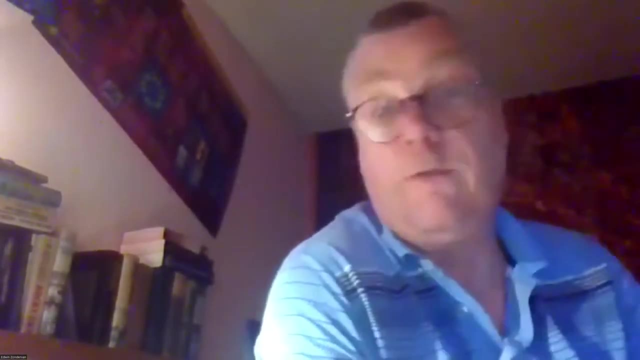 We might still wonder what new, different requirements are needed When we think of new feedstock And products. More complex- Think of biomass, food Or volatile availability of the energy- How the decision making changes when the processes should be fully circular Maybe not so much touched. 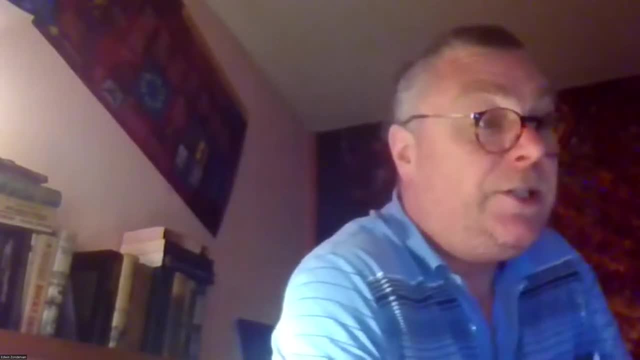 And is the product design Paradigm also The product designer? Product design paradigm: Is that the task for the chemical engineer Or for, maybe, business developers? I don't know. And then the last one: What are the consequences of a crisis? 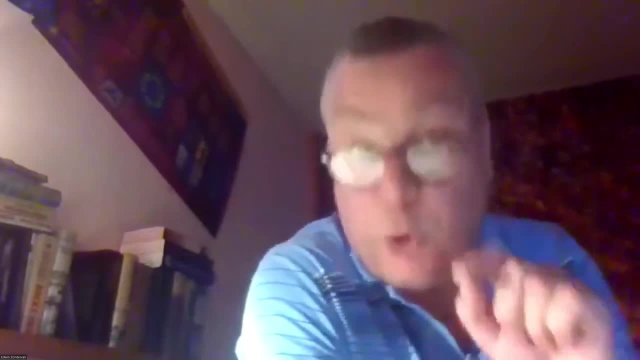 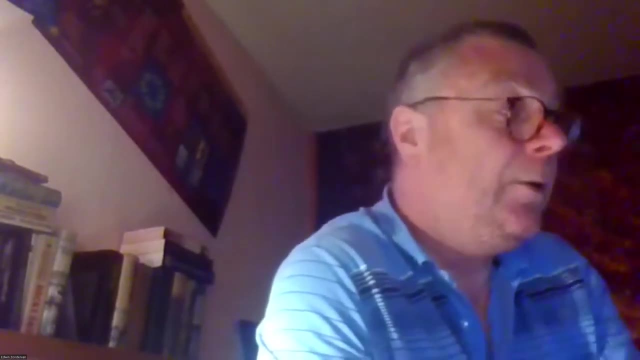 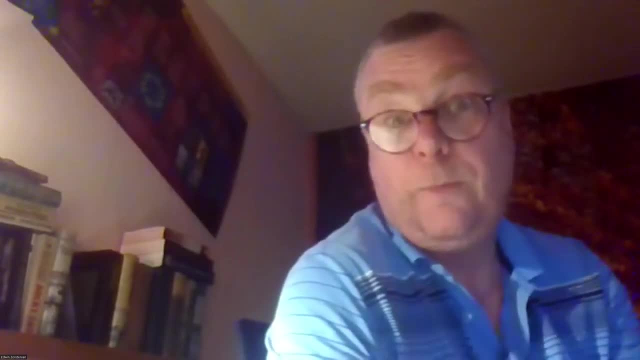 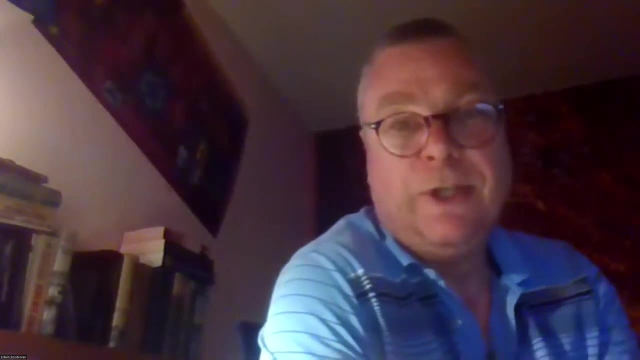 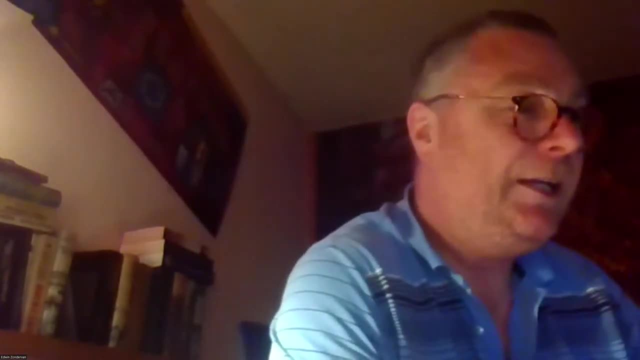 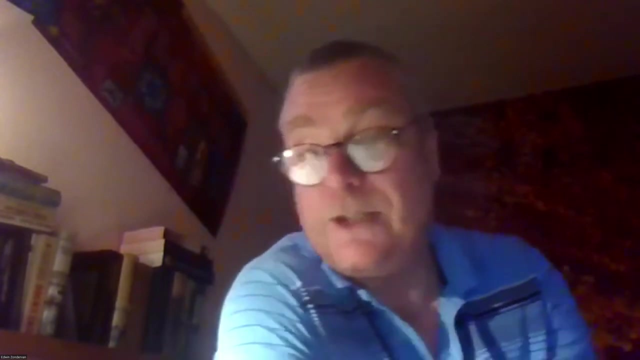 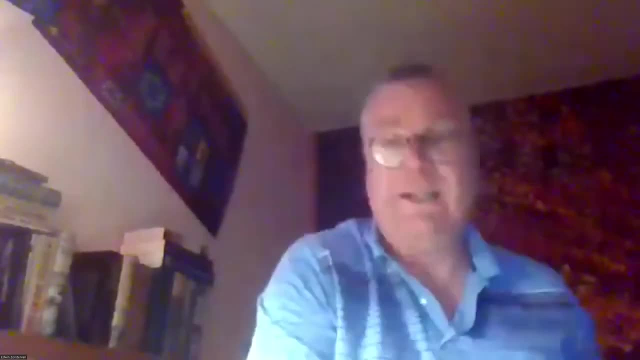 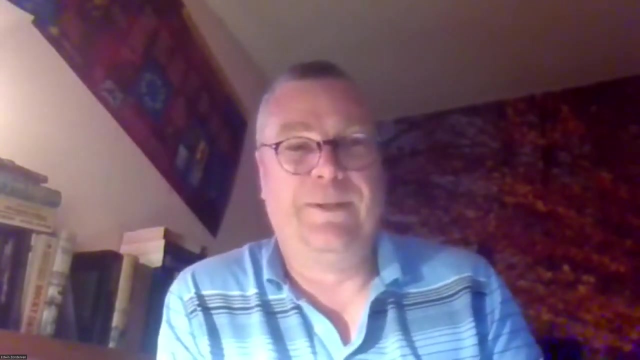 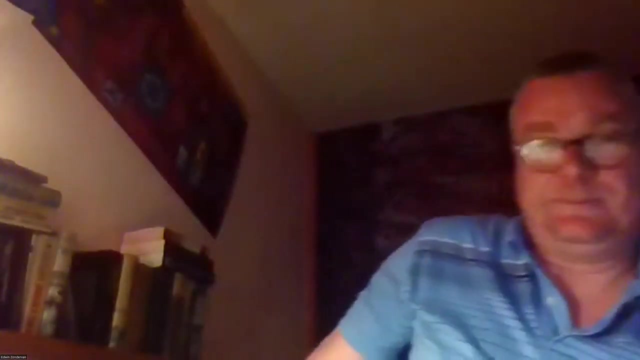 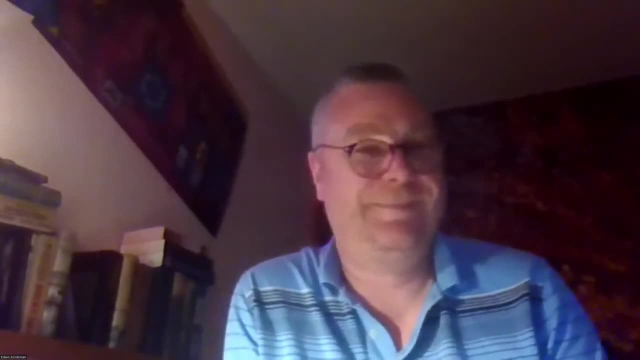 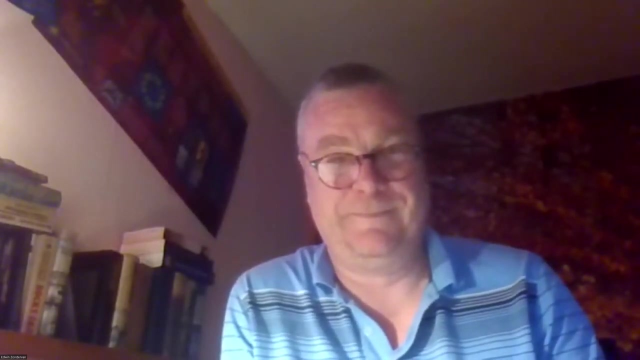 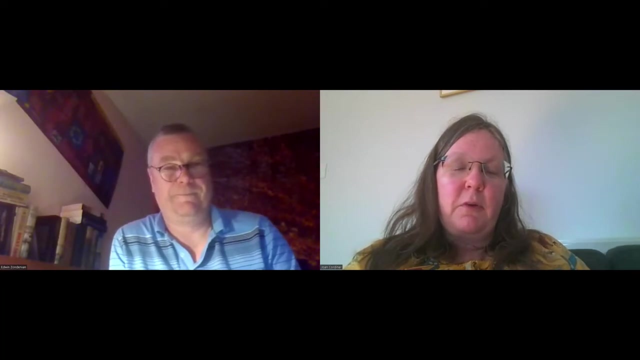 please go ahead. hi there, can you hear me okay? yes, all right. so i i'm an academic now, but i was for a long time an industrialist and i helped at various universities around the world with design projects, and as did my teams laterally in my career, and quite quite a few universities gave. 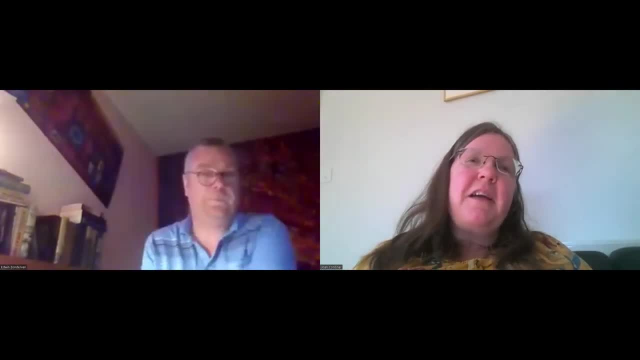 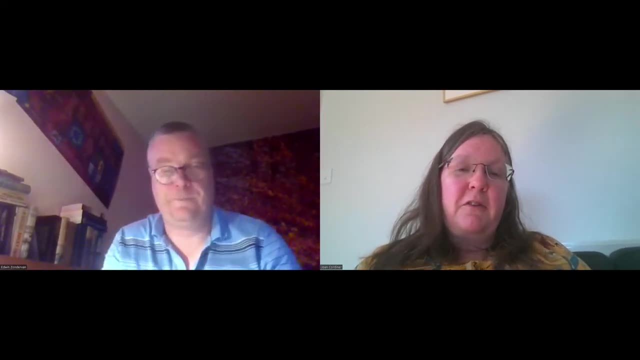 a little handbook or, you know, some guidance for the industrialists, and i find that really helpful because when you're coming in from outside, you can read the course notes. you can, you know, read the synopsis of what's been covered, but it's really helpful to have some guidance about. 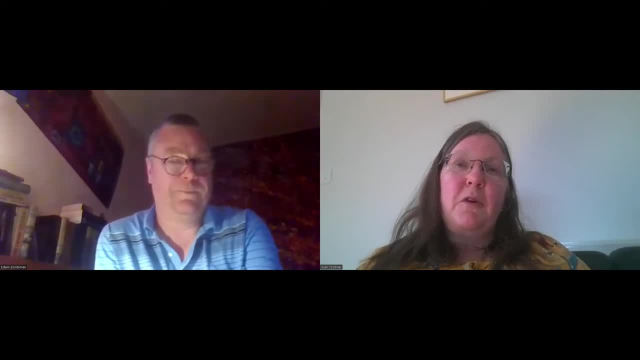 if you're going to use an industrialist, what you want them to do and what you don't want them to do- and i think that what you don't want is equally important- and make sure they understand the rubric. i think the first time i saw a really good rubric was mario eden's design project way. 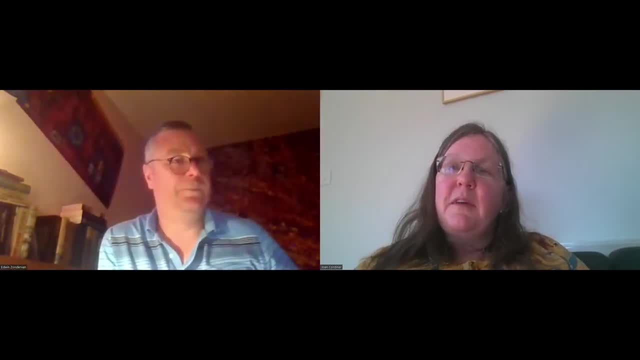 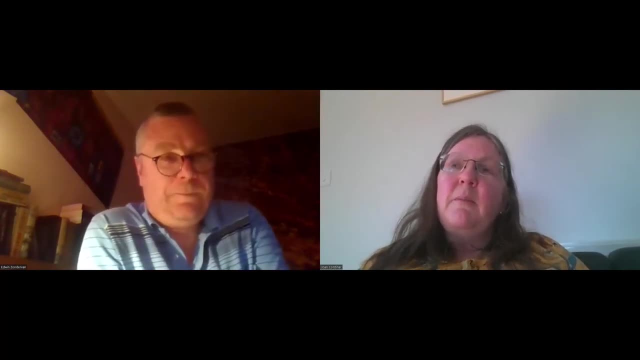 back in 1990, so, um, i don't think i'd seen one before that. but but that really helps the industrialist as well. so, um nc state, where my daughter went, they had 35 design projects to choose from and the students got to vote for um five in order of preference, and they 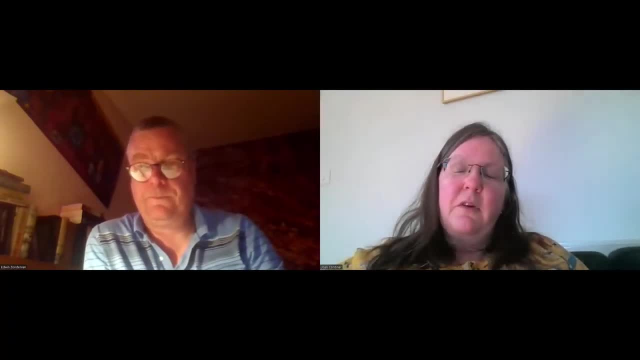 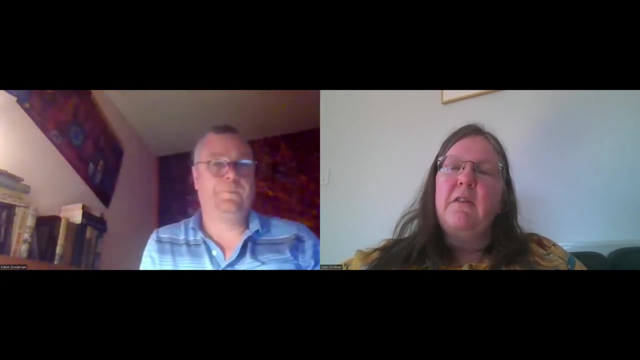 um, they then got allocated- and i don't think they filled all 35 and i don't know how many they did- and they had regular meetings with the, the external staff, and i think that they were even more enthusiastic and the students started to get involved with the students and that's how they got their hands on this project. 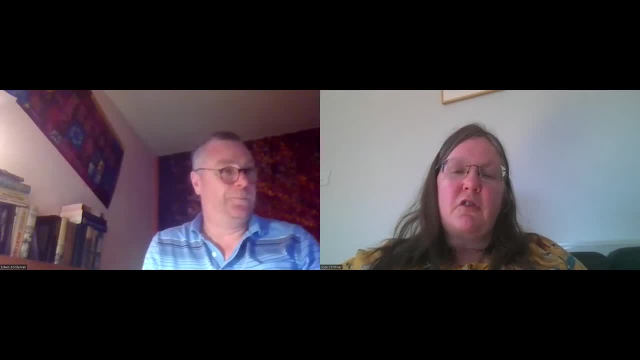 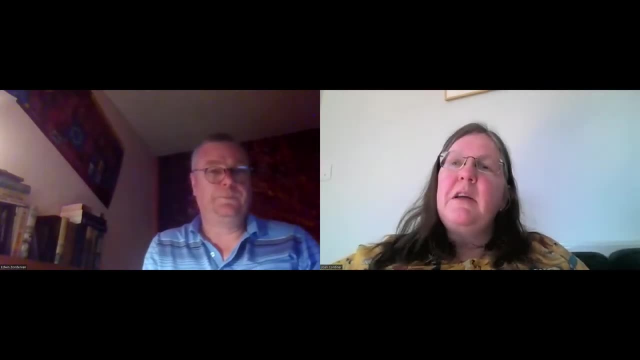 so, yeah, i wouldn't say it was a no-brainer for me, just because i watched the video and i didn't have a big deal with it. i don't think anybody did- because it was so much fun, and so i'm just going to say that i i think that that was the first thing i saw. 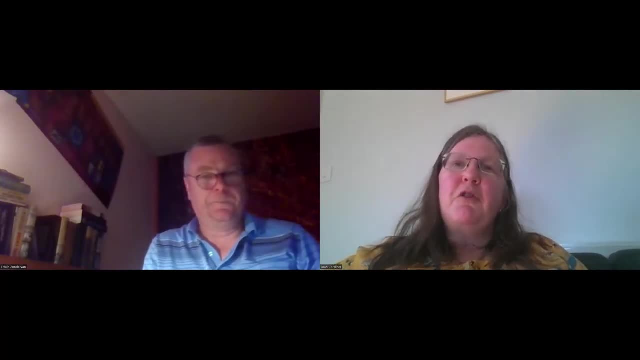 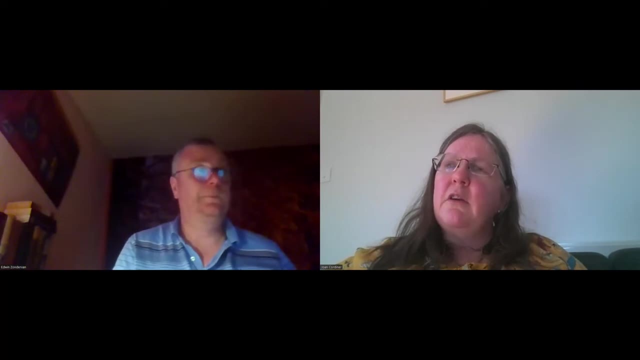 in the second week of- and i think i don't know if any of you saw it, but it was the first thing i really saw that was a little bit different from what i'd seen- spoke to Lisa Bullard, who leads the course there, and she has a book as well about teaching. 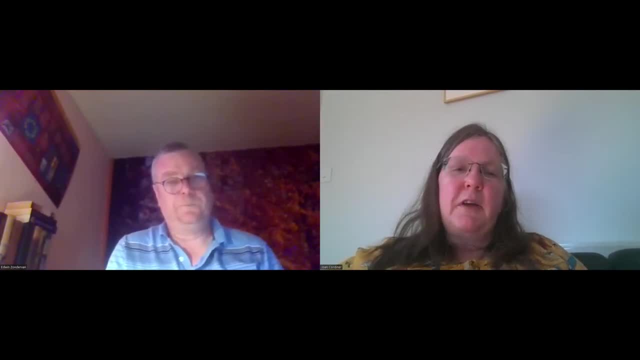 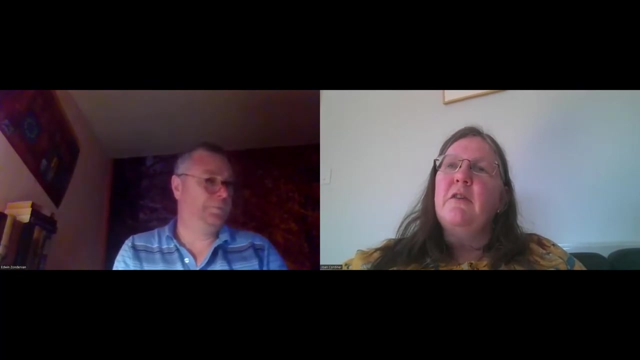 STEM that advocates the flipped classroom, but are we marking the design process, the thought or the outputs and if actually, what you get them to elucidate in their sections of the report, the process they've used and the thinking they've used? it's easier to mark. 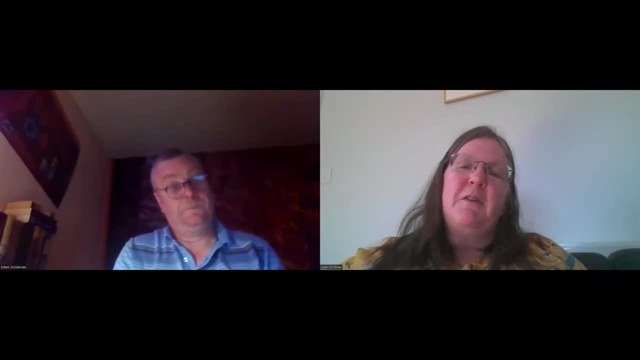 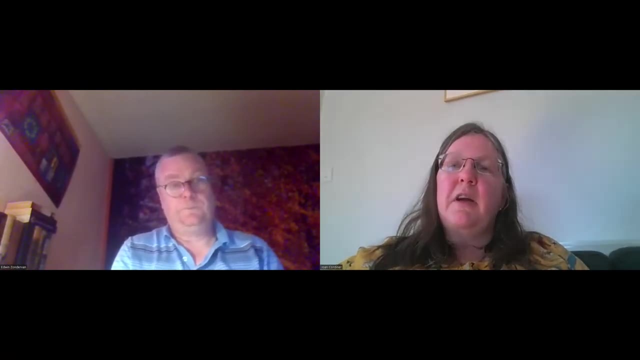 because the outputs in a sense don't matter. I mean they do, but it's really. have they actually learned the material? so I thought that was an interesting way of marking. but you know, overall, if you're going to use industrial lists, you need to teach them too, and I think 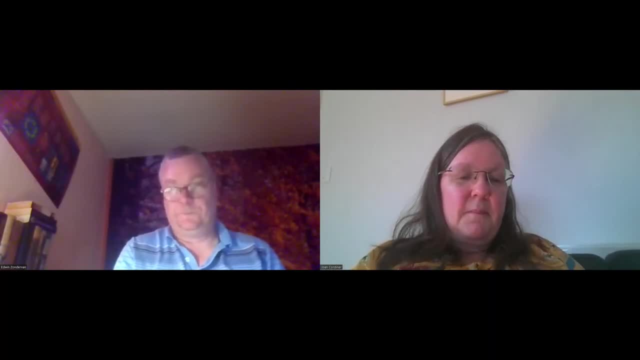 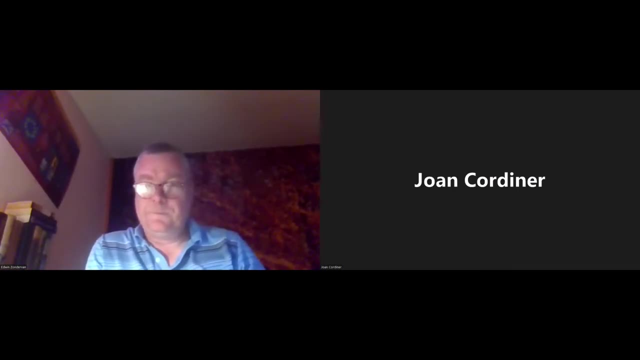 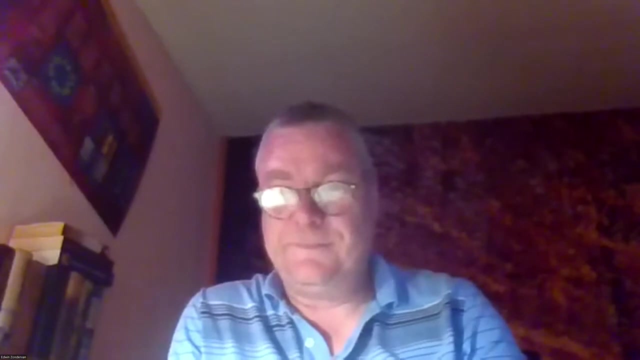 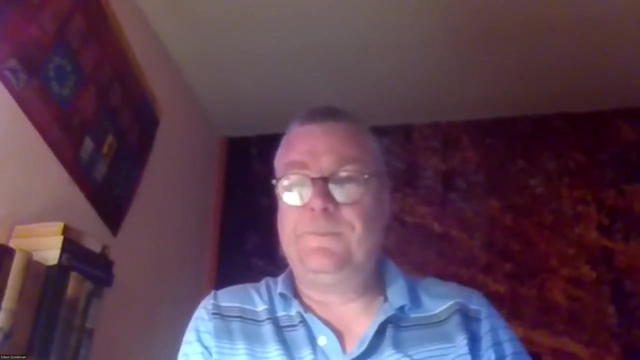 that helps. Okay, Yeah, Before you answer, maybe there is a question that I'm sure Warren would like very much. It's from Jaime David. If you want to ask your question, please unmute him. You can ask it Jaime David. 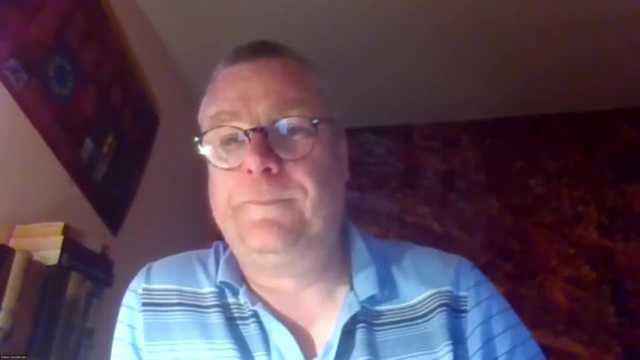 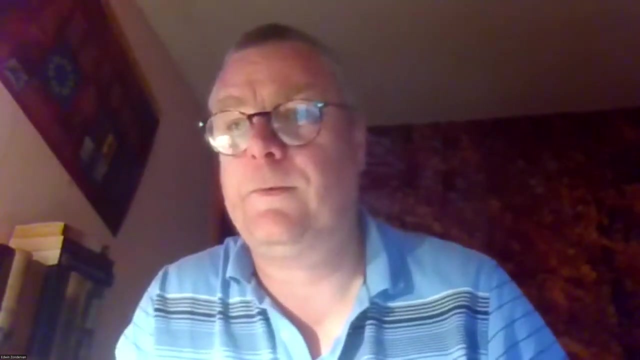 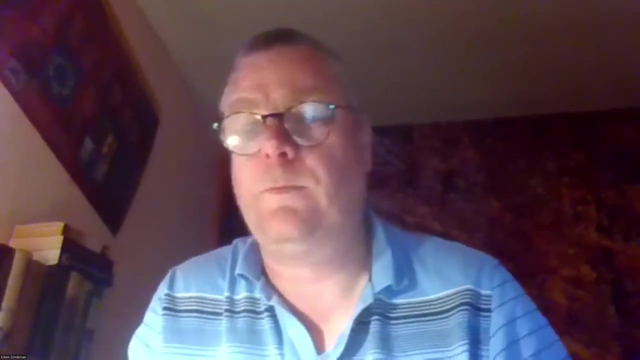 Okay, Hi, Hi, Hi. Can you find the team J A, I M E, David Ponce? Okay, I don't, I think. Let me read it. read the question: When you use the second law analysis, what type of exergy is most relevant? physical? 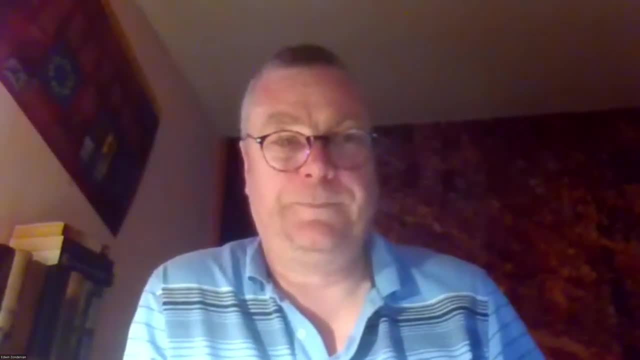 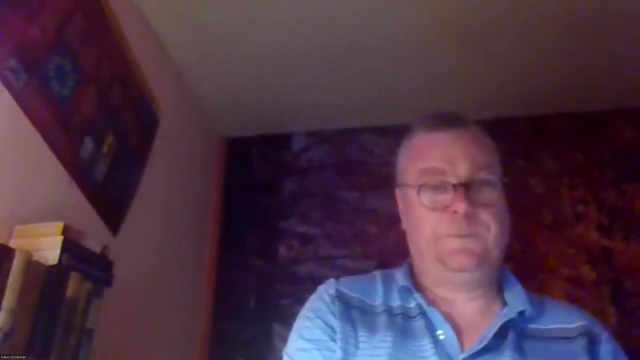 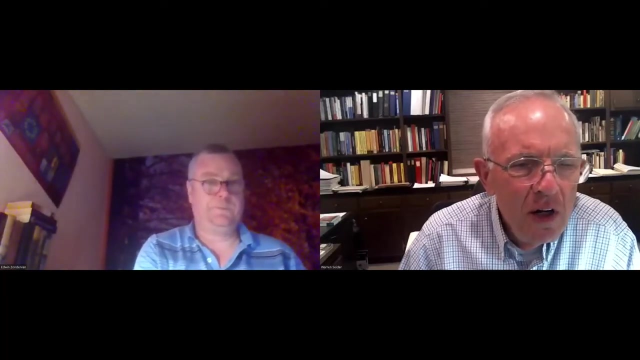 or chemical For Warren. Okay, Thank you. Well, I'm not familiar with working with the chemical. We've worked with the physical all along. Professor Bob Seder, JD Seder, S-E-A-D-E-R, wrote Chapter 10.. 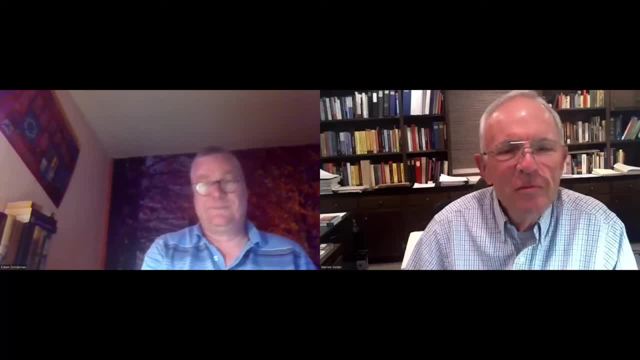 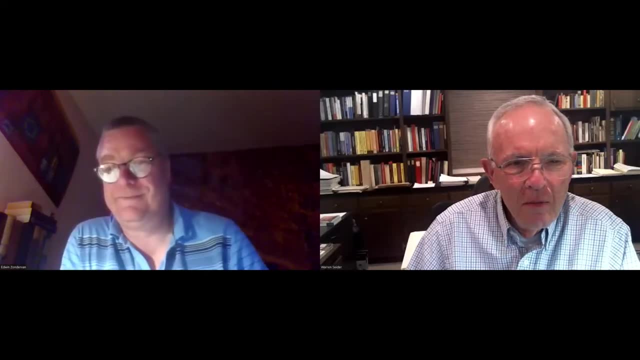 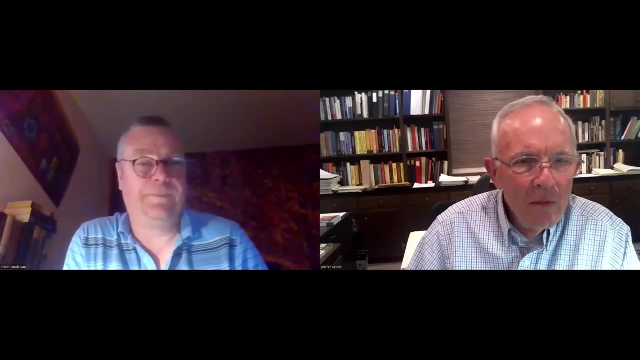 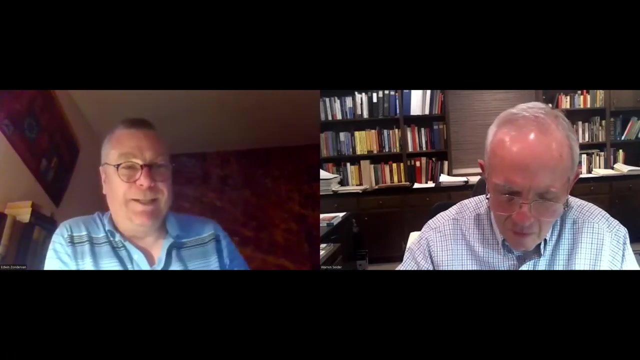 That would be a good question for him, Okay. Okay then I would just ask Danny Edwin, whatever the others have said, do you have anything to say From my side? no, I think it has also been a long and an intensive event. 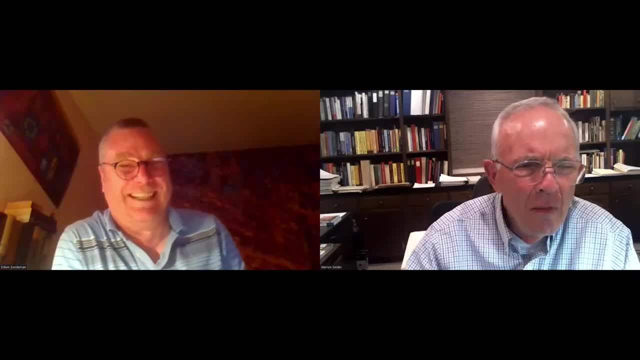 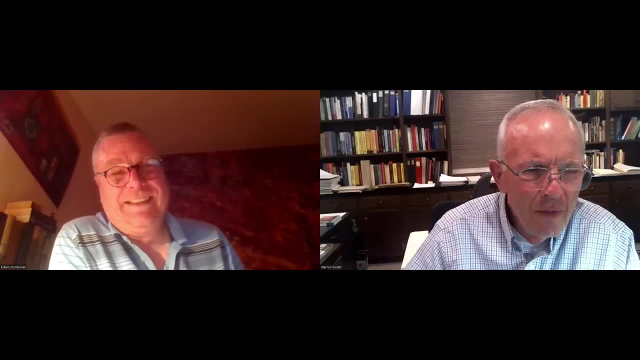 so we're maybe also getting towards the saturation. Yes, From my part. the Jones issues are really super important if the industrial, The industrial contribution, isn't just going to be to grade the projects at the end but to be involved with the project throughout the entire semester. 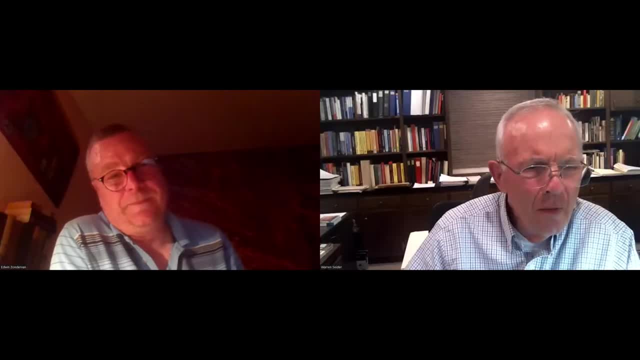 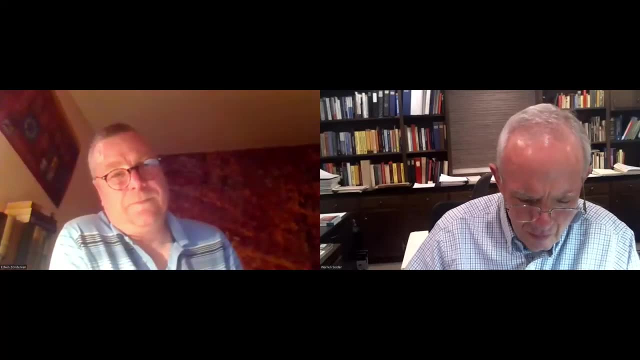 which I don't do at the Technion. Regarding the grading at the end, I have a very simple grading sheet that involves quite straight and very transparent rubrics that they just have to give their viewpoints for various aspects of the presentation that the students make at the end. 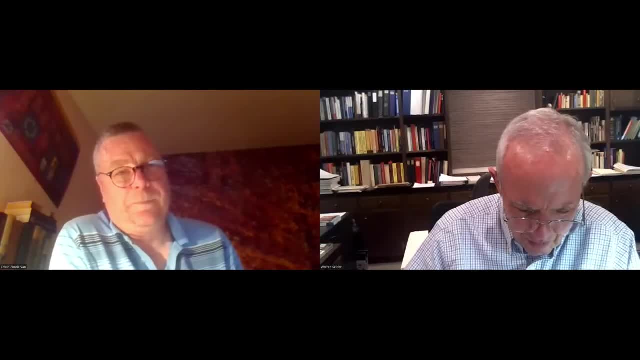 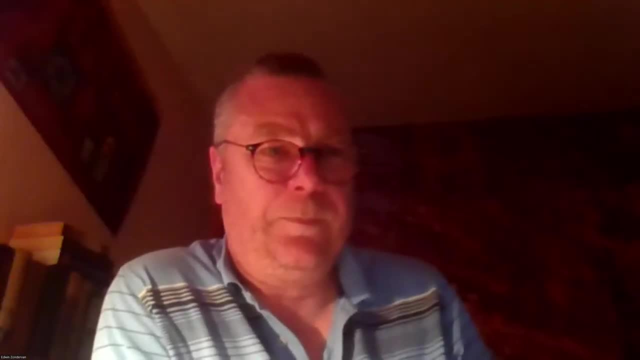 That's worked quite well. Well, actually it's a variation of of a form that is available in our book also, So basically I'm using that and that for many years- I mean 10 plus years- has been fine. 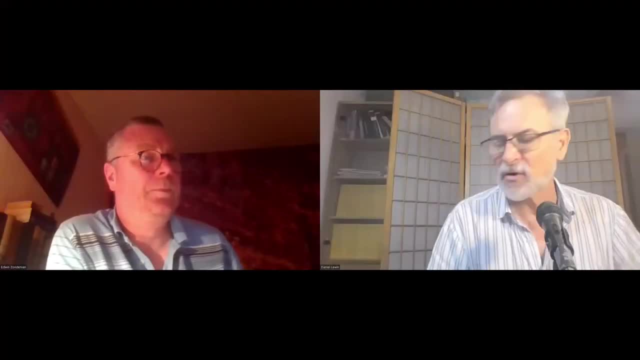 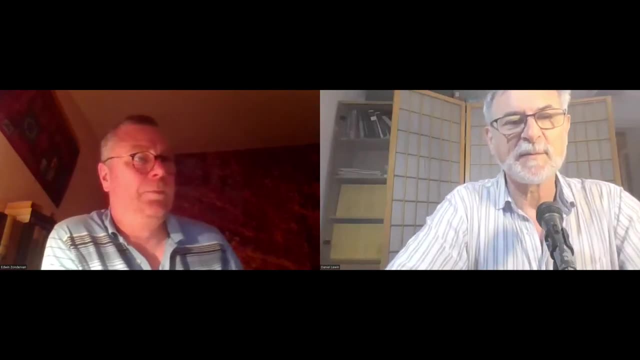 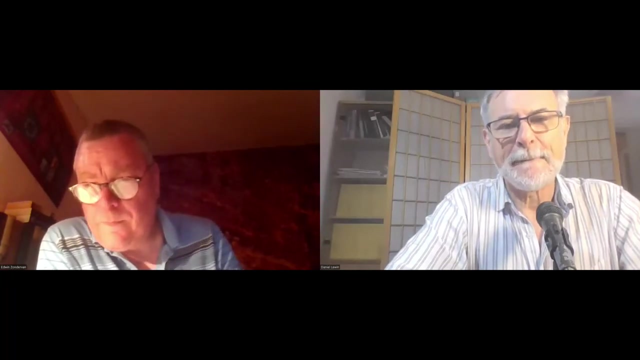 I really liked the input that we got from Mario. I'm going to look into this CATME program. This might actually be a big help to solve a real problem. It's worked well for us. Yeah, I can. There is a question on: could you please identify the scope? 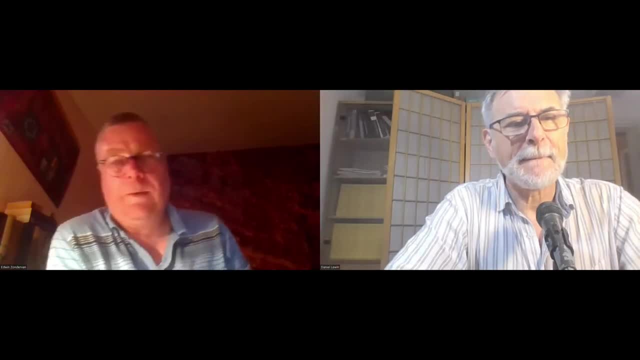 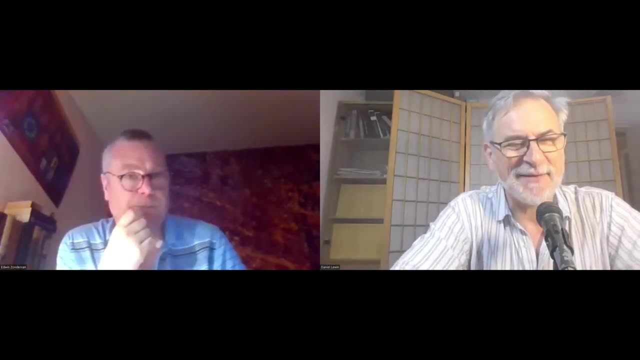 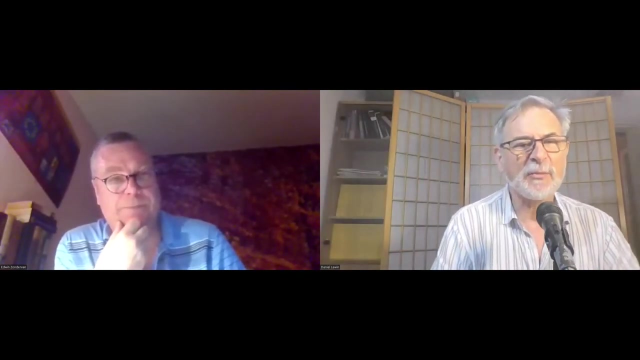 of the project assigned to the student group, The one that I give every year is basically a failed project. I mean, it's a feasible project but it's losing money unacceptably, because I basically have solved the problem given to the students using all the mistakes I have ever seen. 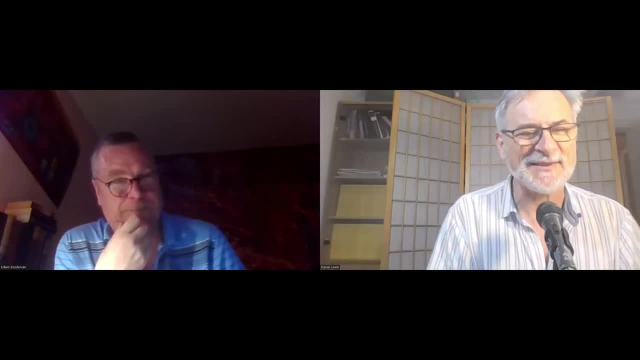 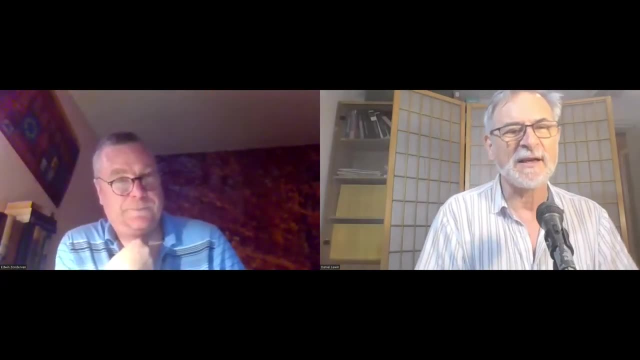 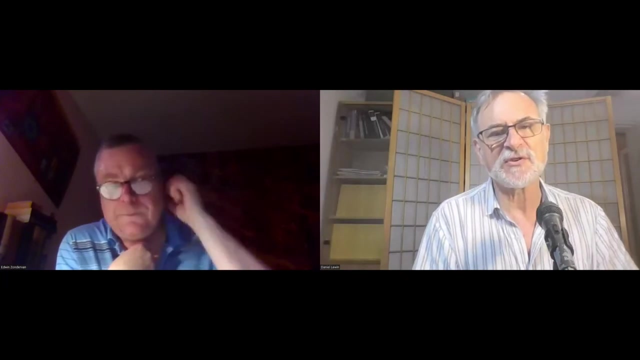 over 16 years of experience with other projects. So it's a collection of calamities that lead to failed project basically, And it requires a student to basically redesign the whole thing. Now Warren mentioned the usage of the spreadsheet that does the calculation of the economics. or let's say, 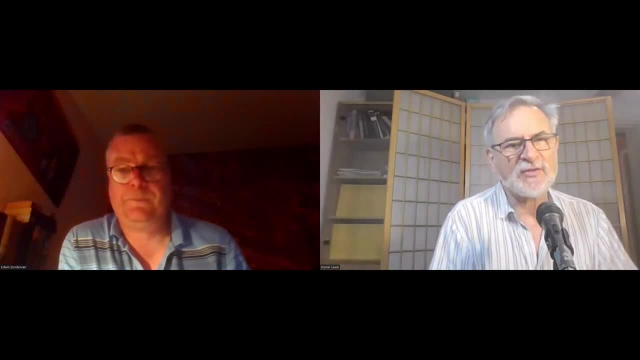 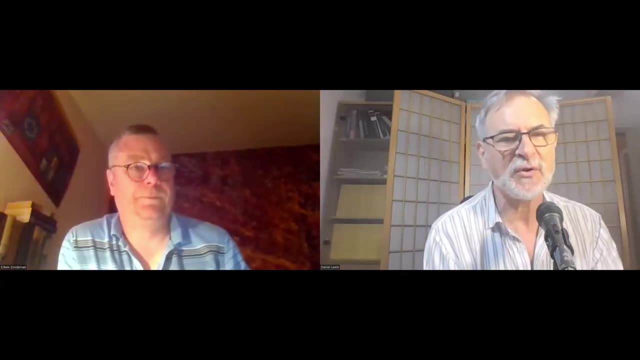 what's available with Aspen? We don't use Aspen. What we have done is we take all the equations that are in the book, all the costing equations, and introduce them into spreadsheets within Unisim, which means that students can do their costing on the fly. 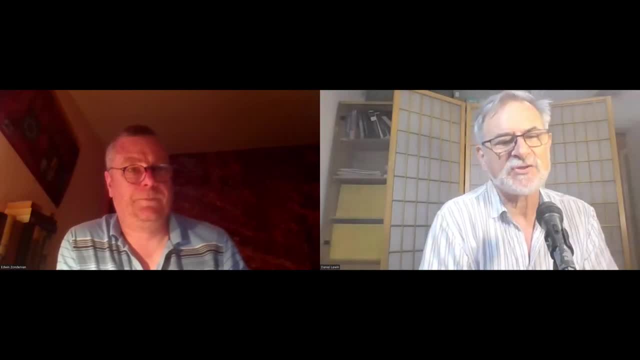 They make a change in engineering and if they adjust the spreadsheets accordingly, that immediately adjusts the economic measures of the process. So students get an instant response to any change they make to the process, how it affects the economics, which is very helpful. 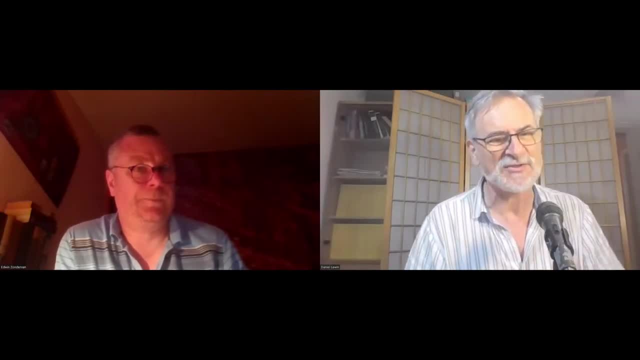 because they know how to drive, in which direction they need to drive the engineering. This is very and it's a very good thing for them to be having in front of them always before they make any change. If there are any students in the participants now. 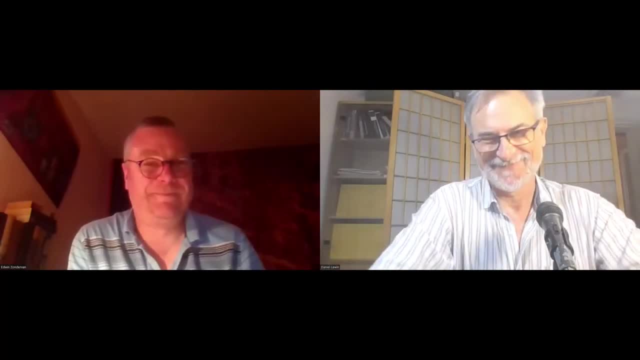 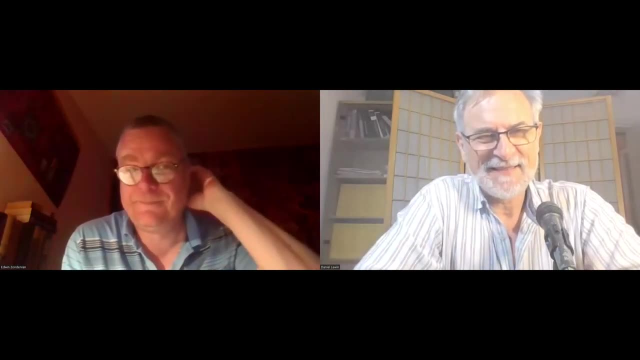 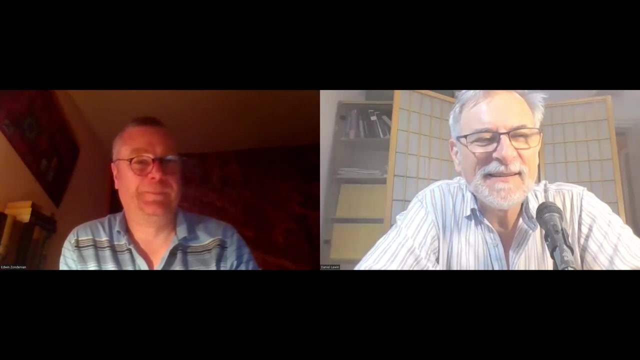 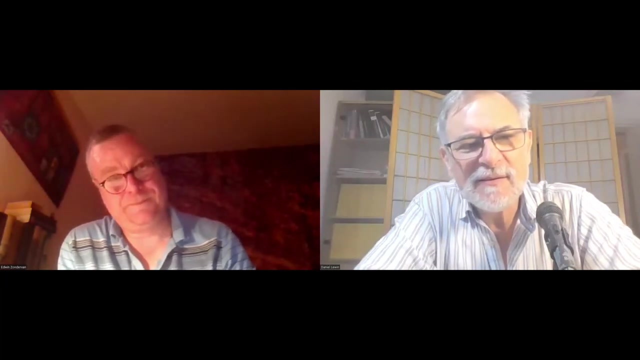 you have the last chance to ask some questions And in the meanwhile, you're thinking of questions. There are two questions that Danny would like, because I stopped him from talking about control. One question says: when teaching plant-wide control, may you share some experience with dynamic simulation software? 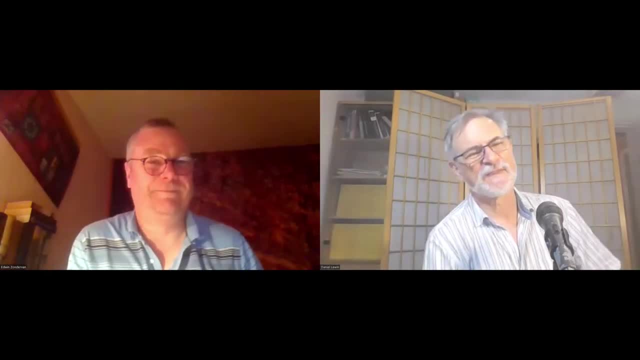 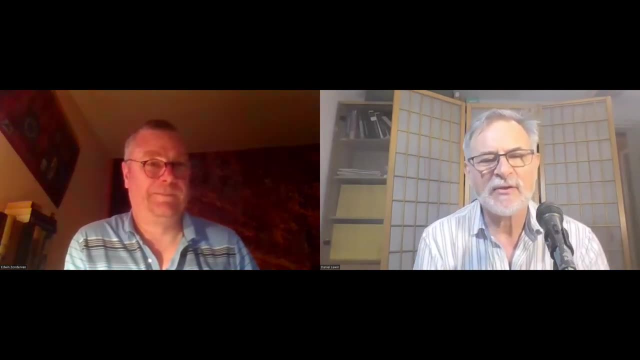 And a second question related is what software you propose for your students to use for design control systems. The scope is: it's beyond scope for a capstone design course to expect students to handle dynamic simulation as well. We do not teach dynamic simulation. 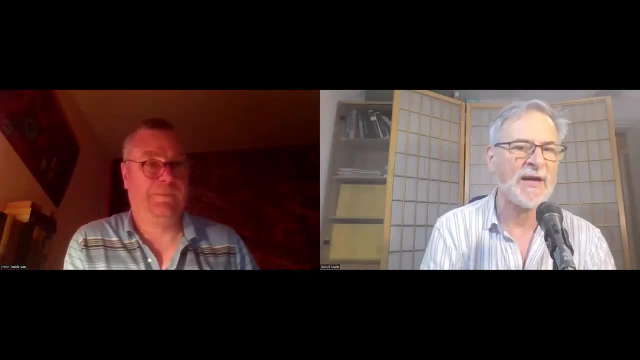 Unisim does have that capability And for advanced projects I've had students working on dynamics And it's very exciting what you can do. The average student won't be able to do this, So we don't require it. It would be a very nice thing to have, but I think it's going. 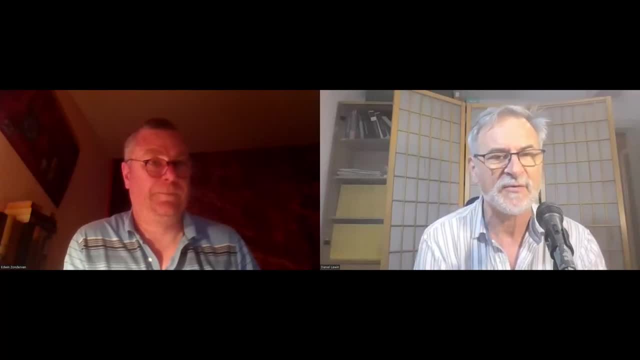 to overstretch what we're offering. We're asking for the average student for such a project. Probably a better solution would be to use Asim, because I think their dynamic simulator is much easier to use than the Unisim. one is probably more reliable too. 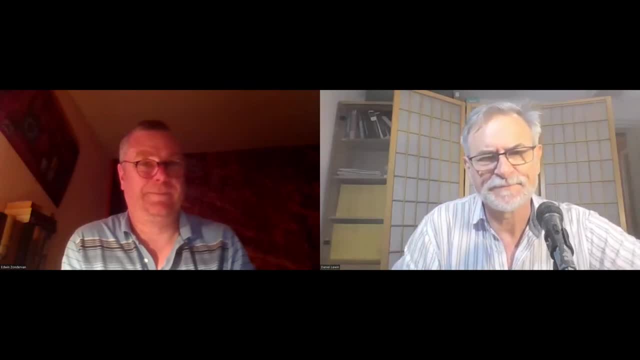 I know that Leuven uses it all the time. I was going to say that Bill Leuven has written books on the subject of Yeah, yeah, yeah, No. it's definitely doable, but I'm just saying from the point. 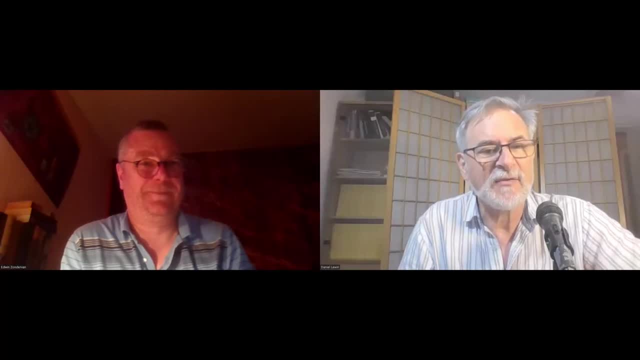 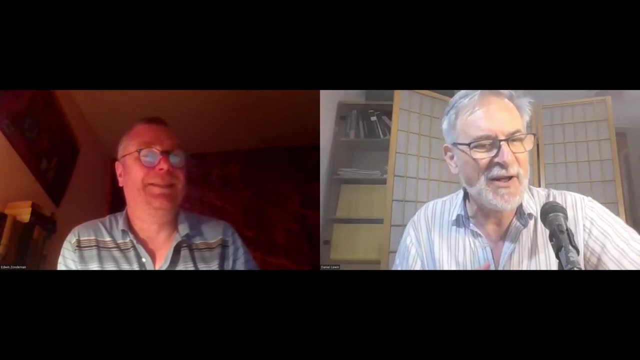 of view of how loaded the course already is. to add that to everything else, I think would be just too much. That I don't argue about the usefulness of it, Don't get me wrong. I think it would be very nice to have that in, but there's a limit to what you can offer. 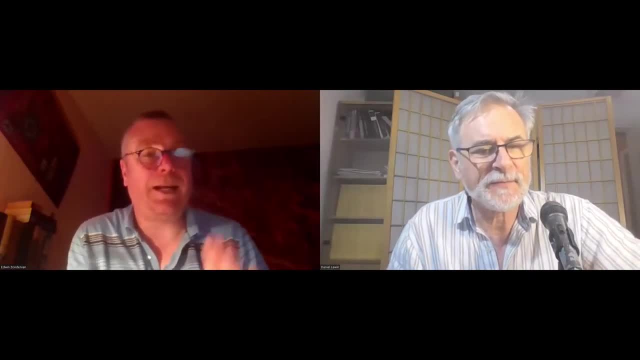 Often it's said that I mean control and design are kind of different subjects. No, they're not. No, they should be. but practically you're not using dynamics in your course, You're just benching it, So it's kind of like put under the umbrella of a process control course. 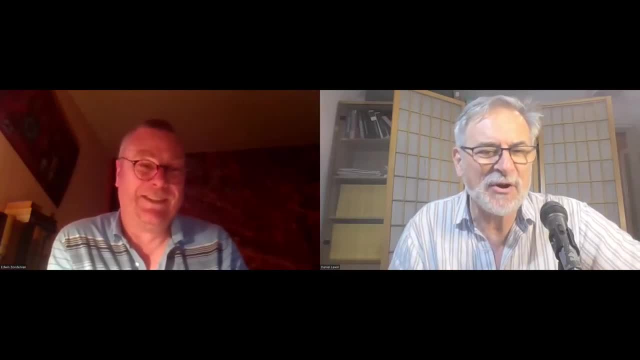 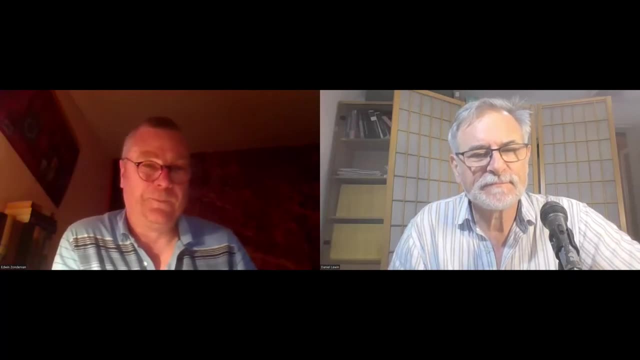 Yeah, because I have. yeah, sure, But how much time are you going to need to do this properly? That's the problem. yeah, Okay, I don't see any questions from any students, but before we stop, let us thank the Thai team, the Thai team members. 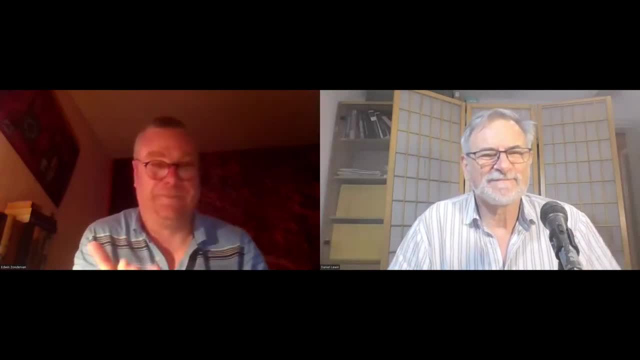 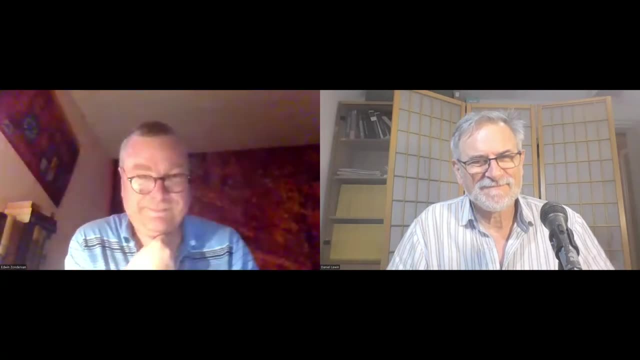 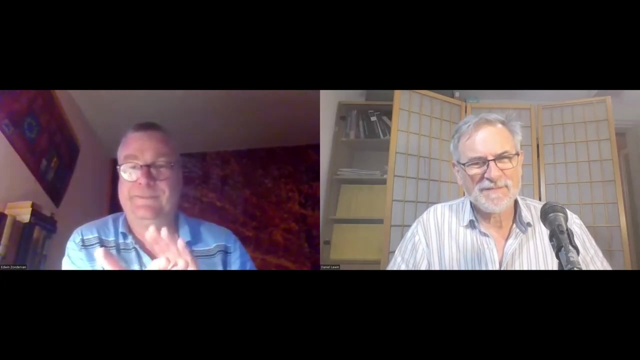 Thank you for organizing it very well. I will just say their first names: Ora Koch, Nishakon, Jakrapath, Raksina Siddhida. I hope I've mentioned all of you. Thank you very much for organizing it. 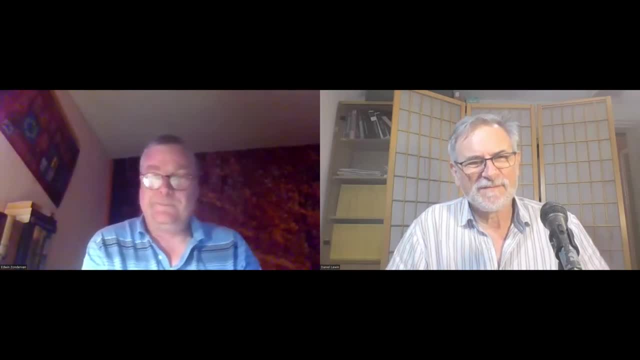 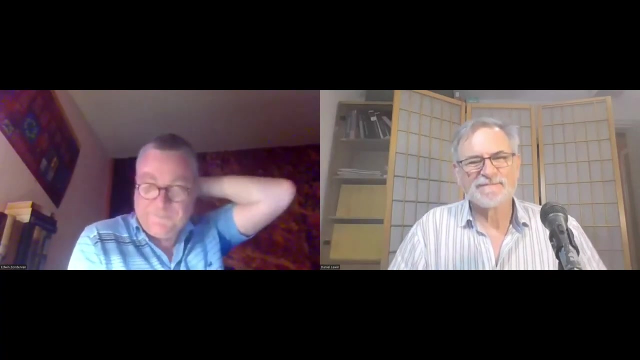 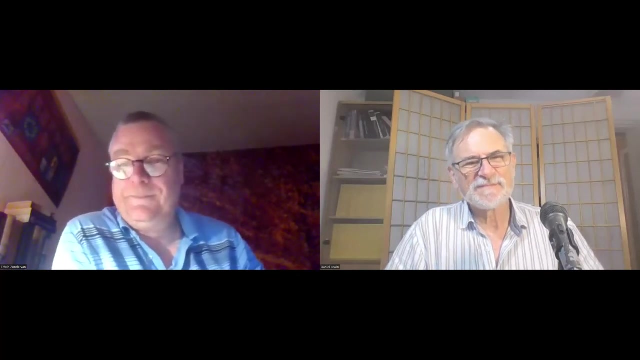 And let me also. We are also receiving some compliments. So one person has said: thank you for wonderful and informative presentation, Excellent experience attending the webinar, Fantastic. And I will read one more, which is near the end: So thank you very much for excellent work. 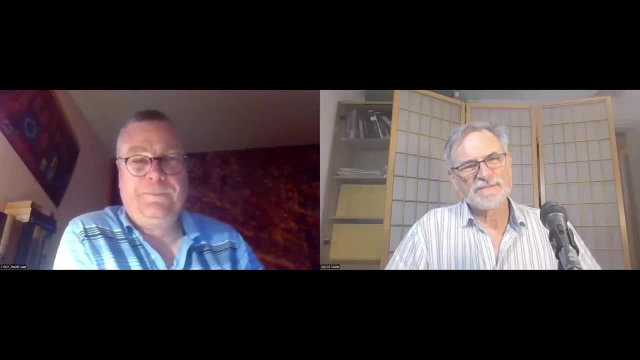 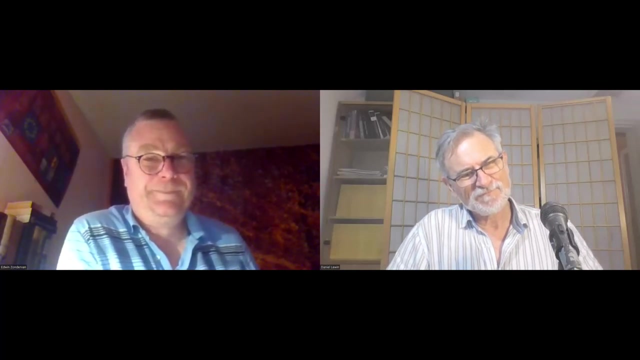 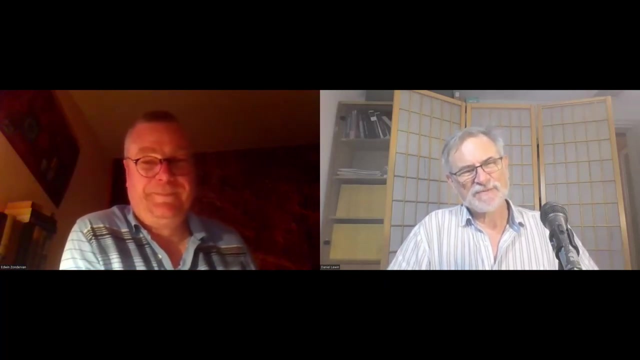 And a more detailed one. Where is it? Thanks a lot for the lectures and organization of this webinar. I very much enjoyed it and learned a lot. This will help us to improve our process, design course as well, and so on. Thank you very much for a great webinar. 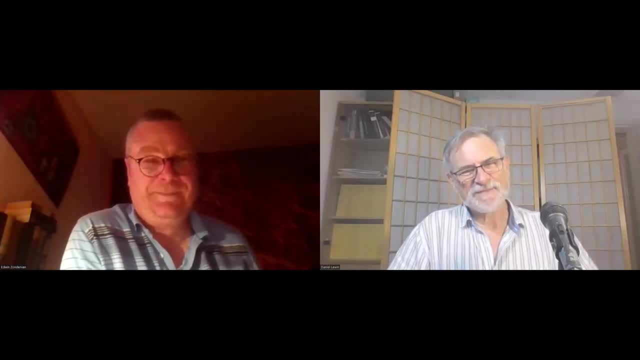 These are all faculty members Right, And it was an excellent webinar, Thank you. Thank you very much. I think we'll end this webinar. Our last remark for me that remains is how do we couple the material and practices that is simulation-based with hands-on pilot plan? 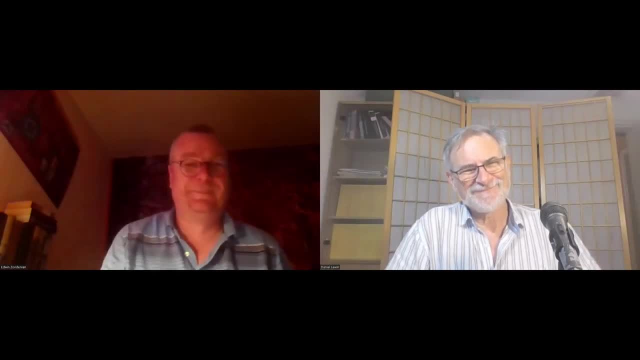 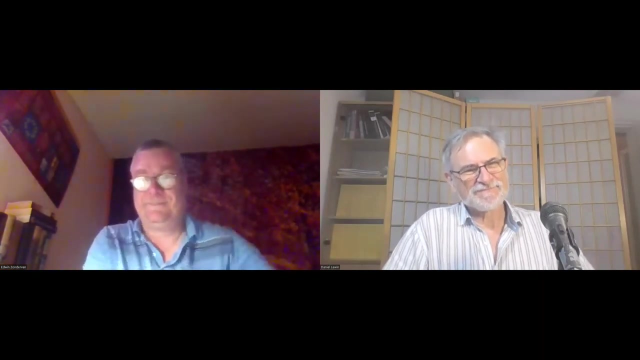 But that's a question. Let's forget that. Thank you very much for enriching seminar and so on. So thank you all for your participation, To Danny and Warren for preparing all the lectures and giving the lectures. my apology for stopping you a little bit at the end. 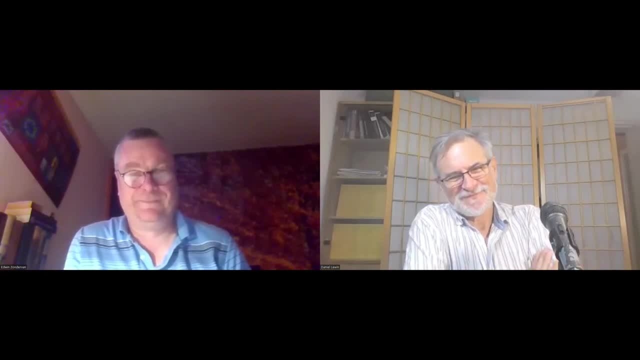 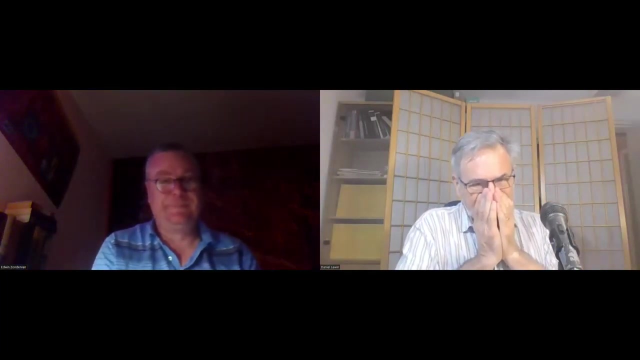 Thank you for Edwin, Iqbal, Mario and Bamroong for doing the panel discussions. I think I hope all the participants who are still here- you got something good out of it. We will put the recorded video on our YouTube channel. 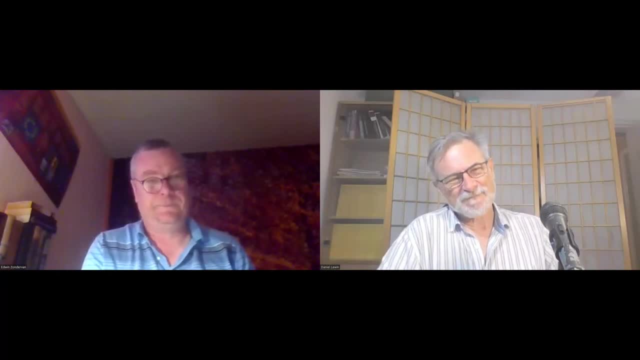 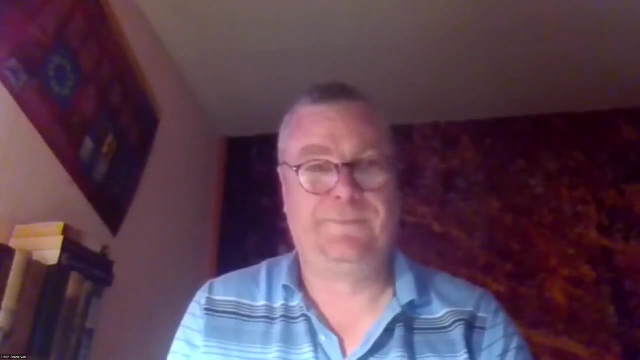 and we will also look at the questions and look at the discussions and maybe share them with you. Okay, I would like to add one thing. Okay, I was going to thank all the people that you did, but, more importantly, we all want to thank you. 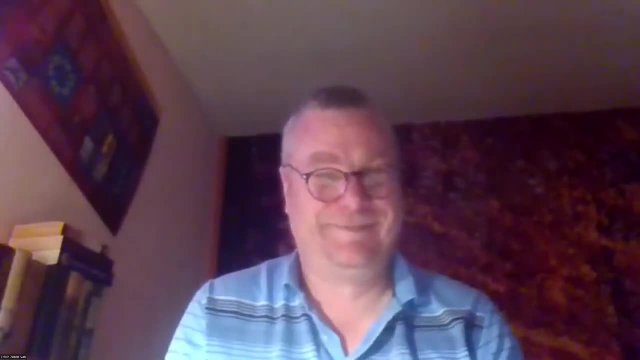 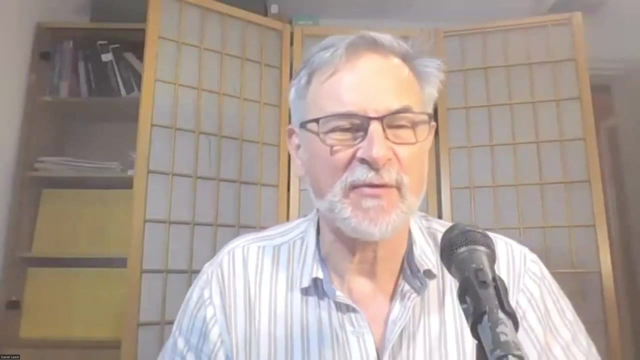 It was your concept to do this. You invited us to do it and it's very much appreciated, Rafi. Yes, thank you very much for inviting us, Rafi. Thank you very much. Thank you very much, Thank you.